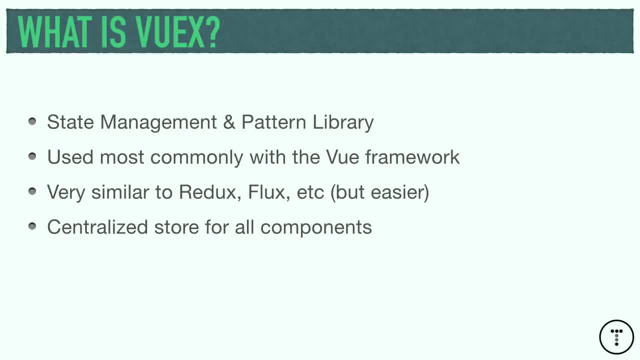 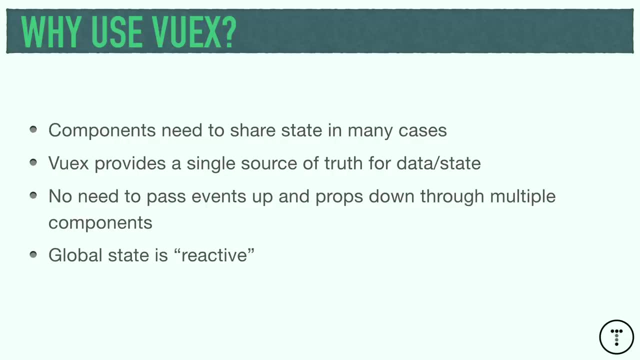 Redux a few times in this course. So Vuex works as a centralized store for all components, which probably means that you can use it for a lot of things. So I'm going to go ahead and talk a little bit more about Redux. So Vuex brings us to why would we use Vuex in our apps. Now, I'm not going to say that every single Vue.js app needs to use Vuex or state management, just like not all React apps need to use Redux. It's more for medium to large scale projects that have multiple components that need to share state and call actions and mutations to update that state. So Vuex gives us a single source of truth for our data, and it doesn't matter where that data comes from. We'll be using a few of those. So Vuex gives us a single source of truth for our data, and it doesn't matter where that data comes from. We'll be using a single source of fake REST API called JSON placeholder. But of course, your back end could serve anything. What happens when you have multiple components without a state manager is usually passed data up by emitting events, pass it back down to other components through props. We did this in the Vue.js crash course. But this gets to be a real pain if your app starts to grow and you start to add more components that need to share that global state. Okay, global state with Vuex is completely reactive, meaning that if we update state from one component every other component that 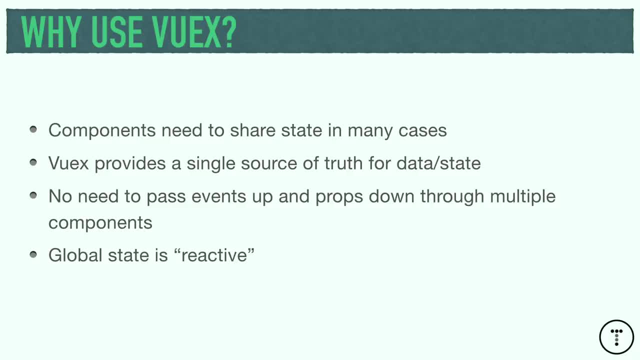 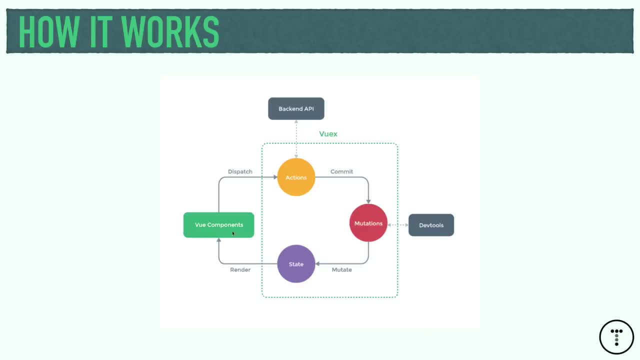 uses that state will also get updated at the same time so let's take a look at a diagram to quickly show how this process works so we have our view component which can dispatch an action like let's say login or add post or something like that and that will make or it will make a request here to our back-end API whether it's your own API or some third-party API you're working with in our case it's going to be Jason placeholder and then we commit a mutation and that mutation updates or mutates the state in the way that we want so maybe it sets an authentication token it adds a new post and then it renders back it changes the state and renders back to the component or components that need to deal with that state so that's the gist of how it works 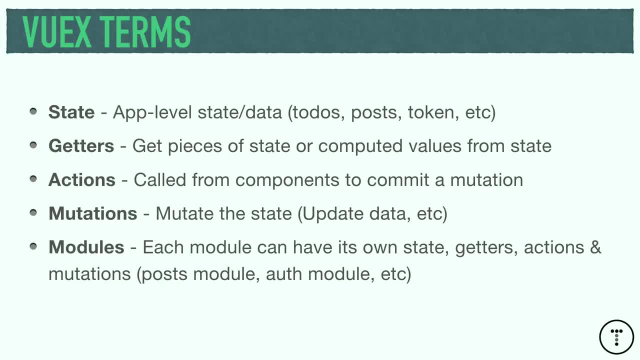 and this will make more sense once we jump into the code so as far as vocabulary we have a few you concepts that Vuex uses so we have state obviously which is your app level data such as to do's post authentication tokens whatever it may be getters which 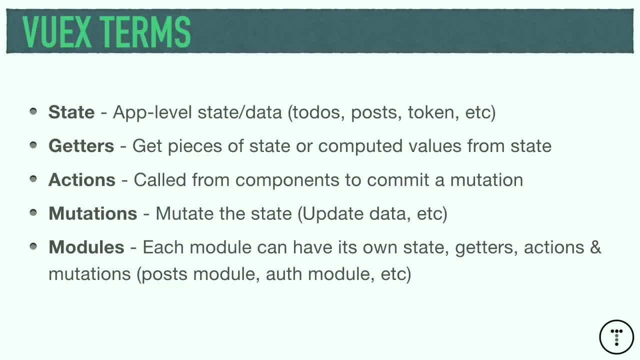 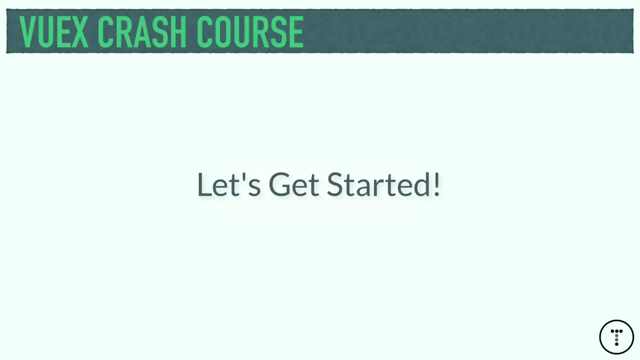 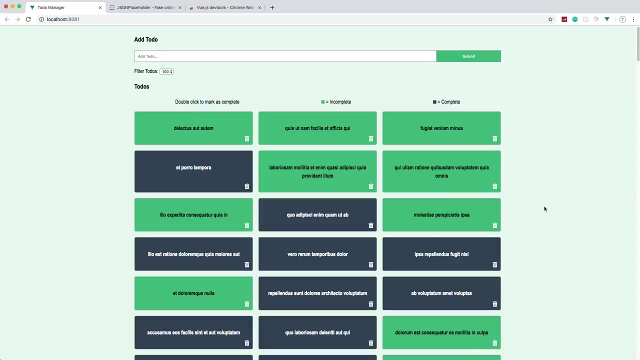 are pieces of state or computed values from state that we can bring into our components actions are used to commit some type of mutation to the state so we may have a form to let's say add a blog post we would fire an action and then commit a mutation to actually mutate that state and add that blog post okay we don't update or mutate state directly from the action we we commit a mutation okay and finally we have modules for different resources in our application similar to how we have multiple reducers and redux we may have for instance an authentication module that handles state that has to do with logging in and getting tokens and all that we may have a blog post module for adding updating deleting and getting blog posts so we might have a comments module so you can have multiple modules and they all have their own state getters actions and mutations all right so enough with the slide let's go ahead and jump in and let's start working with Vuex all right guys so a couple things before we start first of all I just wanted to show you the application we'll be building so it's gonna be a to-do manager and we're 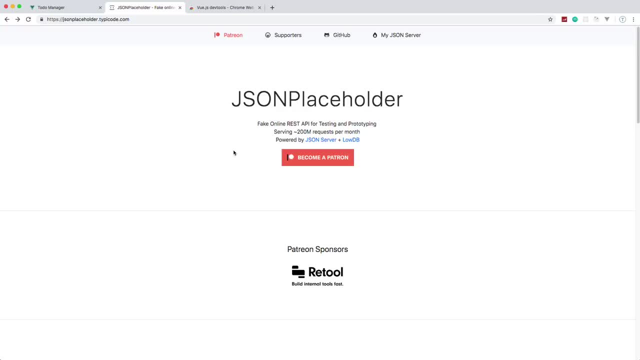 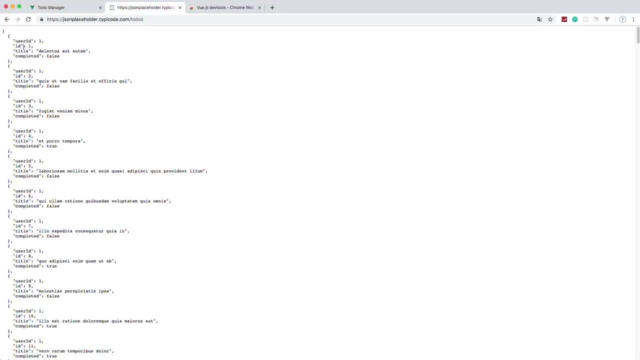 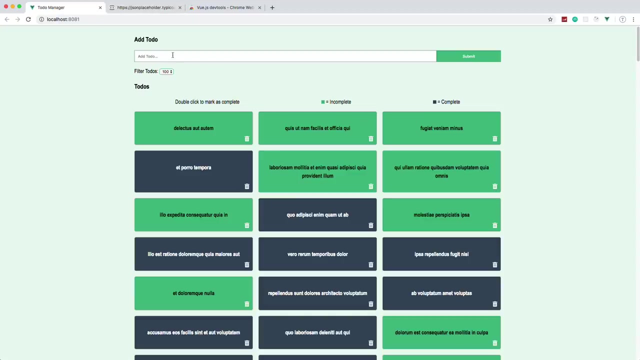 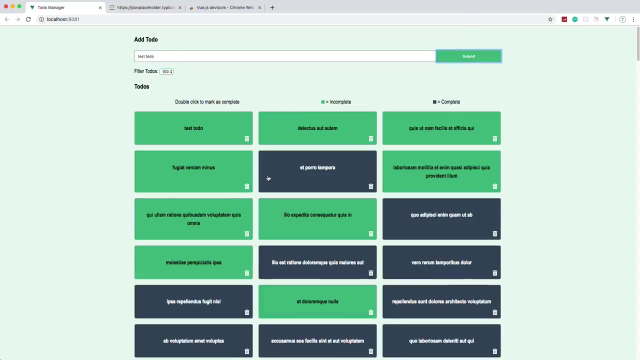 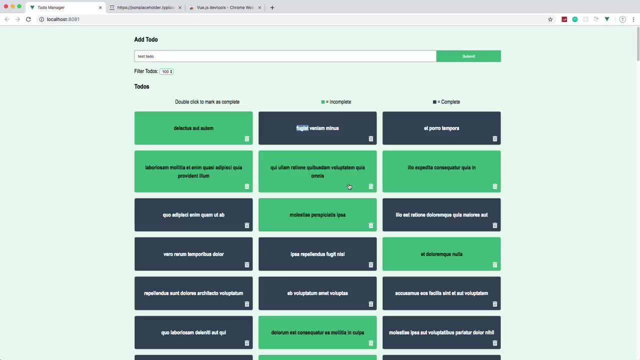 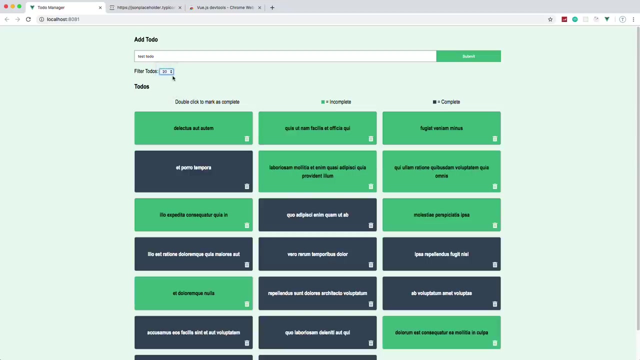 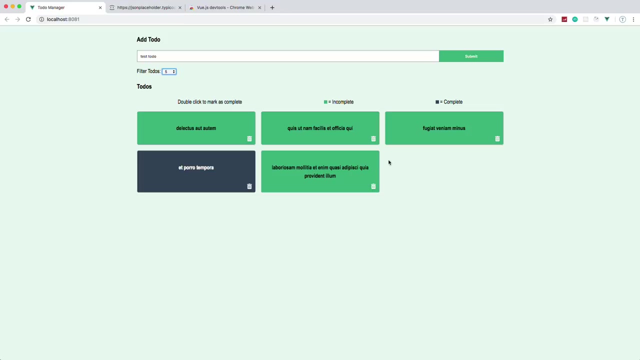 gonna be using Jason placeholder for our back-end rest API so as you can see it's a fake online rest API for testing and prototyping so it offers multiple resources we're gonna be using to do's and as you can see we can make get requests post put patch and delete requests and we can get up to 200 to do's as you can see so each to do has a user ID and ID a title and a completed value which is randomly true or false so that's the data we'll be dealing with and we'll be able to make a post request to add it to do so I'll say test to do we'll submit and you can see it gets added here we can go ahead and delete with the little trash can icon we can set them to complete by double clicking you can see it changes the color we have a little legend here that tells us that green is incomplete and blue is complete so we can change that change that also change it back we can also filter so let's say we want only 50 or we want 20 or 10 or even just five to do's all right so quite a bit of functionality in this little application another thing I want to mention is I would highly recommend using the vue.js dev tools if 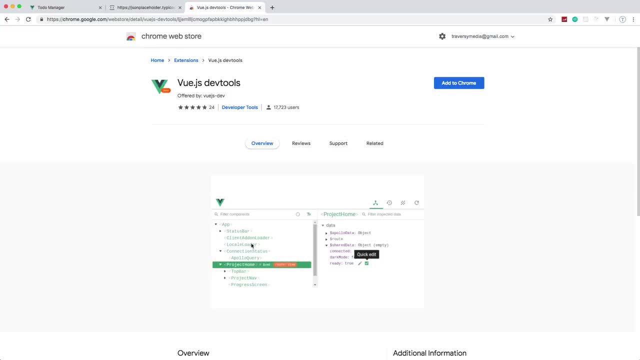 you're using Google Chrome because it shows you not only your view components but it also shows you your vuex state your mutations everything like that so it's really helpful and something I definitely recommend when working with 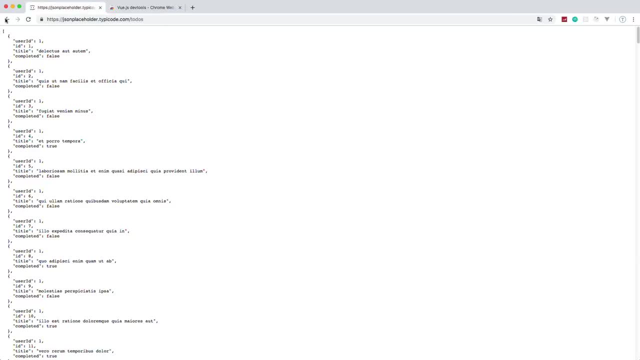 vue.js all right so I'm going to go ahead and just close that up I'm going to keep Jason placeholder open and now I'm going to jump into vs code so I just have an empty folder called vuex to do manager 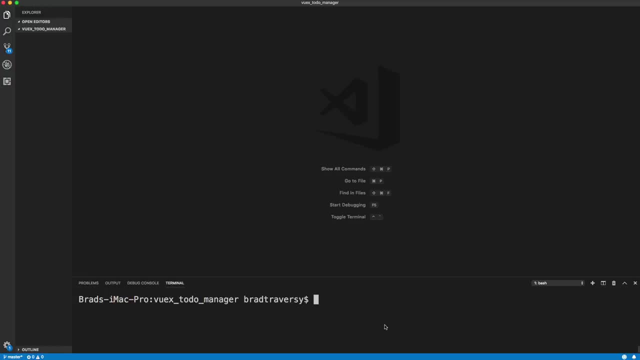 and first thing we want to do is generate a vue application now you're going to need to install the vue CLI if you don't already have it installed and you want to install that globally so NPM install dash G and it's going to be at vue slash CLI okay I already have installed so I'm not going to install it but once you have that set up on your system you can check with vue dash dash 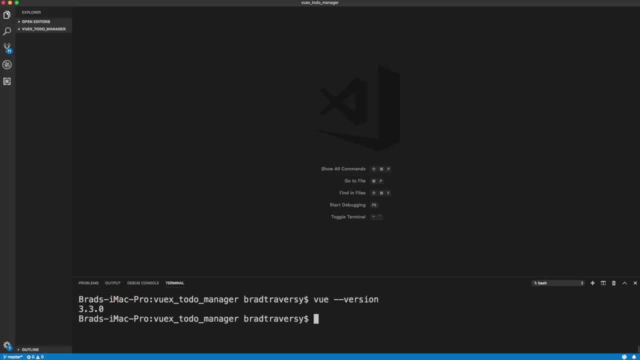 version you can see I version three point three point zero and then let's just run vue.js create now since I want to create it in this folder I'm just going to say dot 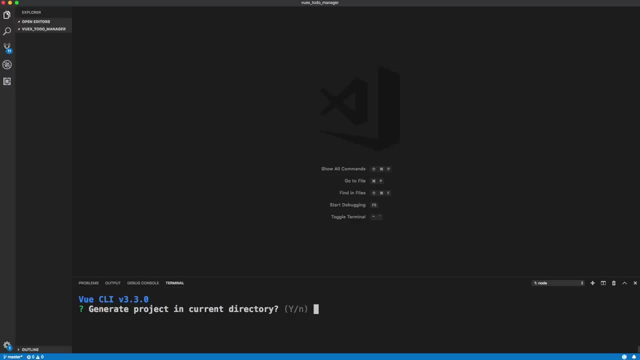 otherwise you could spell out a folder and it would create that folder for you 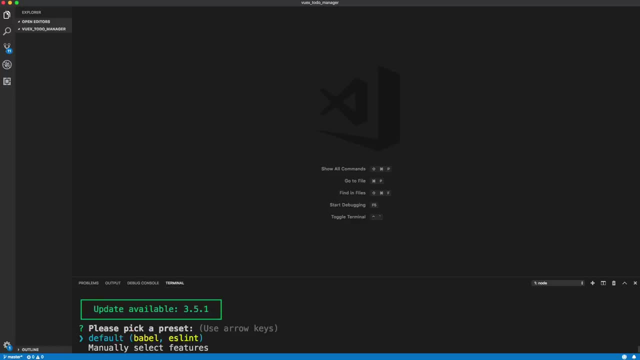 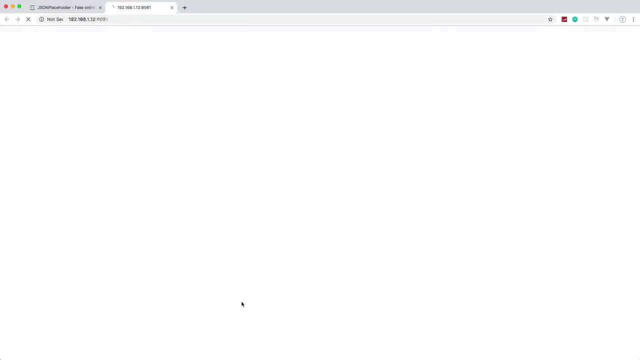 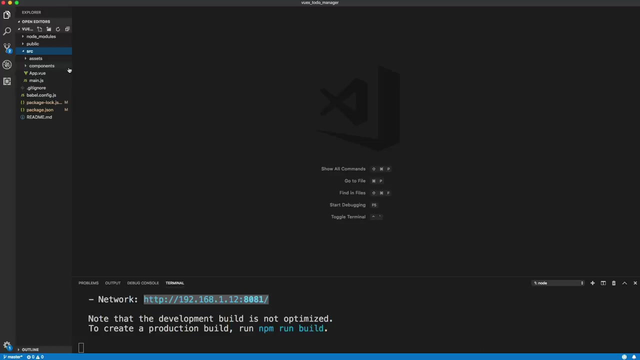 so I'm going to say yes I want it in this directory I'm going to choose the default here and it's going to generate our default application alright so now that that's set up let's go ahead and install our dependencies so all we're going to need is vuex and I'm also going to install axios which I'm going to use to make HTTP requests to Jason placeholder and if you want to use the fetch API that's absolutely fine I just prefer axios so I'm going to install those two dependencies all right that should be all that should be it so now we can go ahead and run NPM run serve that will open up our vue application so you can see for me it's on port 80 81 so go ahead and go ahead and control click that and you can see we have our default vue app alright so Let's jump back into VS Code and go into the source folder. 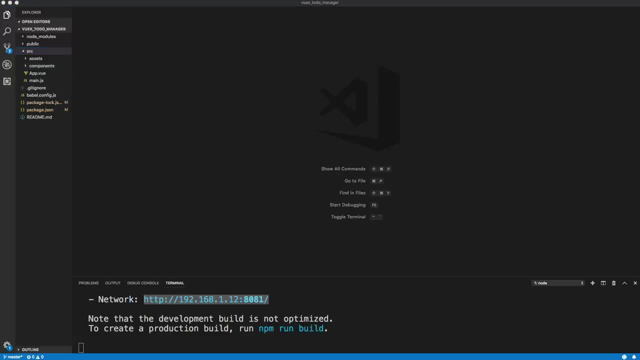 And the first thing I want to do is create a to-dos component. Ultimately, we're going to have three different components. 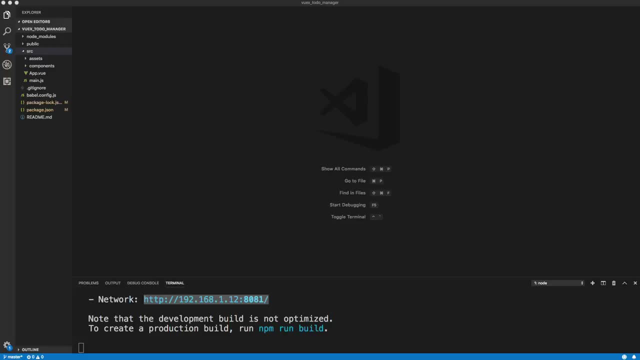 We're going to have to-dos, add to-do, which will be the form, and then filter to-dos. 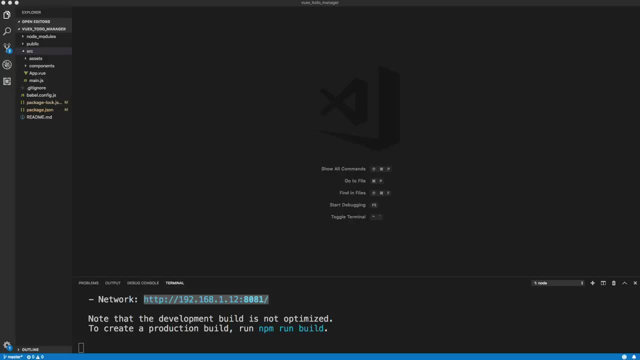 And the idea is that we want to access the application level state in Vuex from all three of these components. And I'm going to show you how to do that. 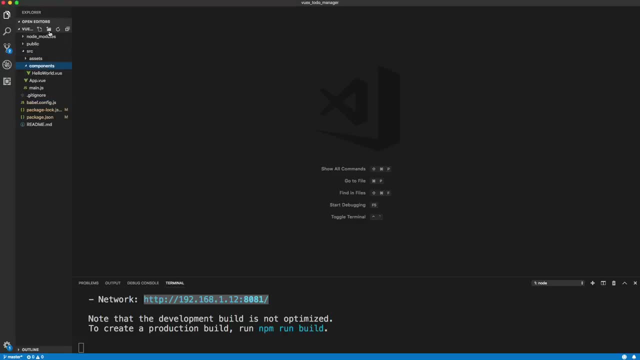 But let's start out with just creating the to-dos component. So under Components, I'll create a file called to-dos.vue. 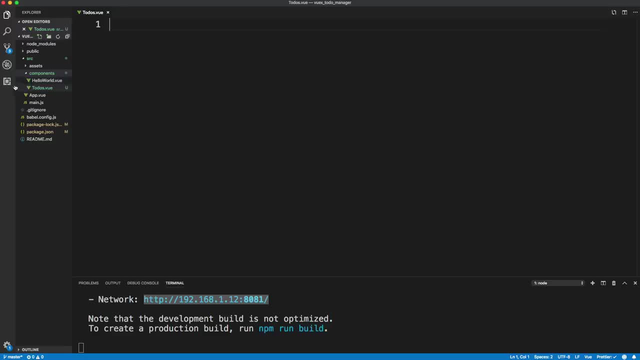 And another thing I want to mention is if you're using VS Code, 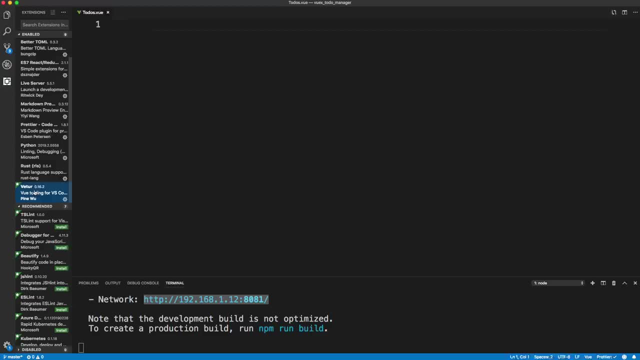 I'd highly recommend using the VUTER extension here, which gives you syntax highlighting snippets. 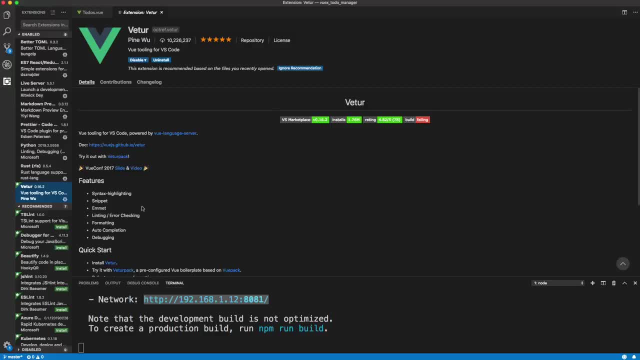 It allows you to use Emmet within your Vue templates. So it offers a lot. It's a great extension for Vue. 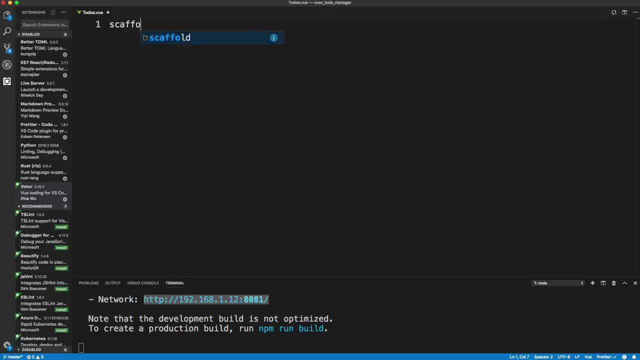 And using that extension, I can actually just say scaffold, and then hit Enter, and it will scaffold out what we need for our Vue component, so the template, the script, and the style. 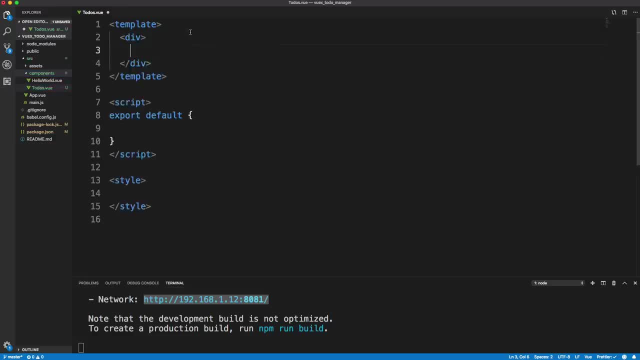 So for the template, I'm just going to put in a div for now. And let's do an h3 and just say to-dos. And in the export default, we want to export the name, which is going to be to-dos. 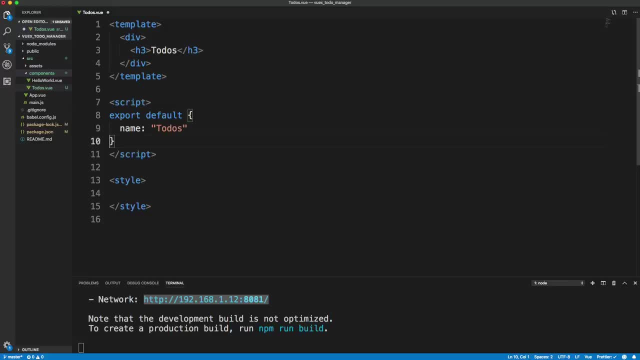 And I'm not going to go over the basics of Vue.js. I do have a Vue.js crash course if you're not familiar with the framework itself. 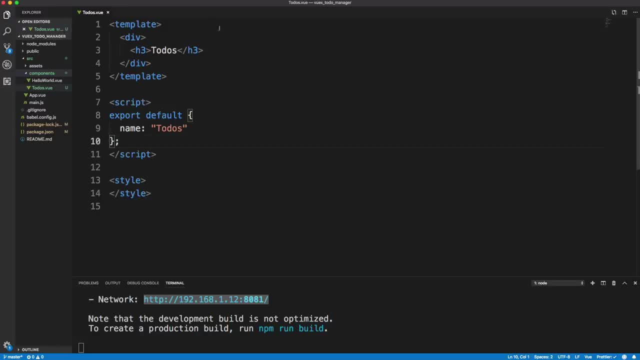 This is a Vuex tutorial. So let's save that. 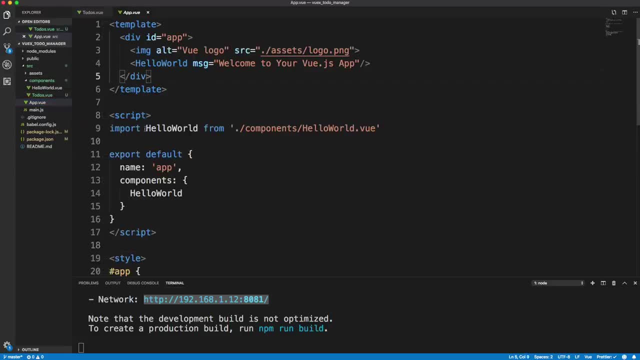 And let's go into our app.vue file. And we're going to import, instead of this hello world component, we're going to import to-dos. And we want to bring that in from to-dos.vue. And we're going to change this down here to to-dos. And then up in the template, let's get rid of all this. And let's just put in our to-dos component. And I'm also going to get rid of this default, the styling, right here. And let's save that. And if we go back to our application, 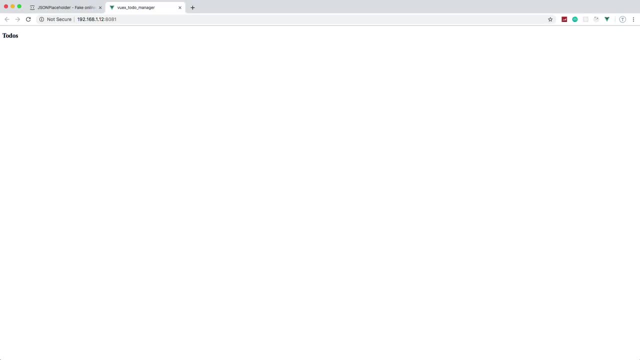 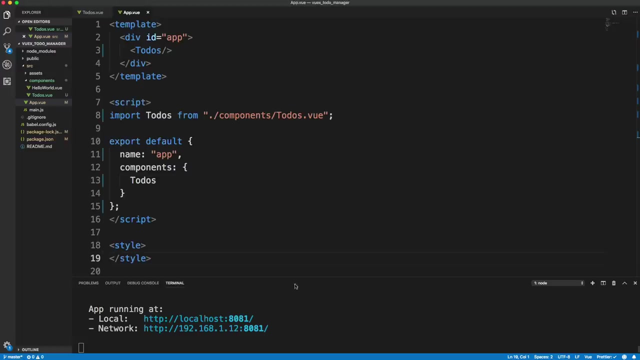 we should just see to-dos. All right, now I'm going to have some styling. We're not using any framework or anything. I wanted to just do some simple custom styling. So for the CSS in the main component here and some of the other components, I'm just going to paste it in. 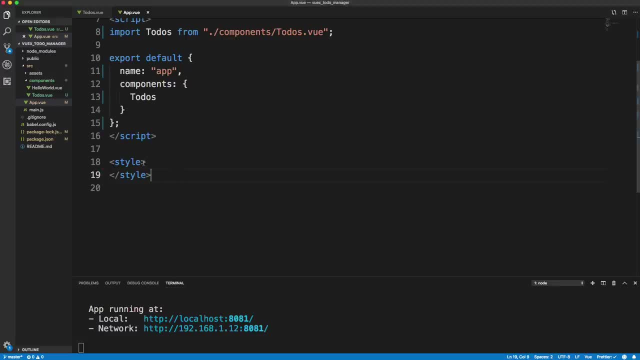 I don't want to waste too much time typing out CSS. So I'm just going to go down to the style here and paste in a couple of things. So just some styling on the body. And then a container that has a max width and centers it with margin auto. So pretty simple. And if you want to pause the video and type it out, you can do that. 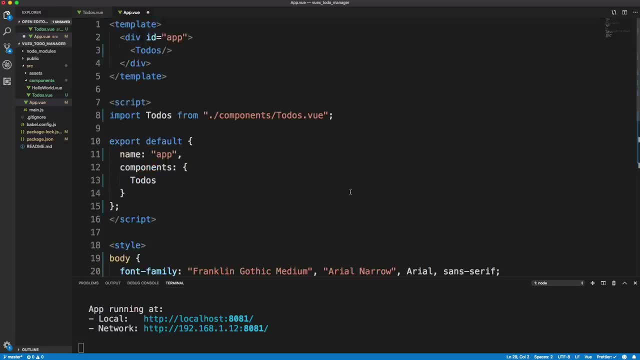 Or you can just go to the repository in the description and grab it from there as well. 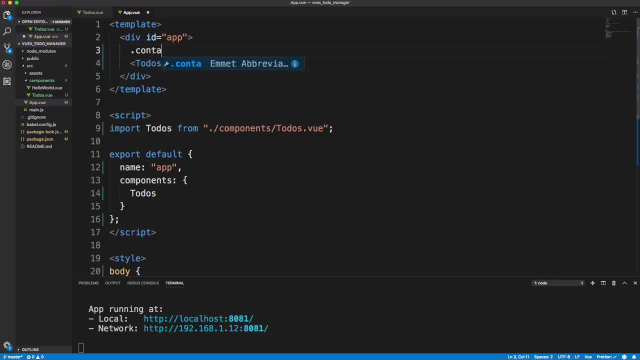 But I am going to put a container class around our component here, our to-dos. So let's just bring that up into here. OK, good. 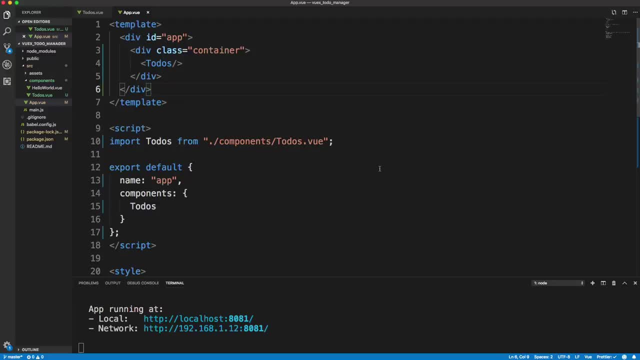 And I am using the prettier extension for VS Code. If you watch any of my tutorials, you know that I say that over and over just so you know that when I save, sometimes it formats things a little differently. So just to let you know. 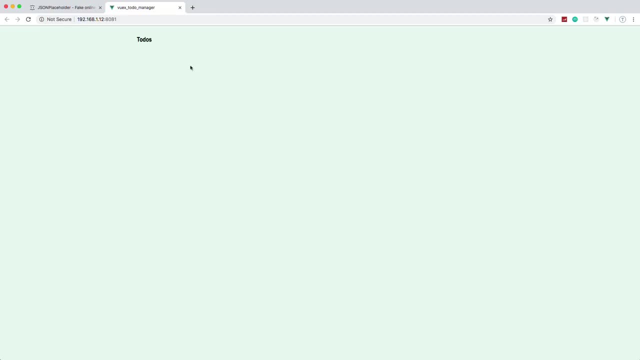 All right, so let's see. If we check it out now, we have our background color. We have everything centered. We have the font. Good. 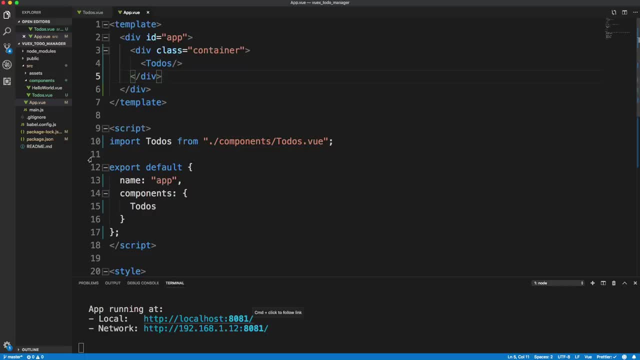 So now I'm going to jump right into Vuex, setting up Vuex. So the first thing we want to do is in our source folder, we're going to create a new folder called Store. OK. 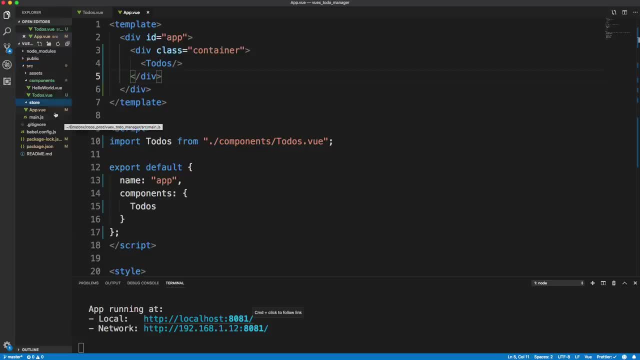 So we want a centralized store for all of our data, all of our state. And in Store, I'm going to create a file called index.js. 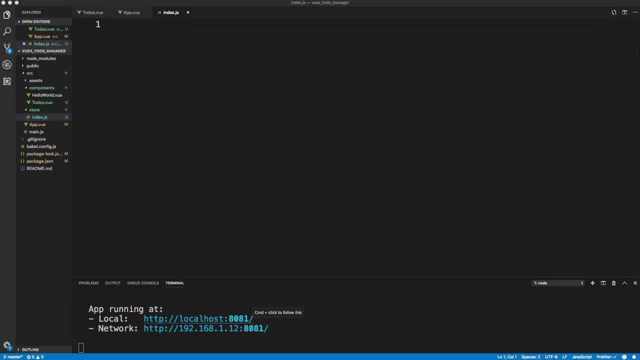 OK, so this index.js is basically an entry point to Vuex. And it's where we combine all of our modules. Now, if you use React with Redux, you know that you usually have a root reducer. And then you have multiple reducers that you combine together. 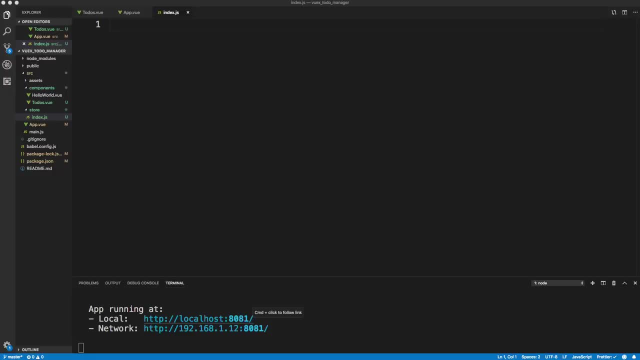 And that's kind of what we're doing here is we bring in all of our modules, and we add them to our Vuex store. 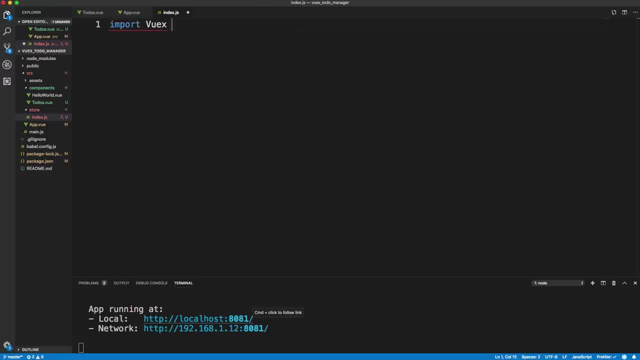 So first thing we want to do is import Vuex. So we're going to import Vuex from Vuex. And we're also going to import Vue. 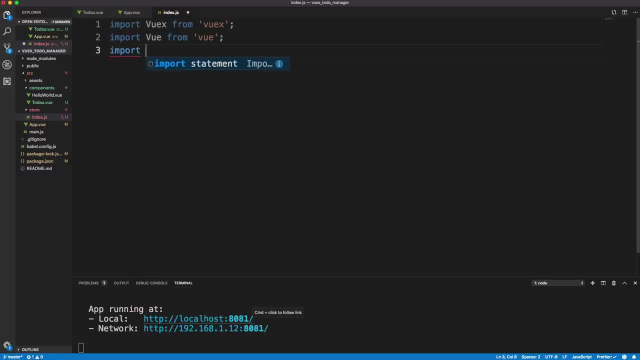 And let's also import our to-dos module, which we haven't created yet, but we're going to in a second. So we'll say import to-dos from, and it's going to be dot slash module slash to-dos. 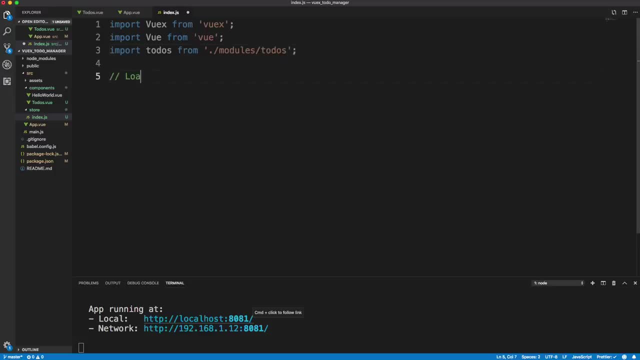 All right, now down here, we want to load Vuex. And the way that we do that is we take Vue, and we just call dot use, just like you would with the router. And you just pass in Vuex. Now we want to create our store. And we do that by export default new Vuex dot store. And we simply pass in an object with a modules object. And any modules we have, we just add here. So we have a to-dos module. 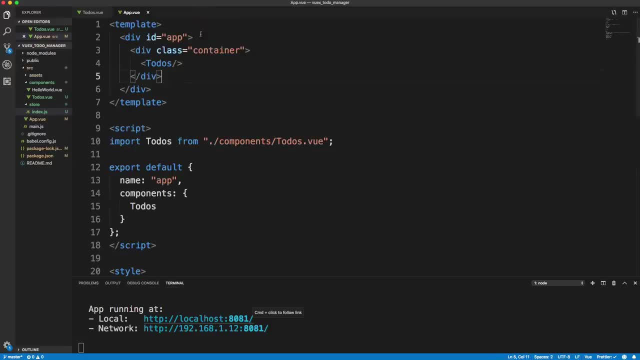 All right, and that's it. We'll save it, and that's it for this file. 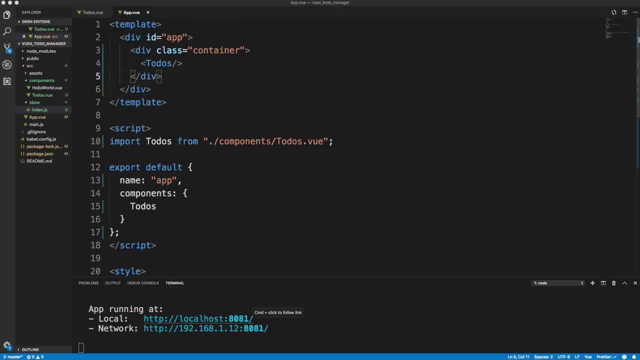 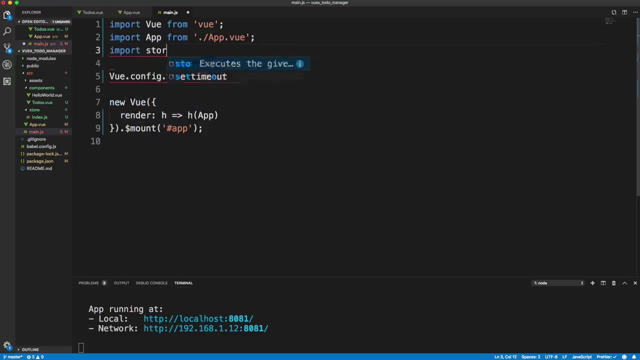 So in order for that file to do anything, we have to bring it in to our main dot js, which is basically our application starting point. I'm just going to save to format this a little bit. I use semicolons. You don't have to, but I choose to. And then we're going to import our store. 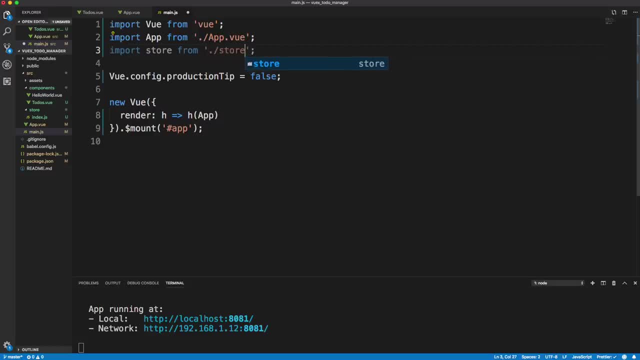 And it's in a folder called store. And since it's called index js, we can just do this. We don't have to do slash index. That'll bring it in. 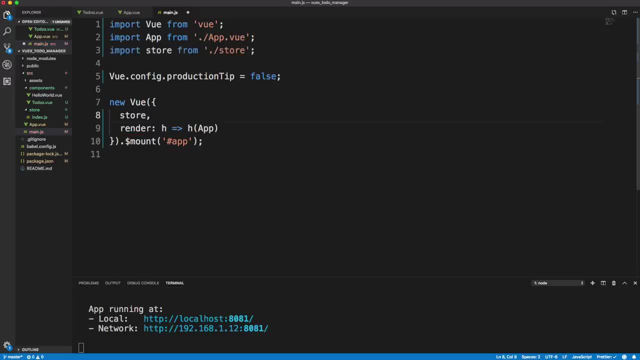 And then we just need to add it to our Vue instance like that. So I'll save that. 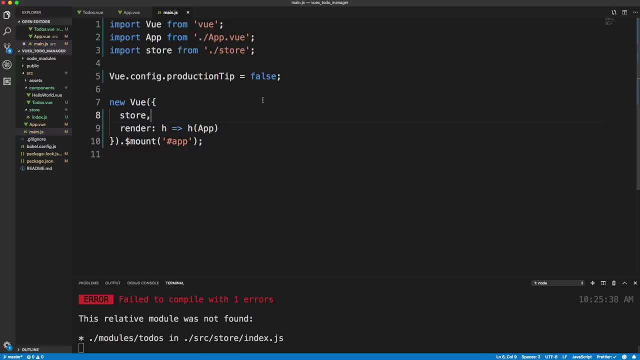 Now we're going to get an error that tells us there is no to-dos module. So let's create that. 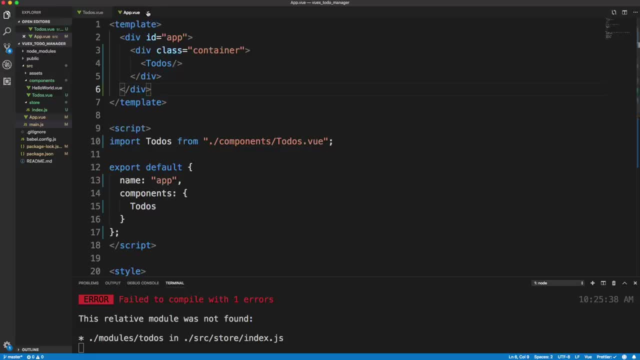 I'm going to close up main js. I guess I'll close up app dot Vue for now. 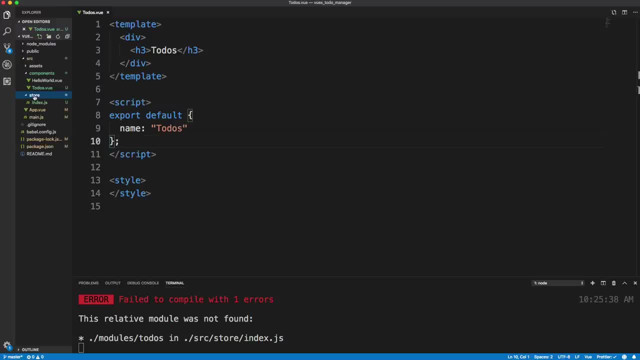 And let's open up, or let's rather create inside store. In our store folder, we want to create a folder called modules. OK. And then, whoops, that's a file. Sorry about that. We want to create a folder in store called modules. 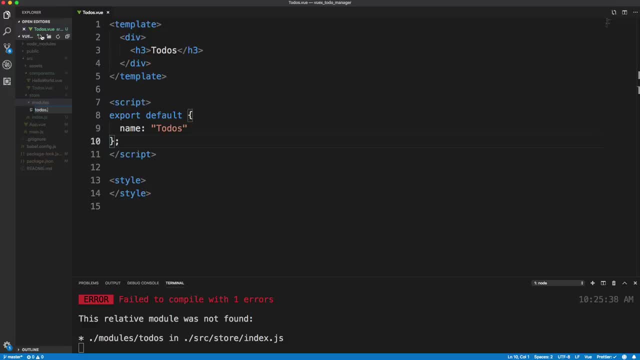 And then inside modules, we want a file called to-dos dot js. 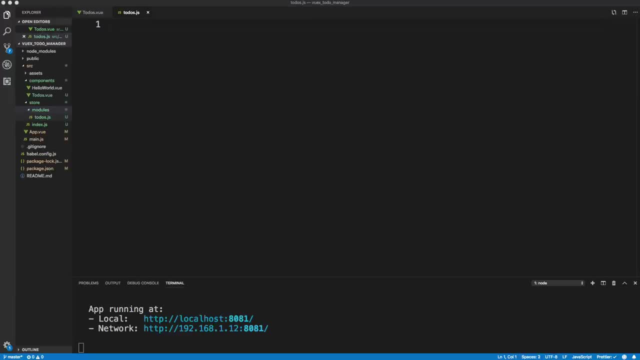 So this is our to-dos module. And this is where we put our state, our getters, actions, mutations, all that stuff. Now, we're going to make requests from here to our back end, which in this case, this is JSON placeholder. So I'm going to import axios for that. 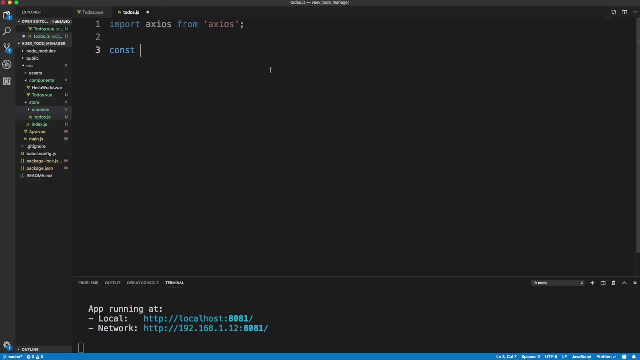 OK. And then we want to set, excuse me, we want to create four things here. 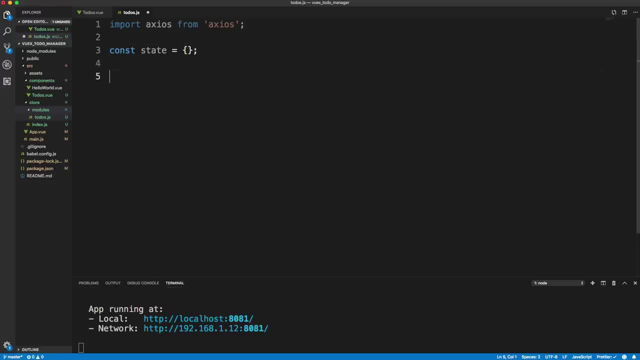 We want our state. So we're just going to create four objects, our state. We want our getters, actions, and mutations. 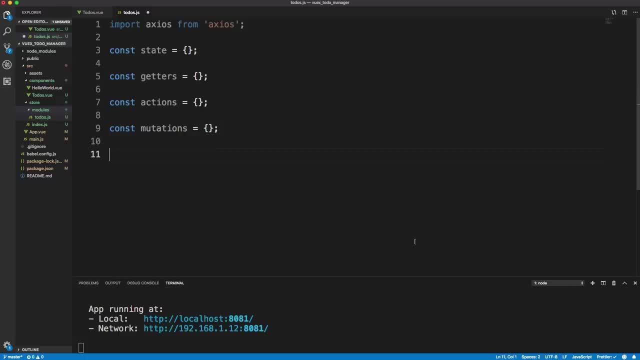 All right. So we have these four things. Now, we won't need to export these. So let's say export default. And we're going to export an object that has state. Now, we need to do like state, state. 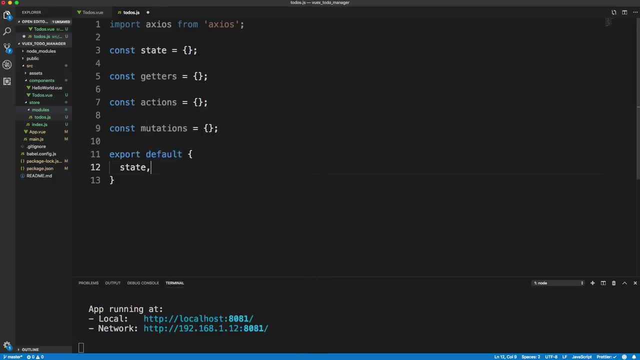 But with ES6, since these are the same, we can simply just do state. 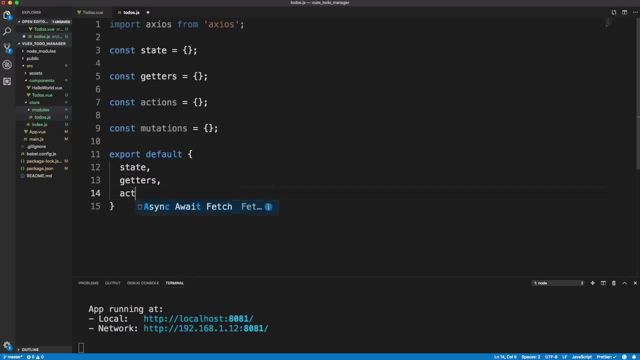 Same with getters and actions and mutations. All right. 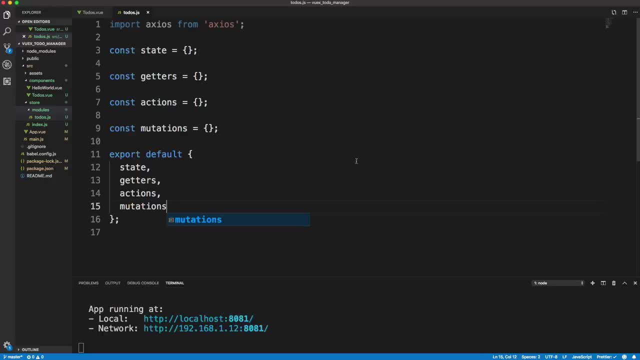 So I'll save that. And that's basically the boilerplate for a module. OK. All right. So we've got the same interface for our Vuex module. 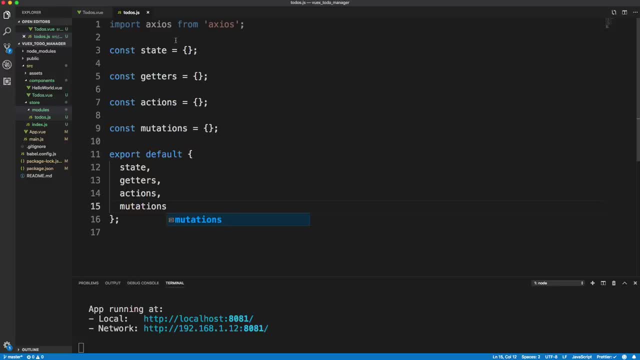 So what do we want to do here? We want to be able to get the to-dos from the application level state with Vuex into our to-dos component. 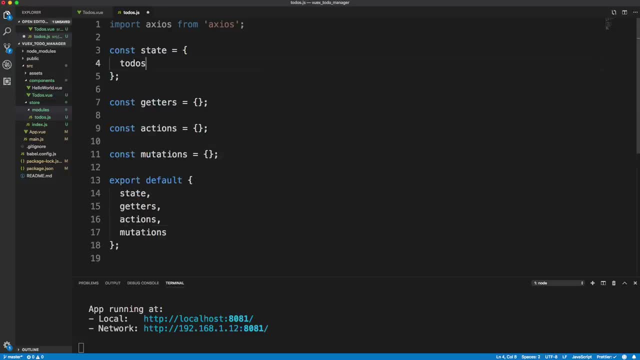 So for now, in the state, we know we want to-dos, which is going to be an array. And for now, I'm just going to hard code a couple to-dos in here. 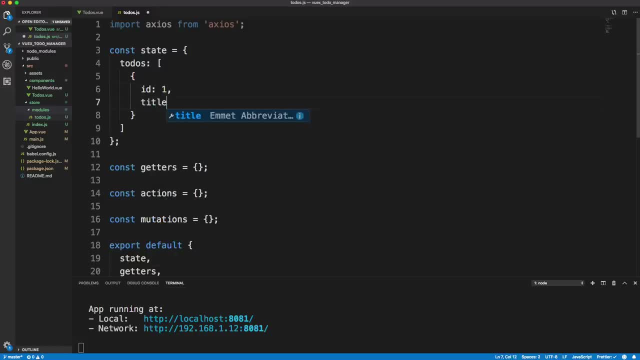 So I'm just going to do an ID and a title. So we'll say to-do 1. And we'll create another one. 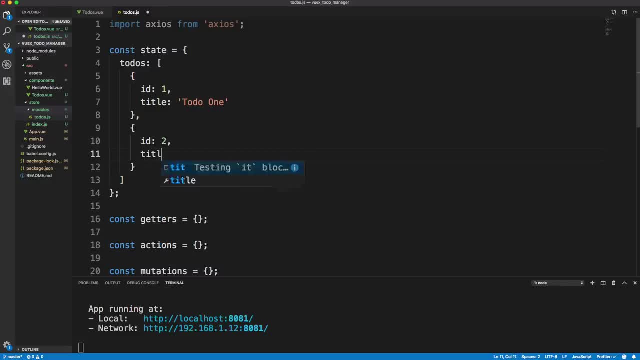 The ID of 2, title, to-do 2. OK. 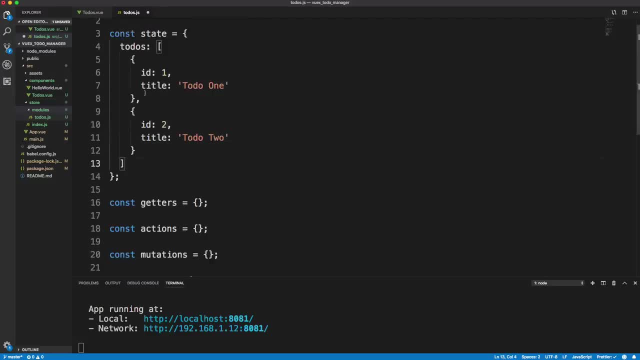 Now, in order for us to get this state into our to-dos component to display, we need to add a getter. So in the getters, let's create a getter called all to-dos, because that's what it's going to do. And this is going to be a function. We want to use an arrow function. 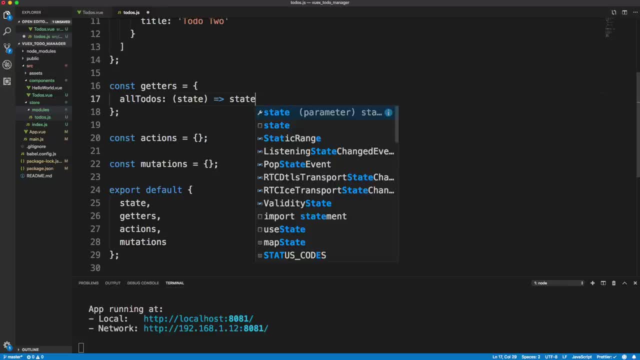 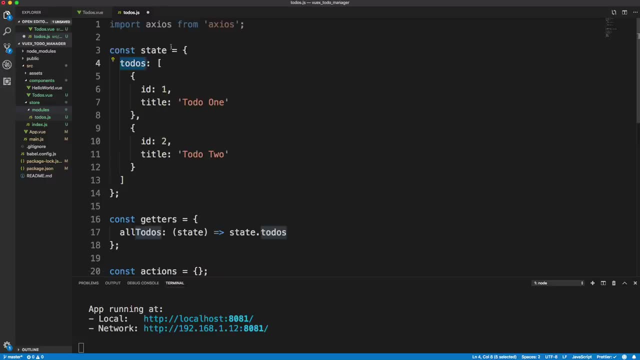 This takes in the state. And then we want to return state.todos. OK, because we want to get this part of the state. It's actually the only property we have in the state. Of course, we could have more. But in this case, we only need this to-dos array. So we're just returning that from the state. So I'm going to save that. And now we can go into our to-dos.vue file. 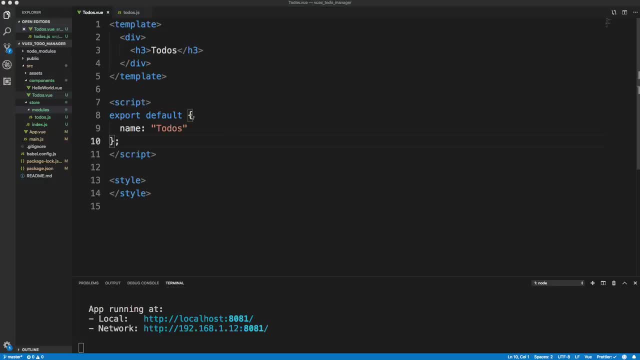 And we need to be able to use that getter. So in the script, we want to import something called map getters, which does just that. It maps getters from Vuex to our component. It's kind of like how Connect works with React Redux. I'll be making a few references to Redux, because I know a lot of you guys have worked with React and Redux. And this is very similar. 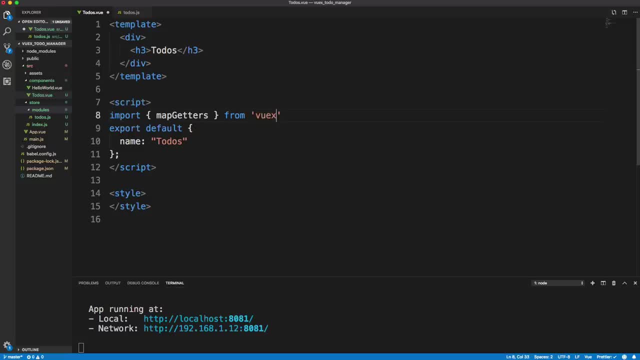 Easier, in my opinion. So we want to bring that in from Vuex. 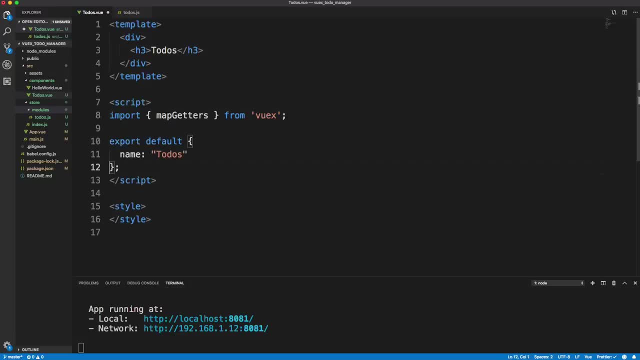 All right. And the way that we implement the map getters, or how we define which getters we want to use, is within the computed property. So we want to add in computed. And we want to just say map getters, and then pass in an array of the getters we want to use. 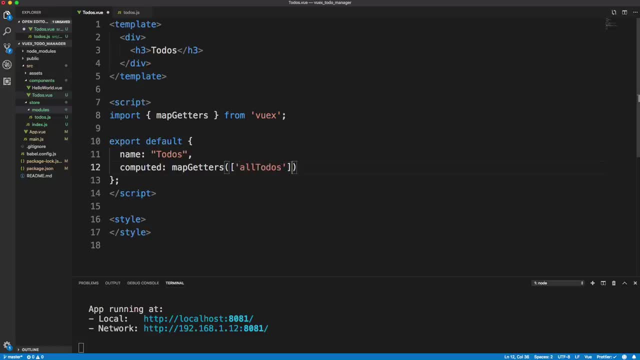 And we only have one, which is all to-dos. So just doing that is going to allow us to use this getter, which remember, returns the state, which has the to-dos. Or returns just the to-dos from the state. 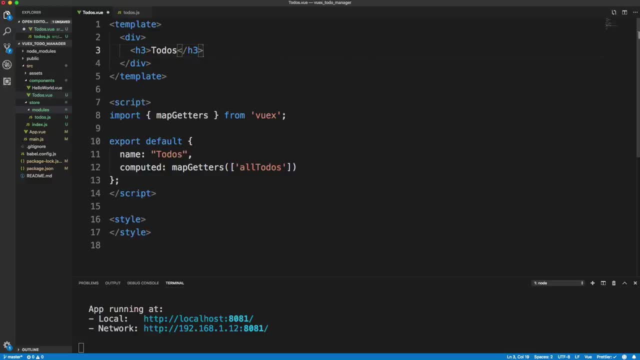 So I'm going to now go up to the template here. And I'm going to create a class, a div with the class of to-do. Actually, to-dos, sorry. And within that, we'll create a class of to-do. 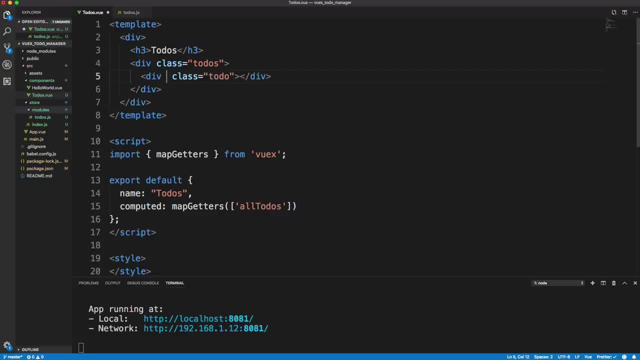 And this is the div we want to basically loop through and output this div for each to-do. 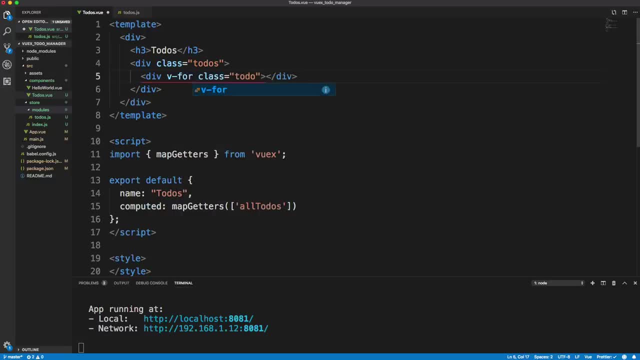 So in Vue.js, what we do is add a v-4 directive. So we'll say v-4. 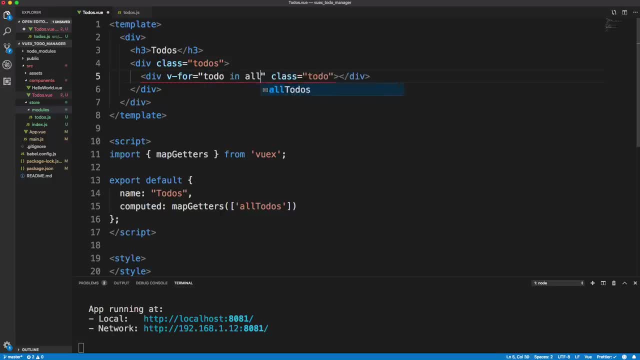 And we're going to say to-do in all to-dos. And we're getting this error here, this linting error, because we don't have a key. When you loop through something like this, you need to have a unique key. 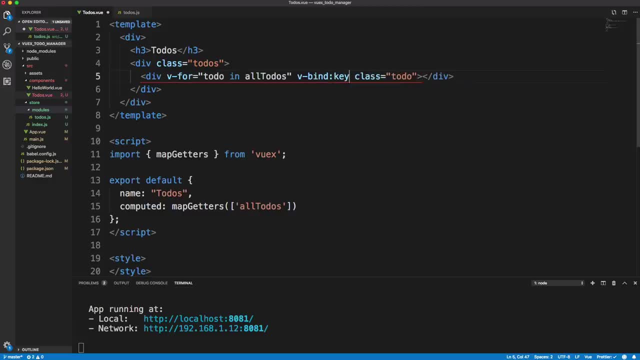 So we want to v-bind a key. And we're going to use the to-do ID, because that should be unique. 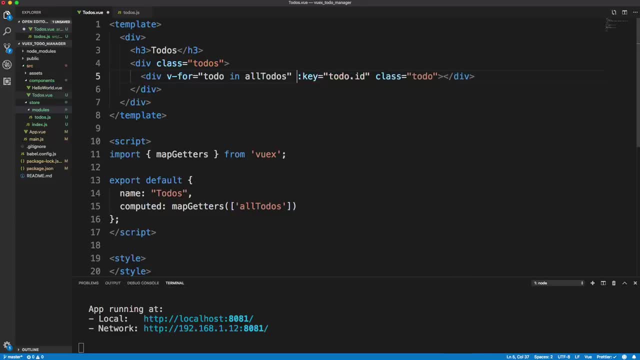 And in Vue, we actually don't need the v-bind. We can shorten this with just colon key. OK. 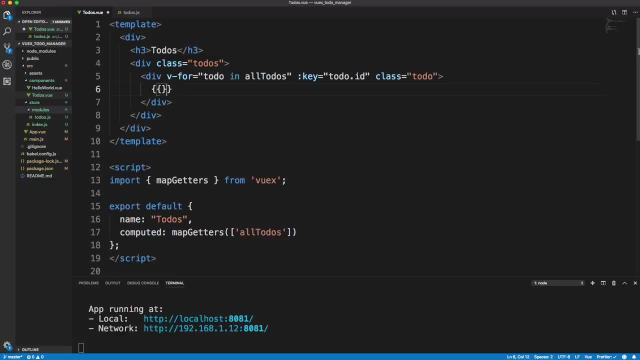 And then in the div here, all I'm going to output right now is the title. So we can say to-do.title. 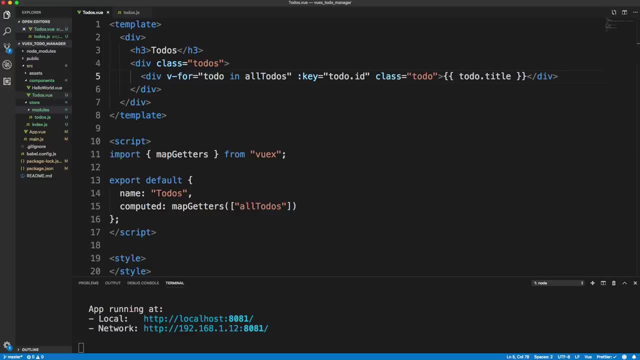 So we'll save that. Prettier just kind of formatted it a little bit. 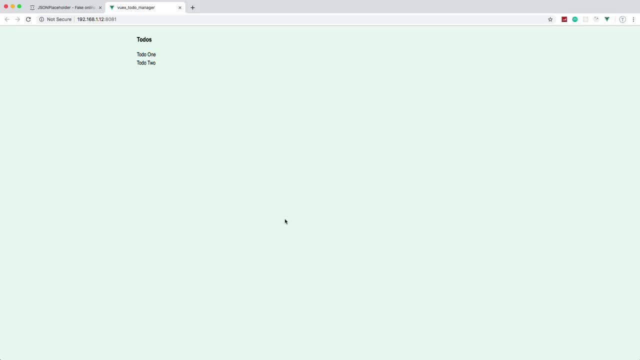 And we'll go back. And we can see to-do 1 and to-do 2. Awesome. 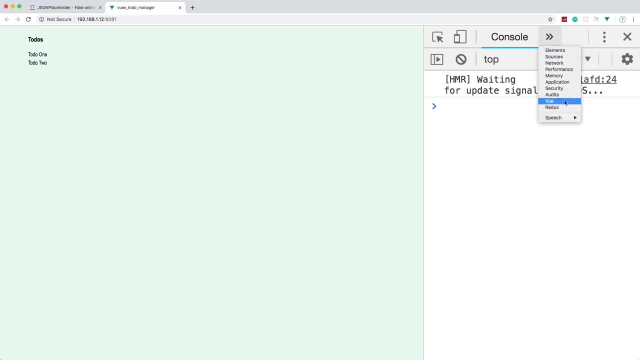 So if we open up our, I almost said Redux tools, our Vue tools here, you can see we have app. We have to-dos. And it even shows us down here the Vuex bindings of all to-dos. 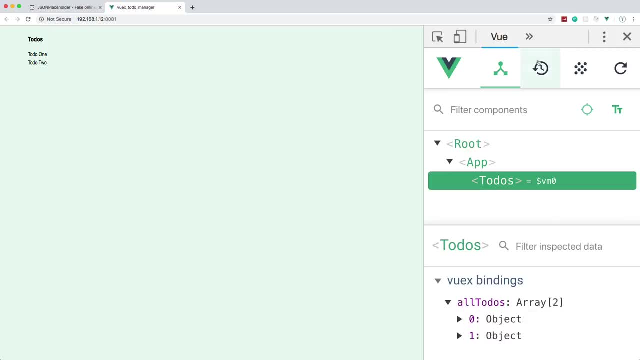 Which has two objects in it. And if we click this right here, this will show us basically everything 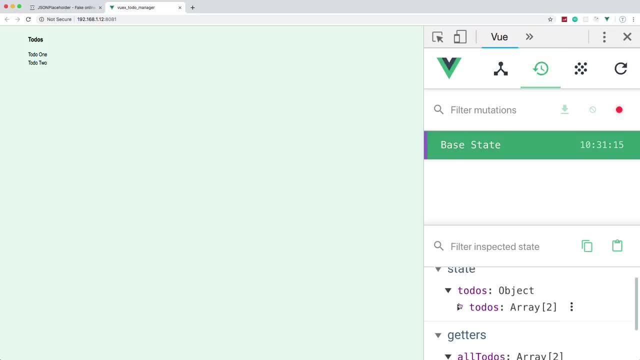 that has to do with Vuex. So down here, it shows us our state. And it also shows us our getters. So this is helpful for debugging and stuff like that. And just seeing the state of your application. So obviously, actually, you know what? 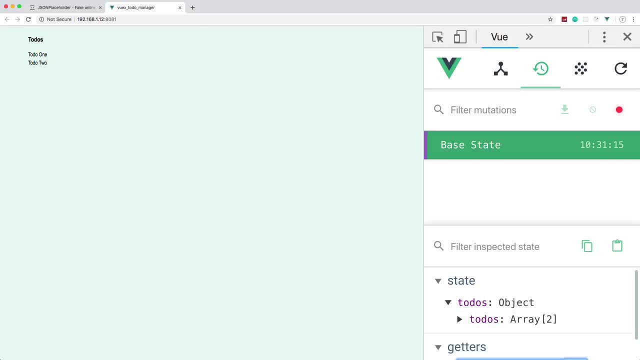 One thing I want to do before we move on is just add a little bit of CSS here. 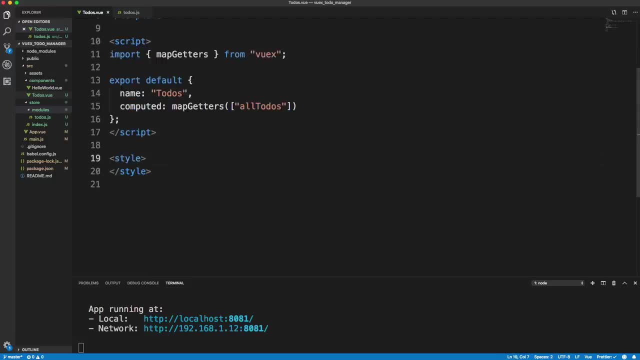 So. In the to-dos component, I'm going to go down to style and just add scoped. 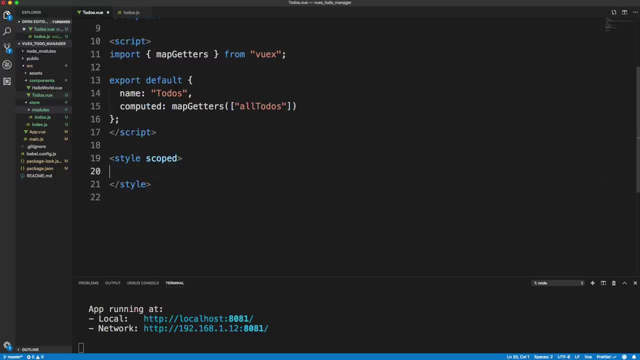 Meaning it only pertains to this component. And I'm going to paste in a little bit of CSS. I'm going to have more later. 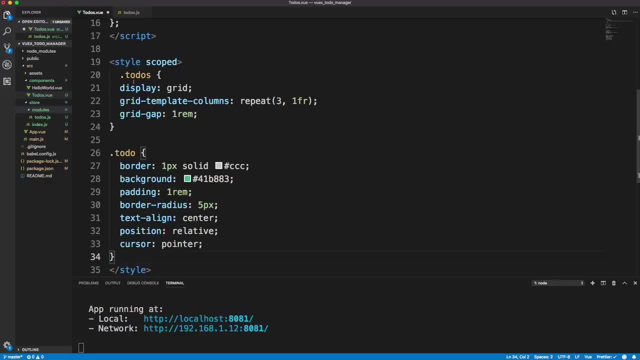 But for now, I'm just going to style the to-dos div and the to-do itself. So we're using the grid system. 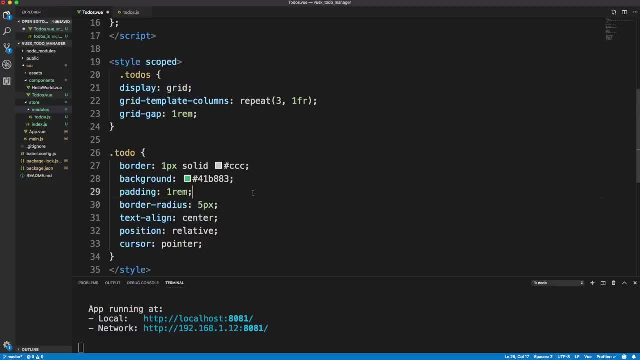 So we have three across. And we just want like a background, some padding, stuff like that. 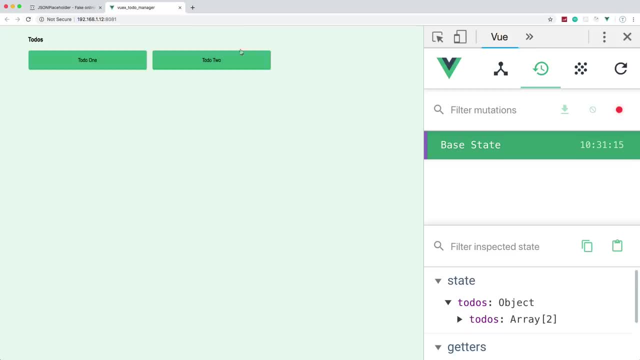 So save. And now if we take a look, reload. Should look like this. OK. 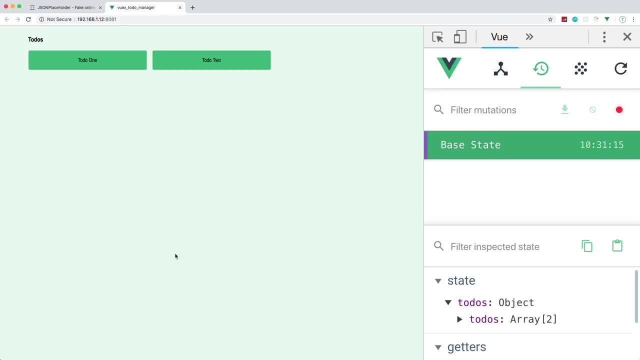 So we don't want hard-coded state, right? We want to pull it from JSON placeholder. 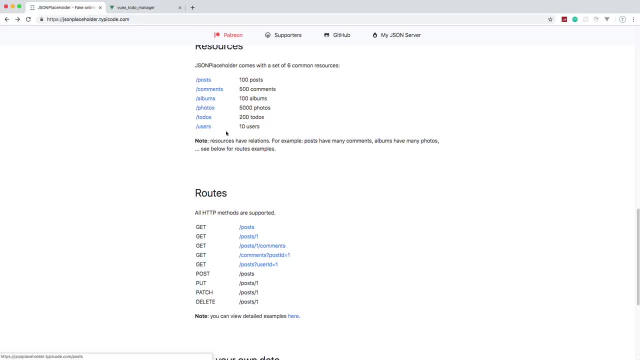 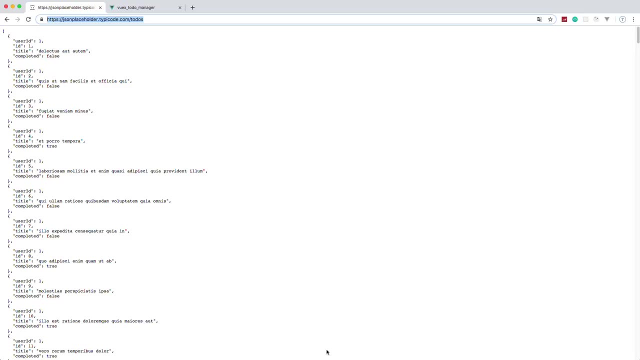 So if we go down here, you'll see that we can make a get request to this. Actually, we want this right here, to-dos. So we want to make a request to this URL to get this data, which is actually, I think, 200. 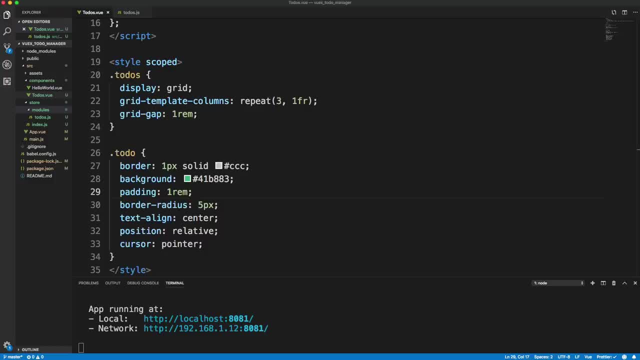 Is it 200? Yeah, 200 to-dos here. So let's do that. Let's go to our. Module. So our to-dos module. 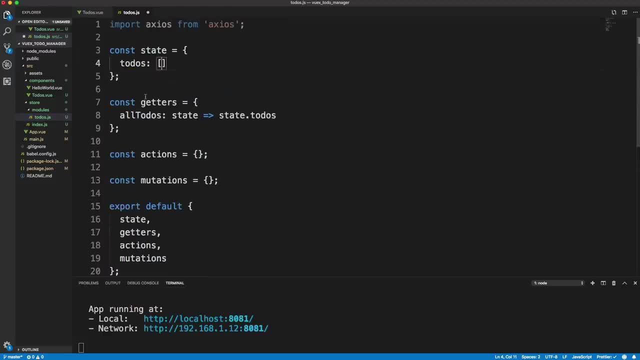 And I'm just going to make this state, this to-dos, an empty array again. 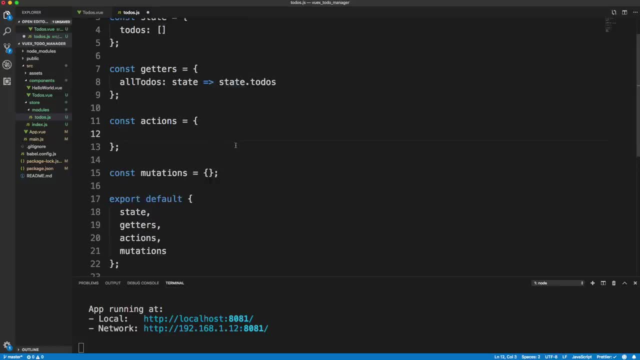 And we need an action that's going to make a request, get a response, and then call a mutation. OK. 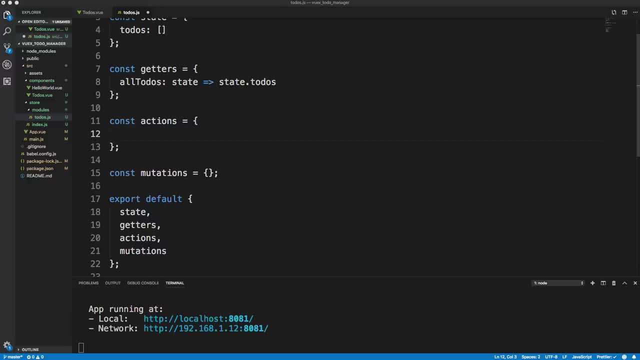 Because the mutation is what actually mutates the state. So let's create an action here. 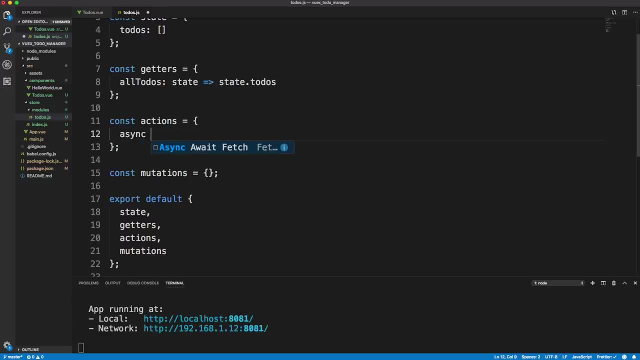 I'm going to use async await. So I'm going to label this async. And I'm going to call this fetch to-dos. OK. 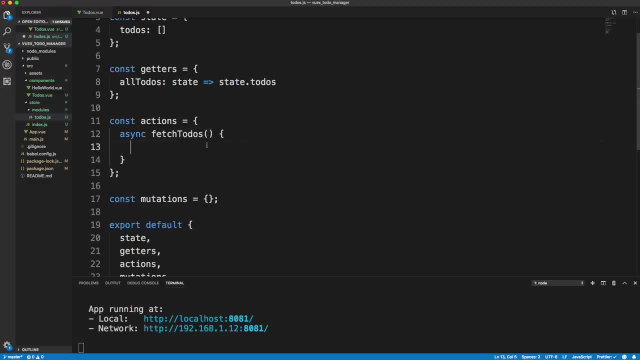 And I'm going to call this to-dos. Now, when you create an action, it actually 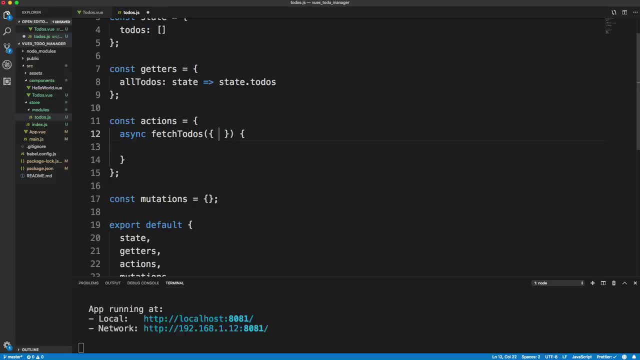 takes in an object, which I'm going to destructure. There's a few things in here. But what I want is commit, because that's what we actually use to commit a mutation. 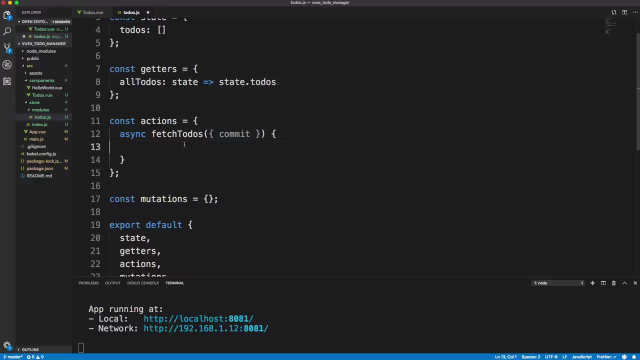 We don't call the mutation directly. We call it with this commit. All right. 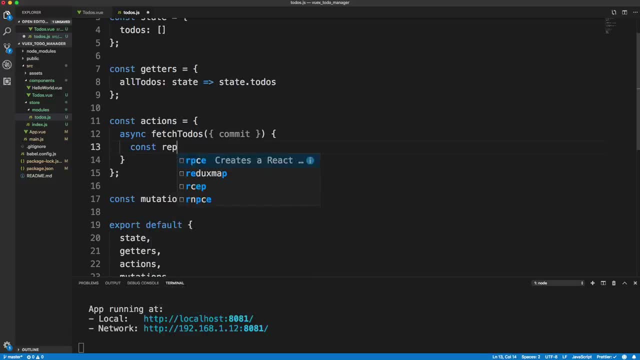 So let's make our request. So it's going to get put in a variable called response. And since we're using async await, we need to say await. And then we'll use axio.sync.wait. axios to make a get request to, whoops, what did I just do? OK. We want to make a get request to this URL. 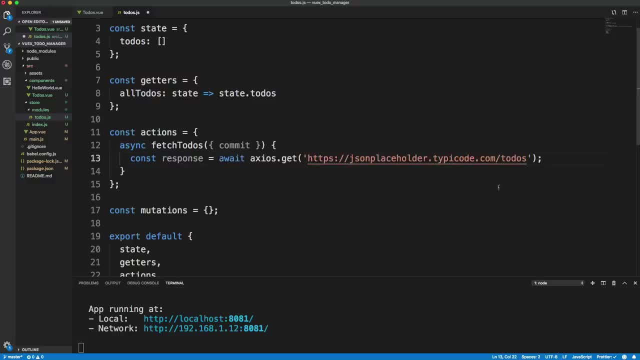 So we'll go ahead and paste that in here. Oops, I didn't put an equal sign here. And that will get our response. OK. For now, I'm just going to console log response.data. And that should get us our to-dos once this is called. Now. I'll go ahead. 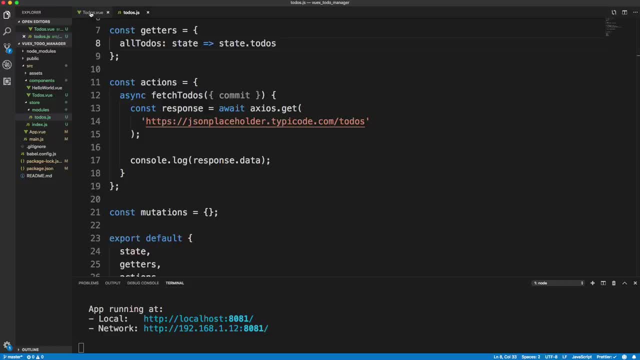 And save this. And let's go back into our to-dos component. 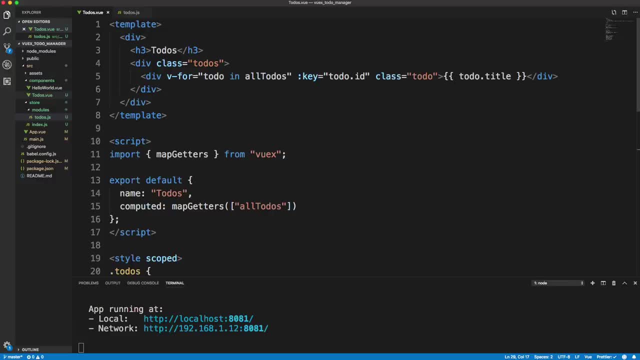 And we need to call that fetch to-dos action. OK. Right now, it's just going to console log. It's not going to do anything to the state. But I just want to show you how we can actually call it. 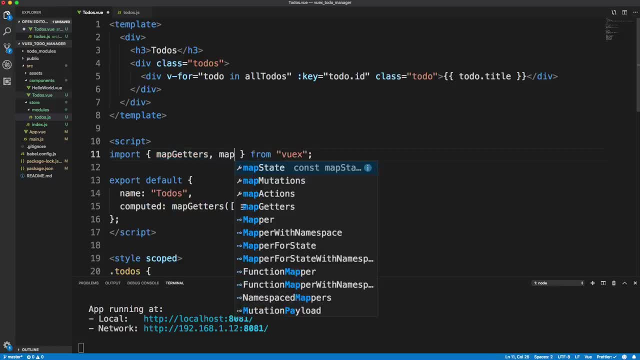 So to call actions, we bring in, instead of map getters, we bring in map actions. 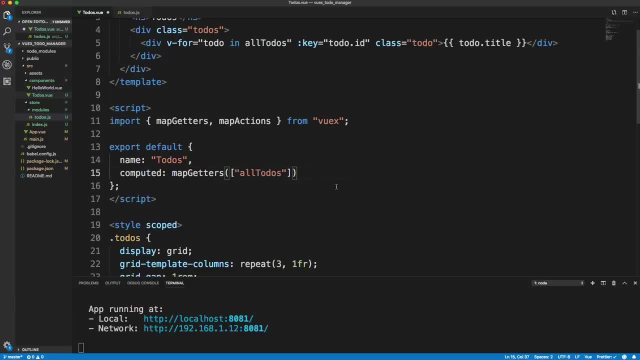 And where we add that is going to be in our methods, which I'm going to put right here. 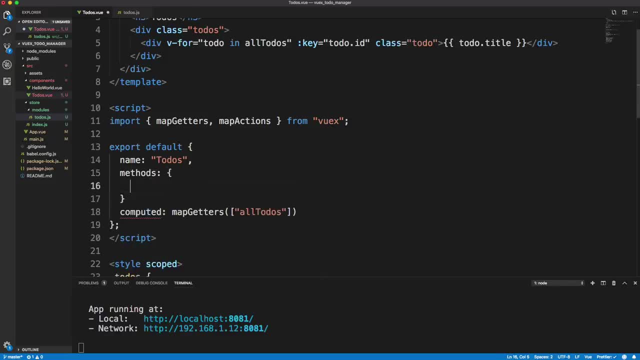 So methods and now I'm going to have multiple methods. So I just want to show you something real quick. 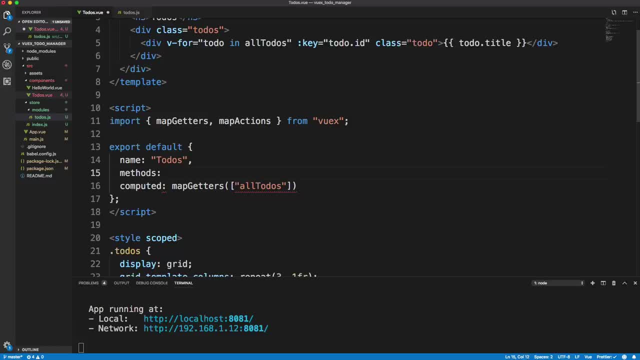 If we were only going to have actions as our methods, we could actually just put in map actions like this. And again, it takes in an array of the actions you want to use, which in our case is fetch to-dos, put a comma here. So we could do that. 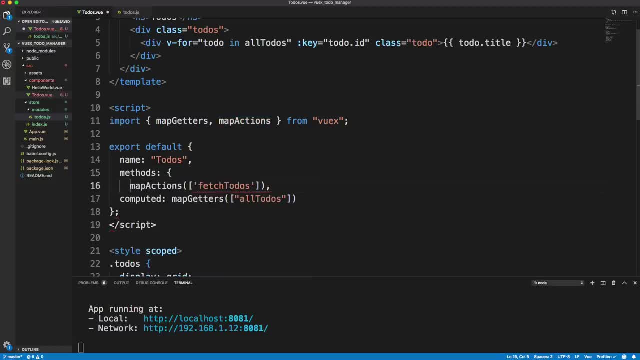 But I'm going to have other actions. So we're going to actually wrap this in parentheses. I'm sorry, curly braces. And then just throw the spread operator on map actions. So this is the same as doing just map actions up here, 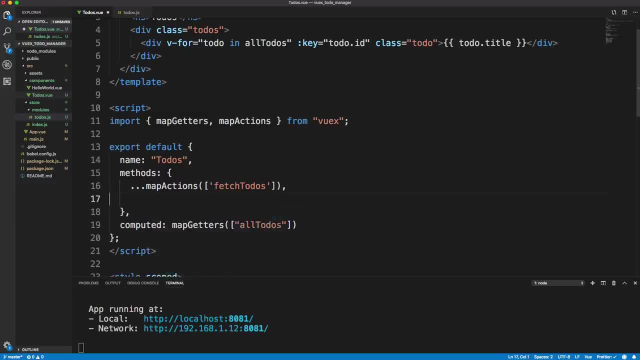 except we can now add other methods down here if we want to. All right. So I'm just going to leave that. OK. 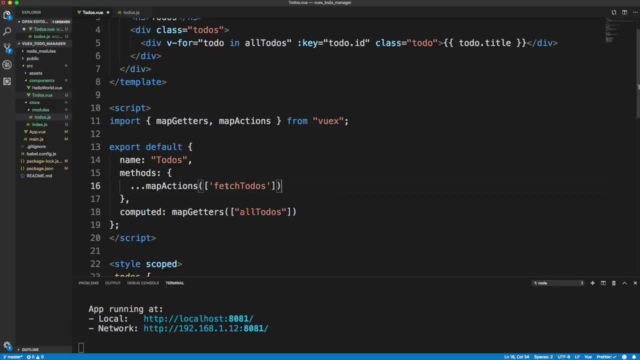 So I'm going to leave that for now. And this fetch to-dos, it's not getting called yet. We're just simply mapping it to this component. Where I want this to get called is before the component loads. So there's actually lifecycle methods in Vue.js. And one of them is computed. And that's what I want to use. So I'm going to say computed. And inside here is where I want to call that fetch to-dos. 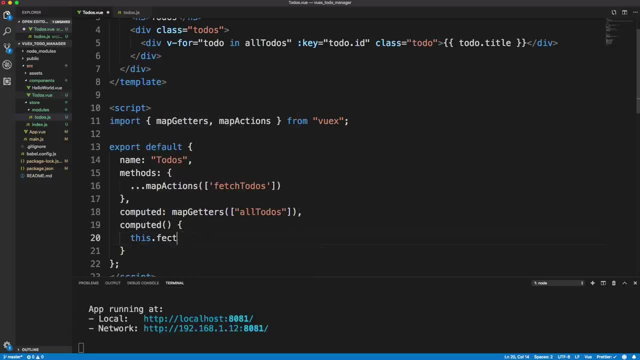 And to do that, all we need to say is this dot fetch to-dos. 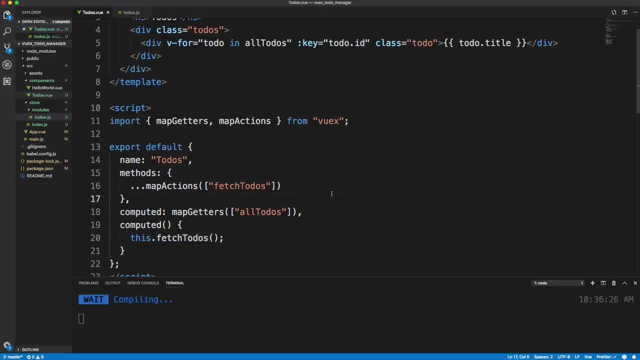 So that will actually call this action. So now I'll save. And as soon as the component is created, 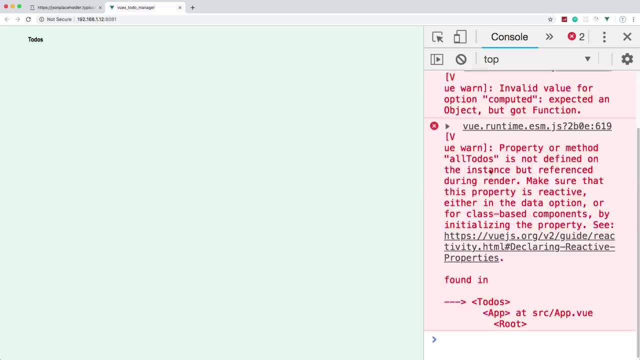 it should call that action, which console logs. Let's see. 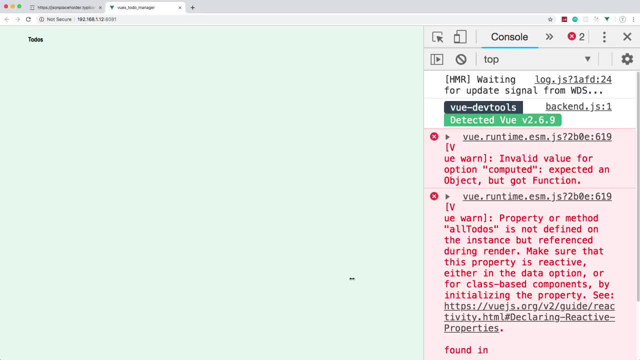 Invalid value for option computed expected an object. Oh, what did I do? I said computed. It should be created. Sorry about that. All right. 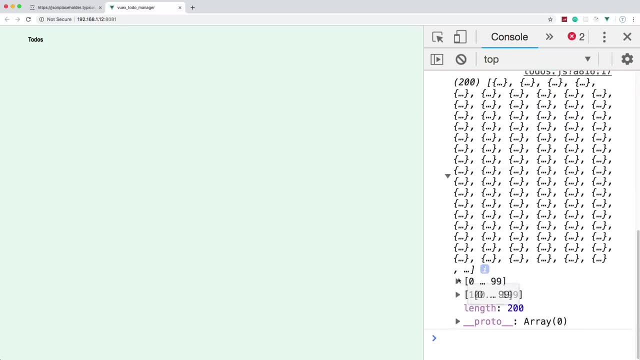 So now if we go back, you'll see that it's actually logging all of our to-dos. All right. Just reload that. Make sure we don't get errors. Good. 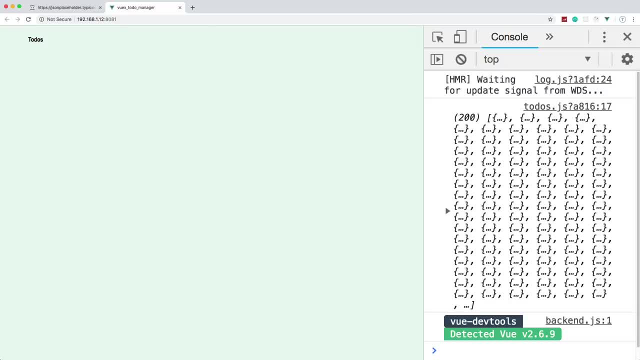 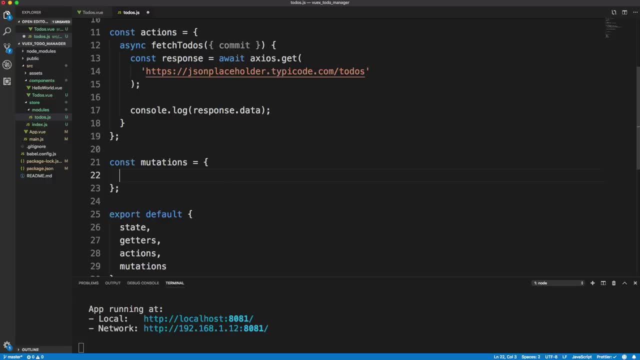 So we know that it's console logging. But now we need to add it to our state. So that happens through a mutation. So down in mutations, I'm going to create one. 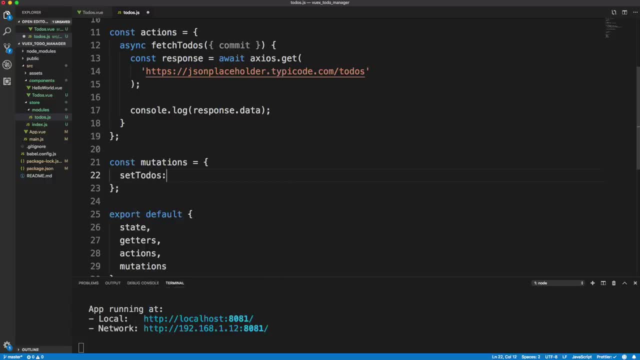 And I'm going to call this set to-dos. All right. 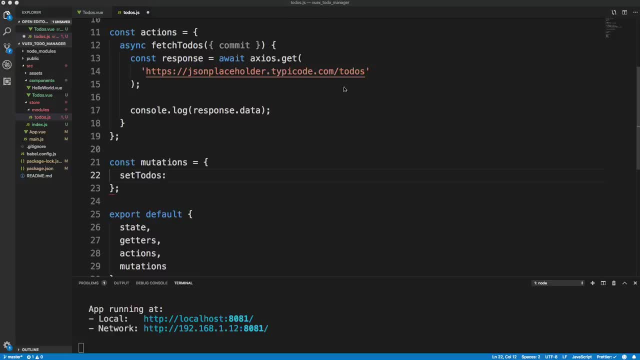 Now this set to-dos is going to take. I want it to take in an array of to-dos, which will be this response. And I want it to add that to the state. OK. 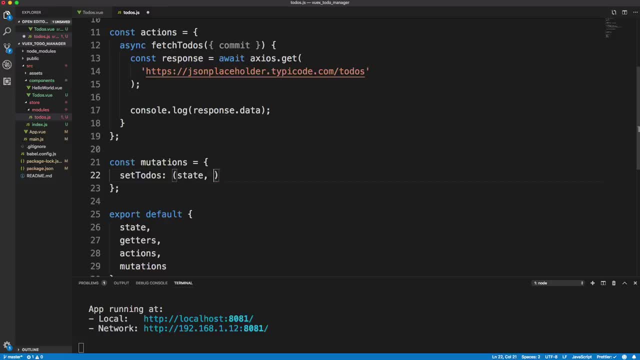 So this is going to be a function that takes in state and to-dos. And what we want it to do, no pun intended, is take the state dot to-dos and set it to the to-dos that are passed in. All right. 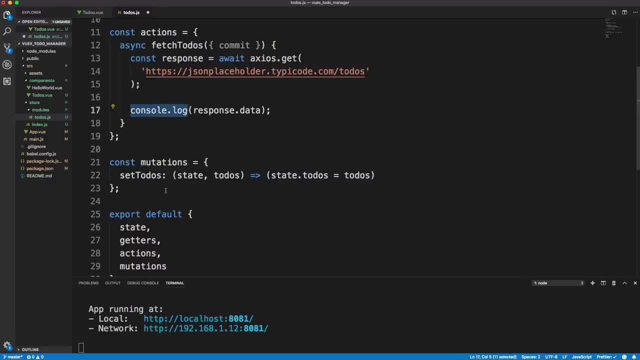 Now up here, in order to call this, we don't simply just do set to-dos or anything like that. 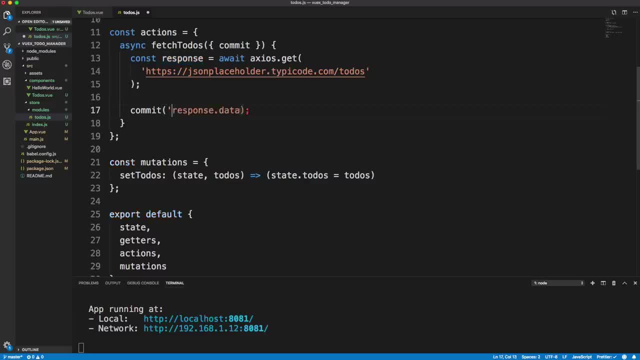 We need to use commit. So we say commit. The first parameter is the mutation we want to call, which in this case is set to-dos. Second parameter is what we want to pass in, which is going to be this. So this is this being passed in. And we're going to set it to our state. And then it should get sent down to the component. So we'll save that. Let's go back. 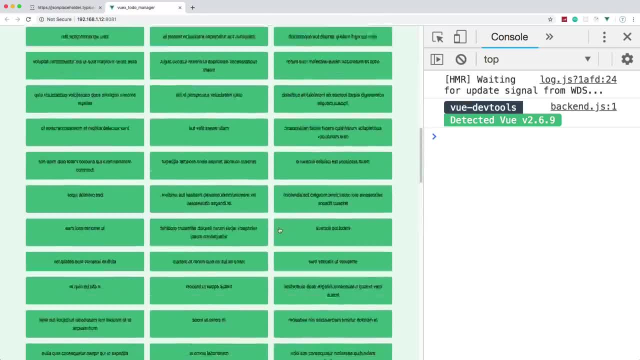 And there we go. We have all of our to-dos in the state that are now showing in the component. 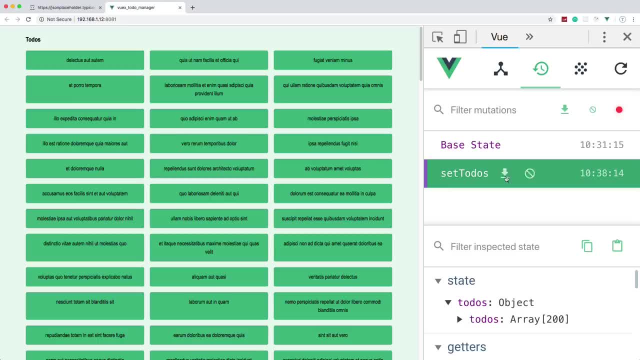 If we go to our View Tools, you'll see that set to-dos was fired off. 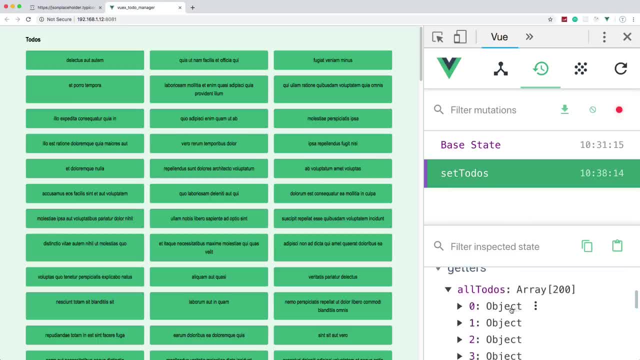 The mutation, we have our state has 200 objects in it, our getters. 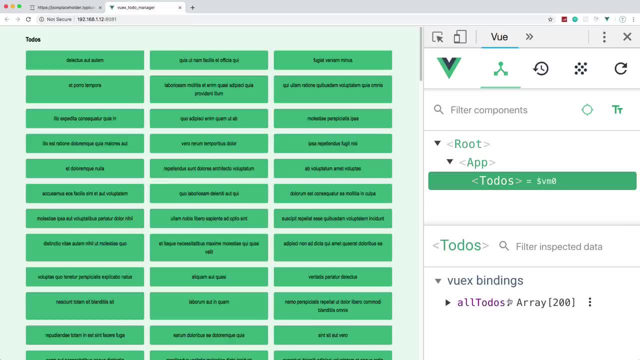 So good. And if we go here, you can see our Vue X binding with the getter. 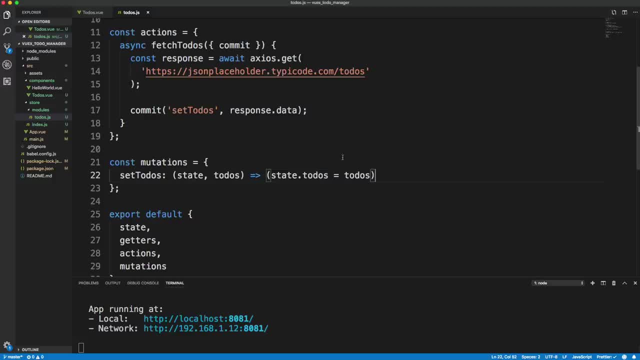 So that takes care of fetching the data. Now I want to be able to add. To add a new to-do. 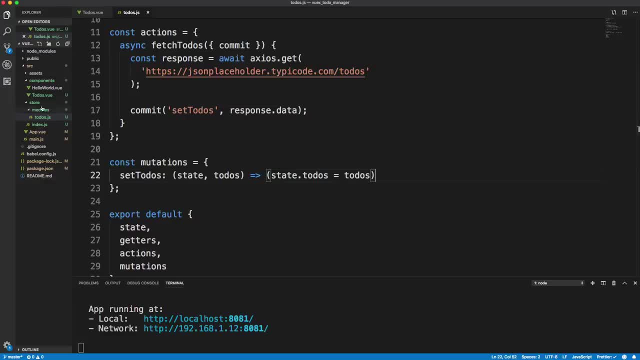 So this is where we start dealing with multiple components. So in components, I'm going to delete this hello world. We don't need that. 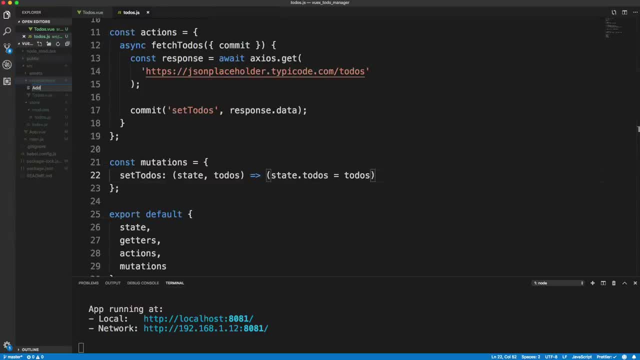 Let's create a new one, new file and components called add to-do.js. OK, so I'm going to just go ahead and scaffold. 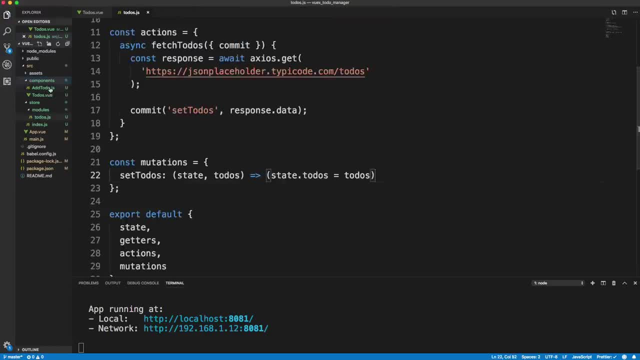 Whoops, I'm sorry. JS, not JS. This should be add to-do.vue. 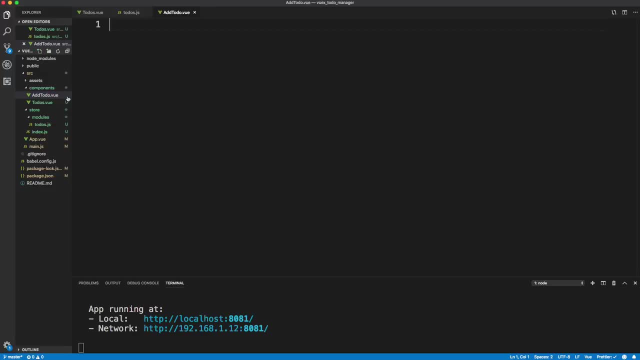 All right, so scaffold. And let's do a div here with an h3. And we'll say add to-do. And then we want to export default name. 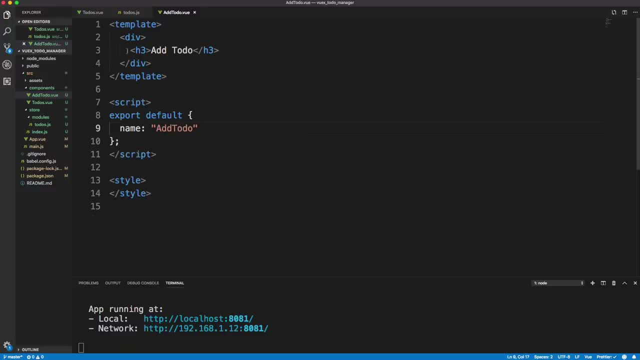 Will be add to-do. Save that. 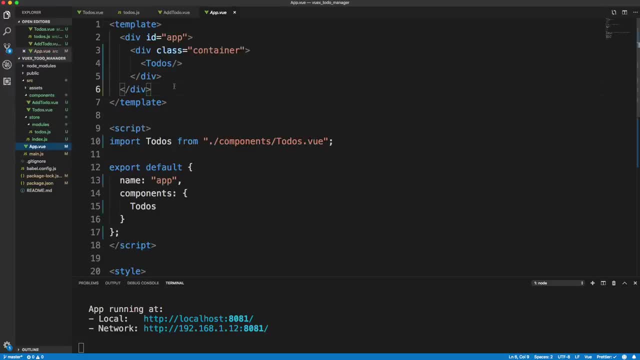 Let's bring it into our main app.vue file, which is right here. So we'll save that. Let's bring it into our main app.vue file, which is right here. So we'll save that. Let's bring it into our main app.vue file, which is right here. So we'll bring in add to-do. 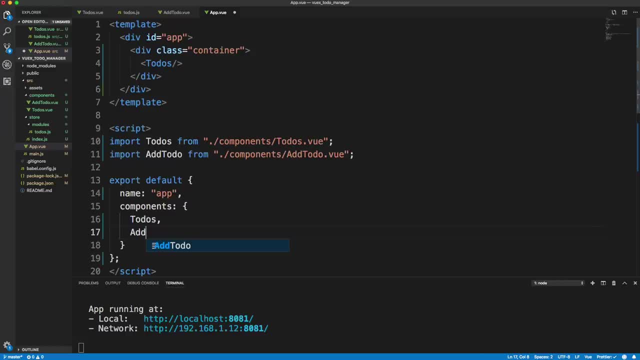 OK, we need to add it to our list of components. 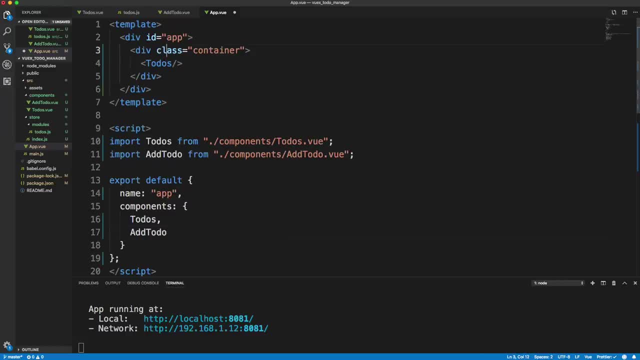 And then let's go up here and let's put it right above the to-dos. So right here. 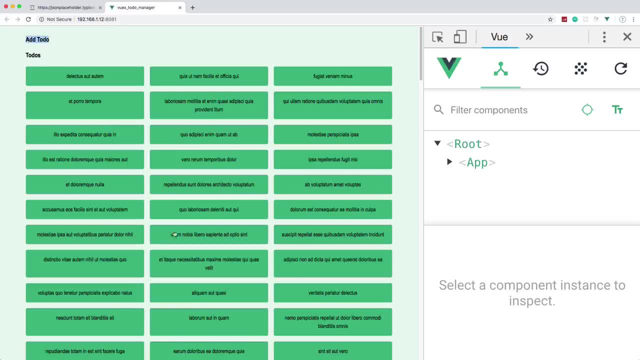 So we'll save that and go back. And you can see that the component is being displayed. 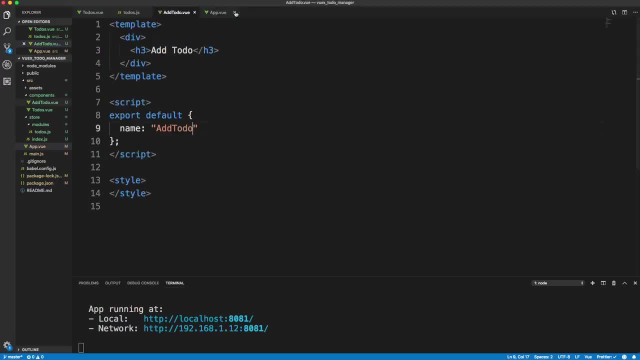 All right, now we're going to want a form. All right, now we're going to want a form. So let's go back to add to-do. And in this component, we're going to create a form right under the h3. Actually, I'm going to put it in a div with the class of add. And then put a form, no action. 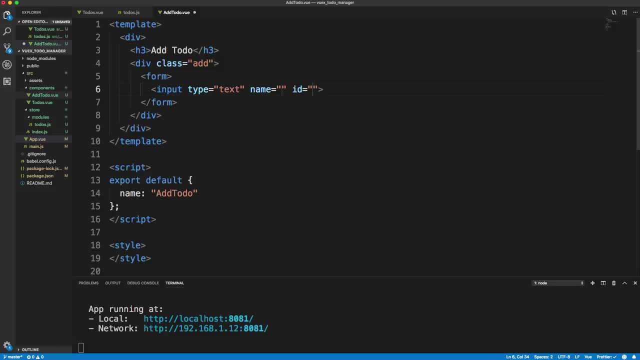 We're going to have an input type of text. Don't need a name and ID. 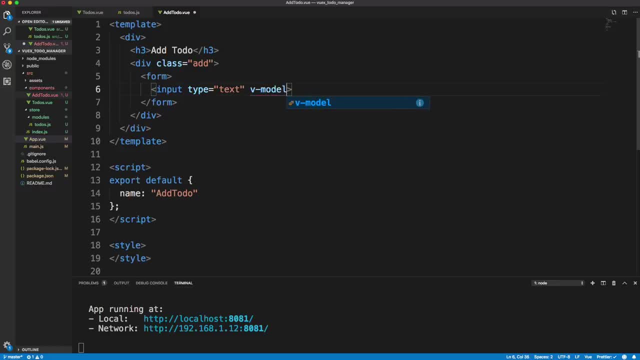 What we do need is a vmodel directive because we're going to bind it to the title. OK, we're going to have. 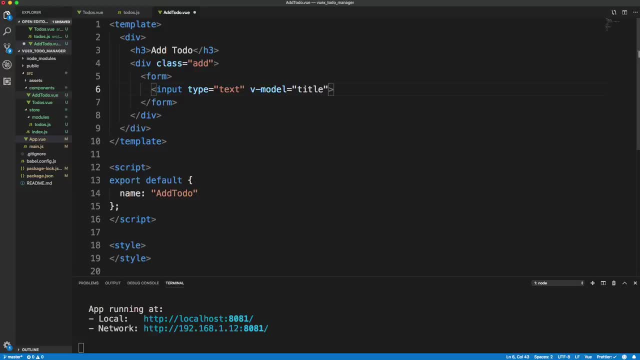 Data in this component called title. And let's add a placeholder that just says add to-do. And then underneath that, we'll have an input with the type of submit, value of submit. And I'm going to just give this a class of. 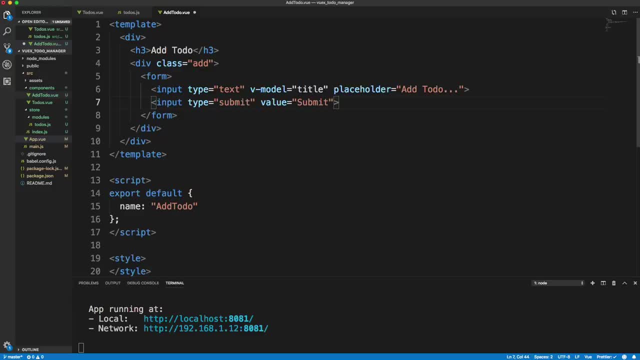 Actually, I don't think we need a class here. No. 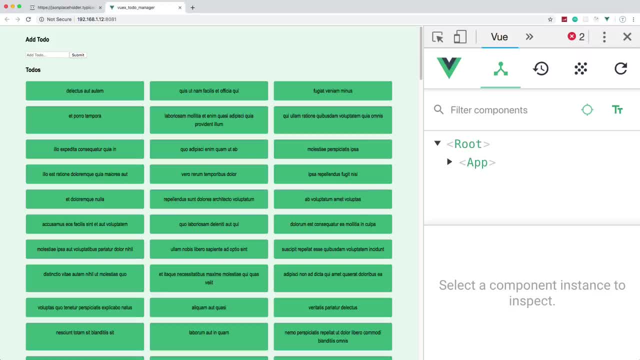 All right, so let's see, we have our form. Let's save that. And it should show up right here. 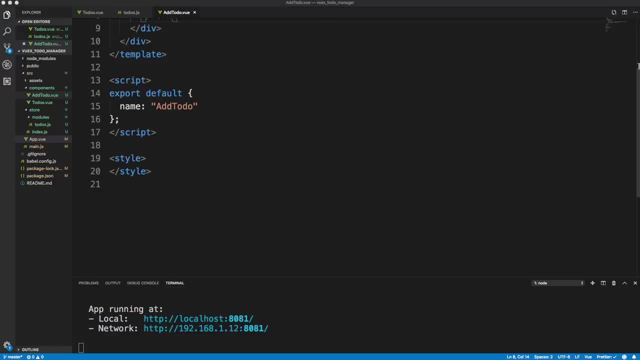 And I'm going to add some styling to this form real quick. 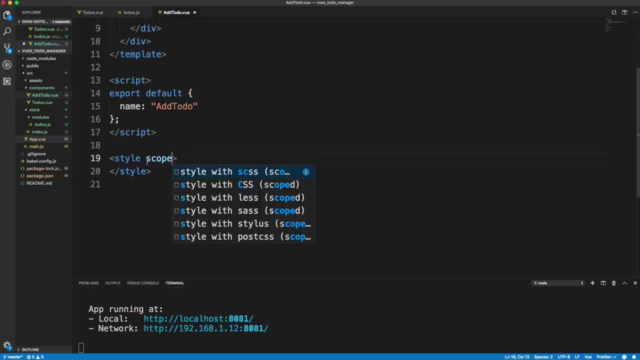 So let me just grab that and say scoped. And I'll paste that in. 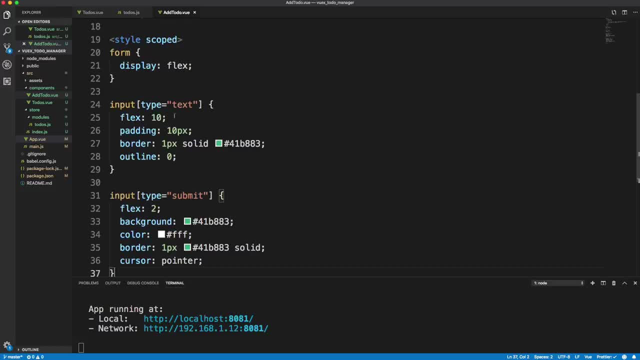 So I'm just using flex on the form and then the the text should be really long. And then the submit button at the end. 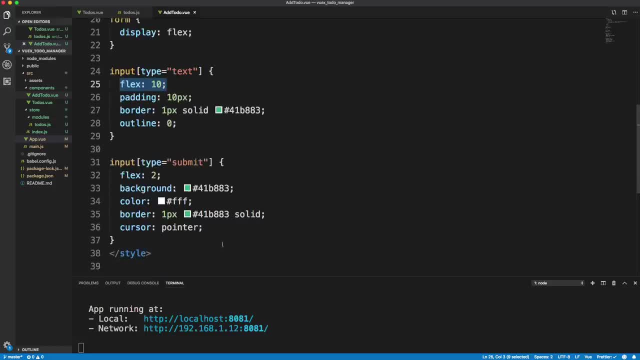 I'm also adding the border, the green border to the button and the text and giving the background. The green background to the button as well. 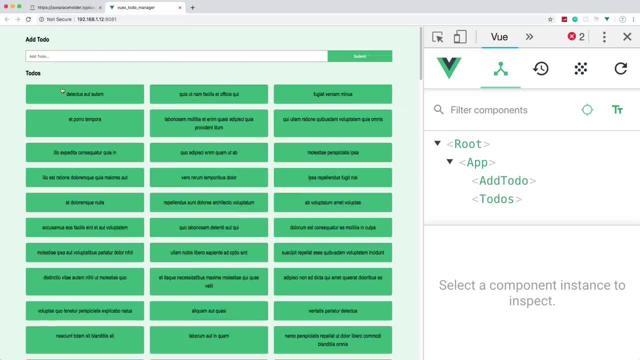 So now if I go back and I reload, you'll see we get a better styled form. All right, now we're going to need to have an action called add to do right when we submit 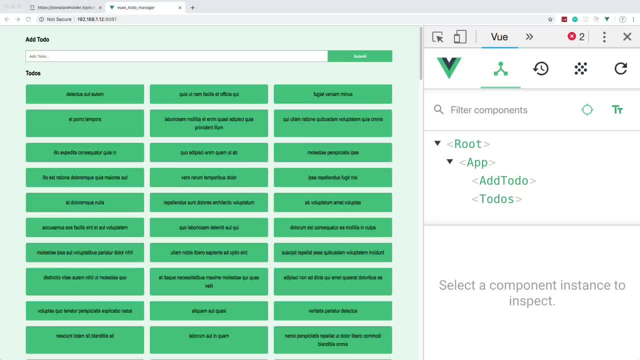 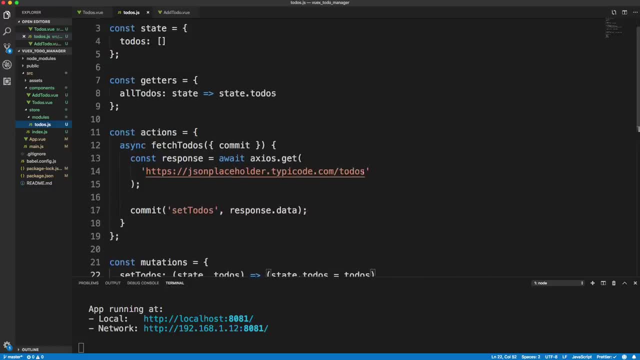 this, we want to call that action. So let's go back into our view X to do's module. So I want to go into store modules to do's dot j s and inside actions, we're going to put another. Method. 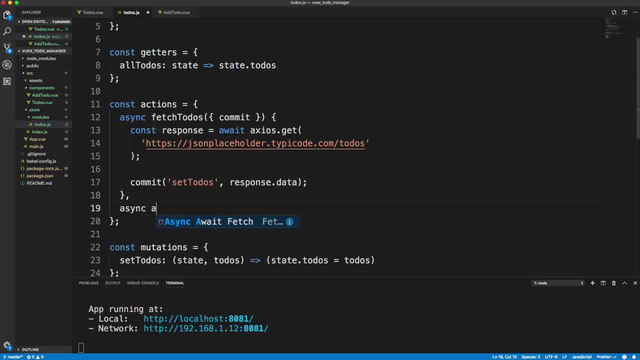 So I'm going to put a comma here and we'll say a sync add to do whoops. So add to do and then this is going to take in an object which we want to destructure and just take out commit. And it's also going to get passed in a title. All right. When we when we create this, it's going to get passed in the title. And then. Inside here, we're going to make a request, a post request to Jason placeholder to send this to do along. 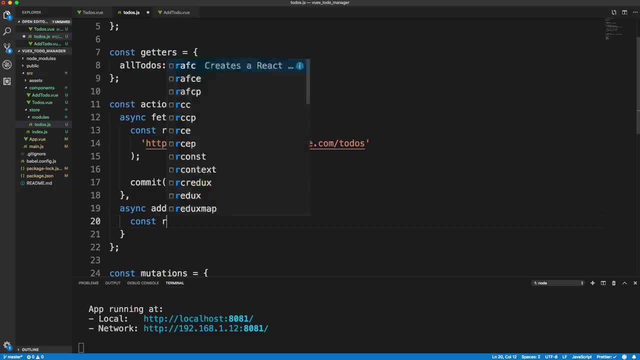 So again, I'm going to be using a sync await. So I'm going to do response equals a weight axios dot post. Okay, now the post request is going to go to the same URL here. So I'm going to just copy that and paste that in. Now. We're going to send along with this. I'm going to send along the title. And then I'm also going to send along the completed value as false, any new to do. It's not going to be completed. 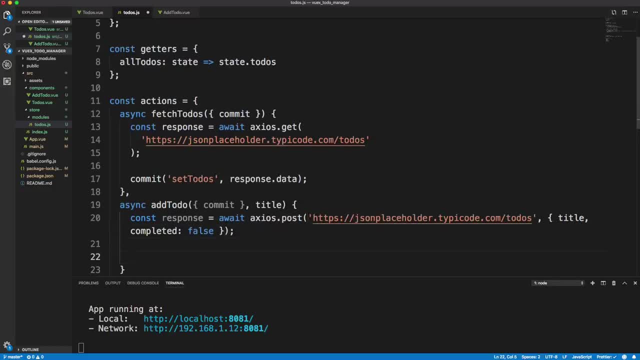 So that's our request. Now once we make that and we get the response back, all I want to do is call a mutation 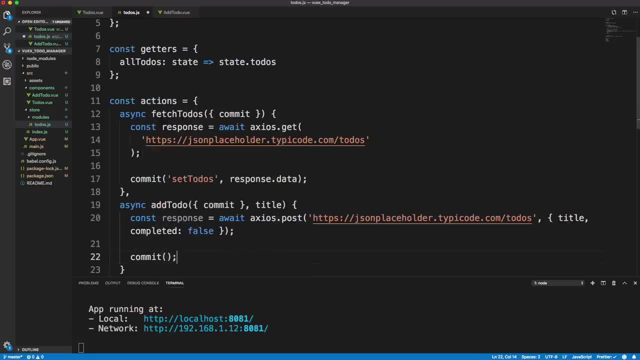 or commit. A mutation. 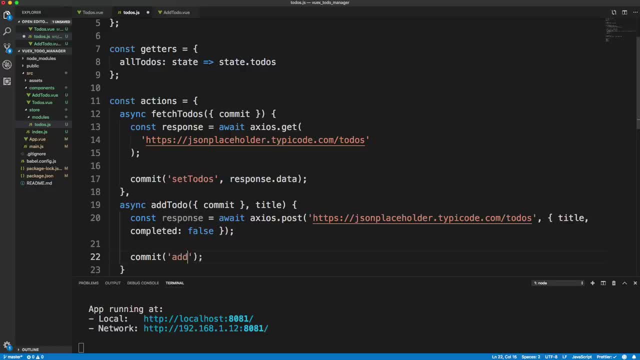 And I'm going to call that, um, add to do right. And then, or let's call it new to do. And then we're going to pass in that response dot data, which will include the new to do. Okay. 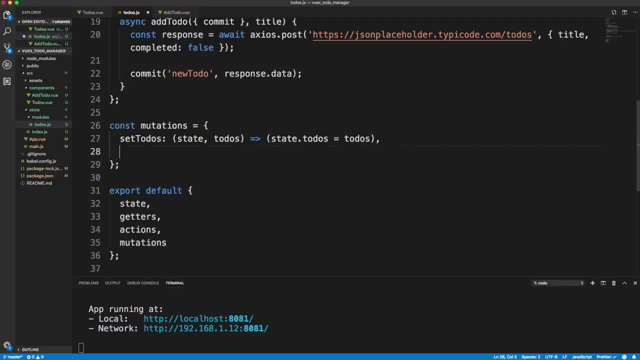 So down here in our mutations, let's put a comma here and let's say new to do. 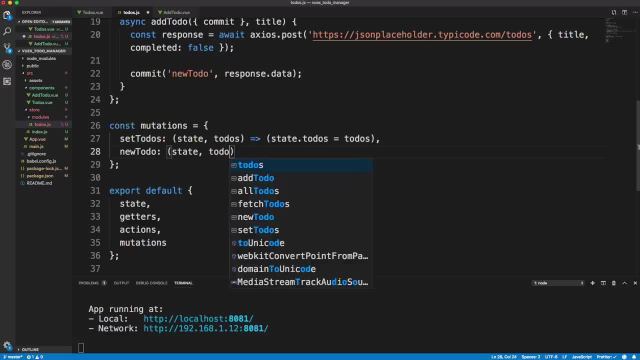 And this will take in state and a single to do. And then to add it, I'm simply going to take the to do's that are in our state and I'm going to, I'm not going to push cause I want it on the beginning. So I'm going to use unshift instead of push and pass on the to do. All right. 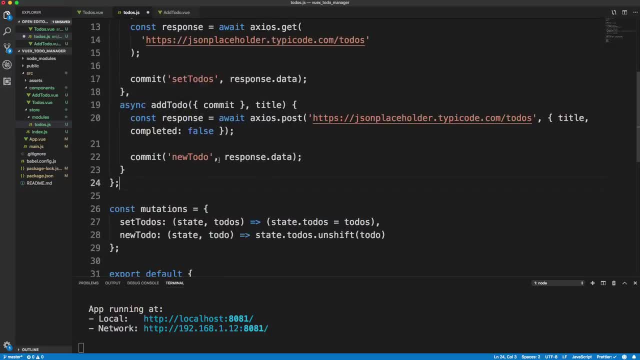 So you can see that the action we're making our requests, getting the data, but then we commit our mutation to actually mutate the state. 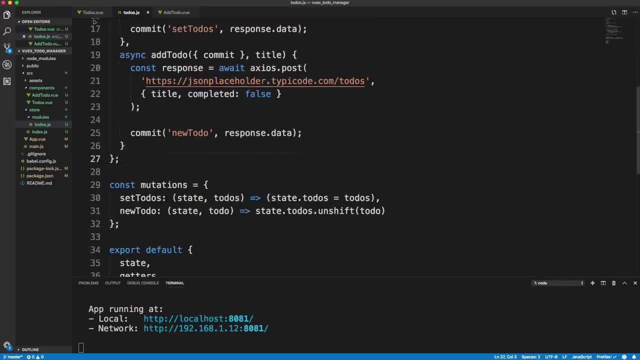 So let's save that. And let's go back to our ad to do. 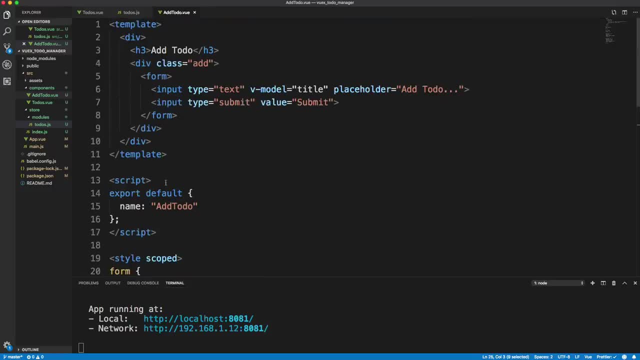 Okay. So let's go back to our component and we want to be able to call that action. 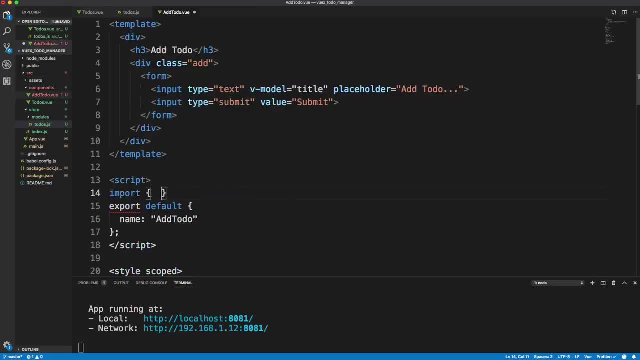 So in the script here, we're going to import map actions from view X. Okay. Just like we did in the other component and to use map actions, we want to add in methods and I believe it's the only, no, we're going to have an on submit. So, um, we're just going to add the spread operator here. And then map actions and the action we want is add to do all right. So this form here, we want to add a submit event. 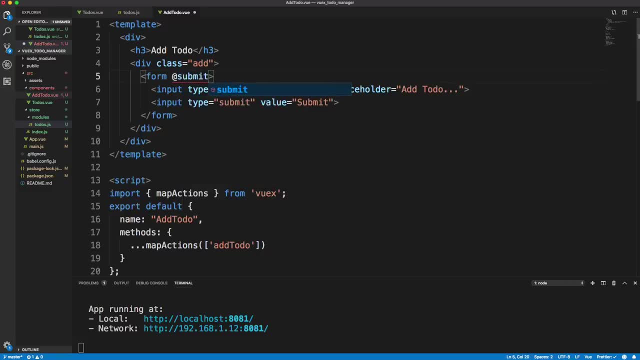 So let's say, um, at submit, we want to call on submit. 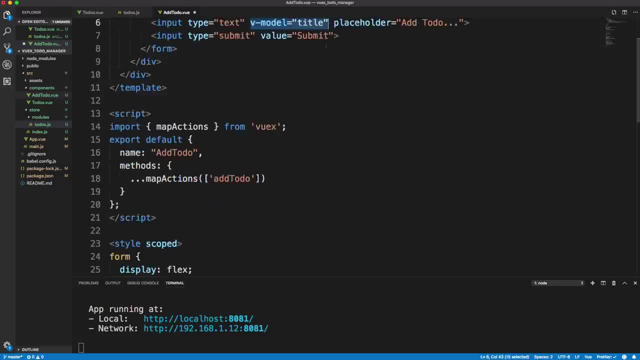 Now one thing I forgot is with this V model title. Okay. 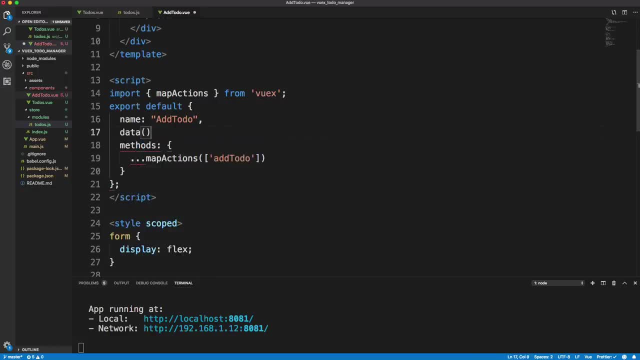 We want to add a data method here that will return an object that has that titles. So we want to return and just say title, which will start just empty. All right. 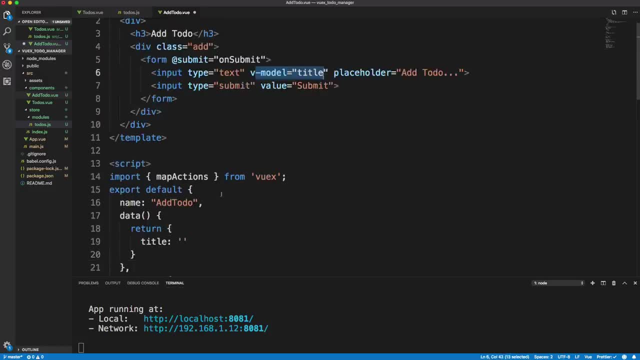 So whenever you have a V model like this with a property, you want to add that to your data in the component, which has nothing to do with view X. That's just few JS. All right. So we have this on submit. Okay. 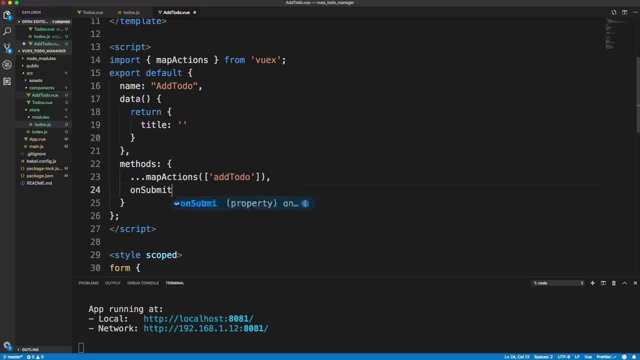 So we're going to add that to our methods down here. Let's say on submit takes in an event parameter and sentences to submit. Since it's a submit, we want to call prevent default so that it doesn't actually submit to the file. 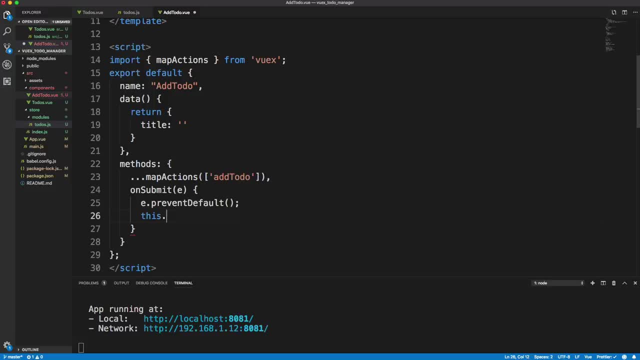 And then we just simply need to call our add to do actions. So we do that with this dot add to do. 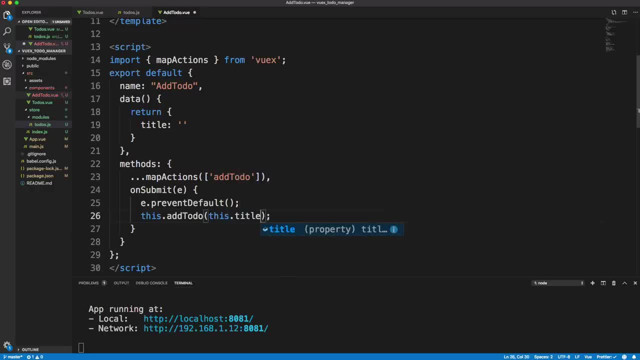 And remember we're passing in a title so we can access it with this dot title since it's part of the data of this component. So let's save that. 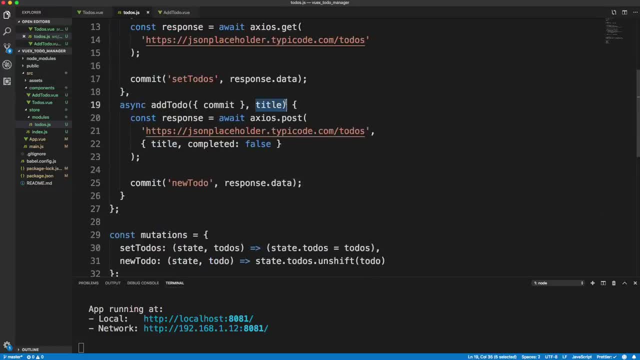 So this dot title will get passed in right here. We'll make the response. I'm sorry. We'll make the request. 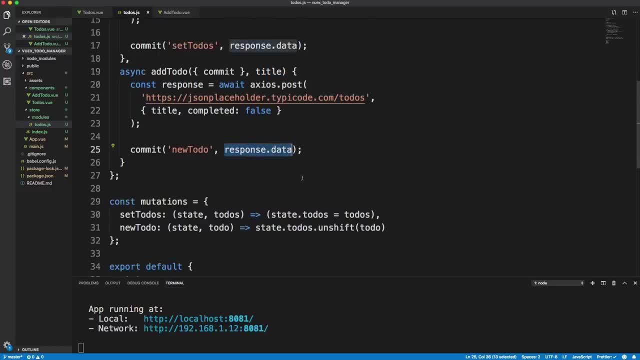 We'll get the response, which will include the whole new to do, which we commit to the new to do mutation. All right. So let's try it out. 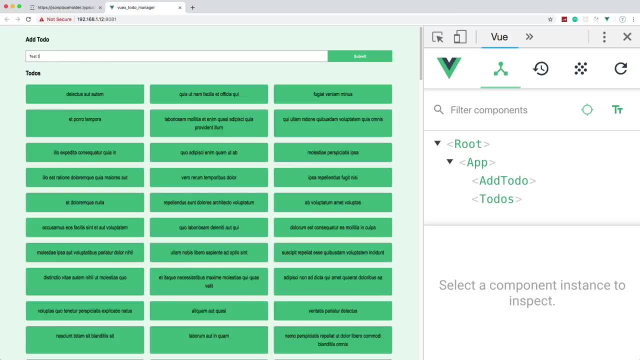 We may have an error, hopefully not, but we'll say test to do and submit and there it is gets added. Okay. 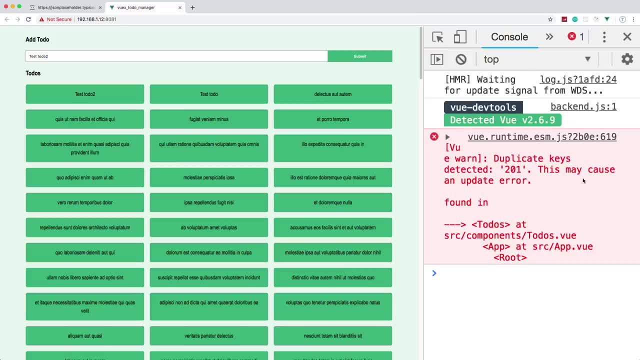 Now one thing you'll notice with Jason placeholder is if we look in the console, we get this duplicate keys because whenever you add a new value, it's always going to have the same ID. 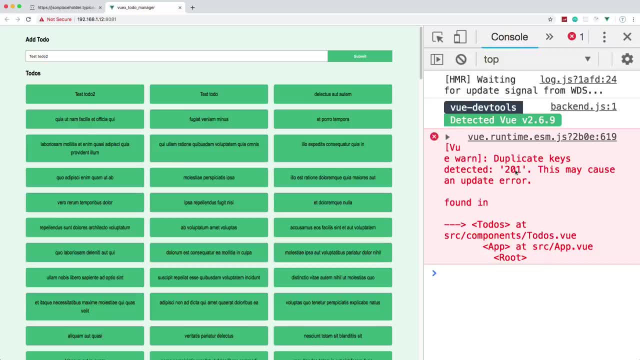 All right. Because it doesn't allow you to actually add to the database and persist and then have 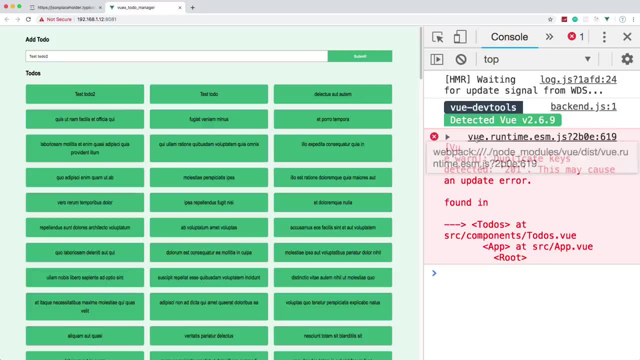 another ID and another ID. It's just for testing. 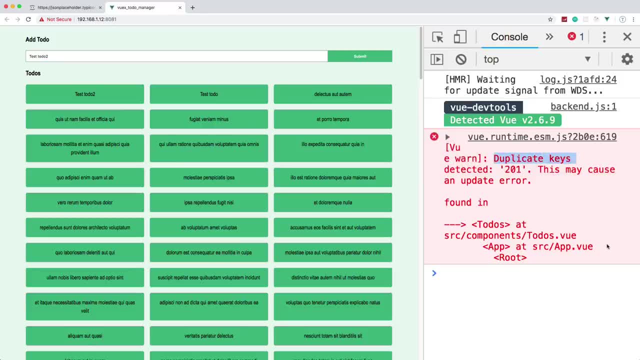 So this is just telling us that we have duplicate keys. So basically. All of these have the same key because they have the same ID, but if it was a real backend, you wouldn't have that issue. Okay. 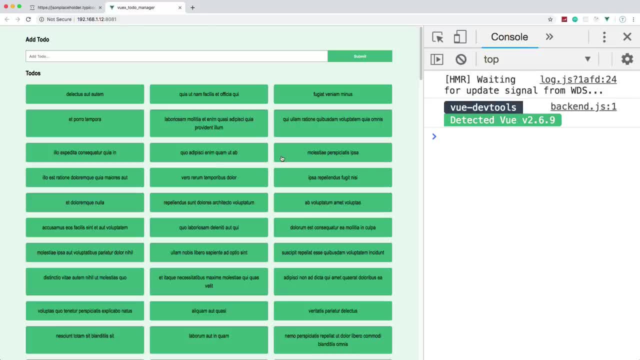 Just like if I reload, it goes away because obviously Jason placeholder isn't going to allow just anybody to, um, update their database. All right. 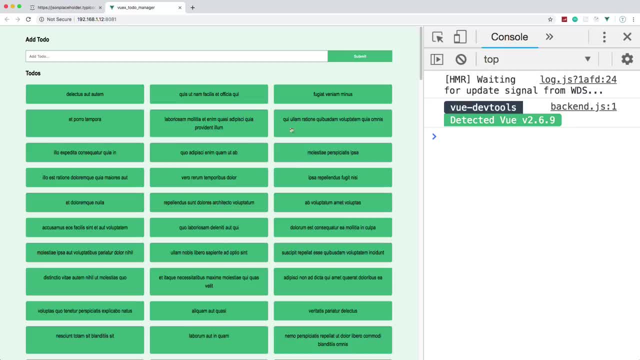 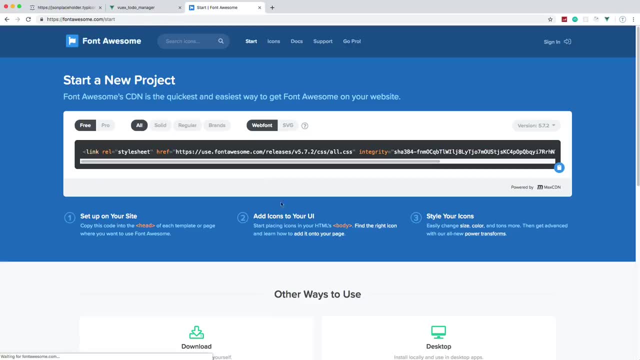 So now what I want to do is delete, I want to be able to delete these and I'm going to add an icon. So I'm just going to go to font. Awesome. And click start using free. We'll grab the link. 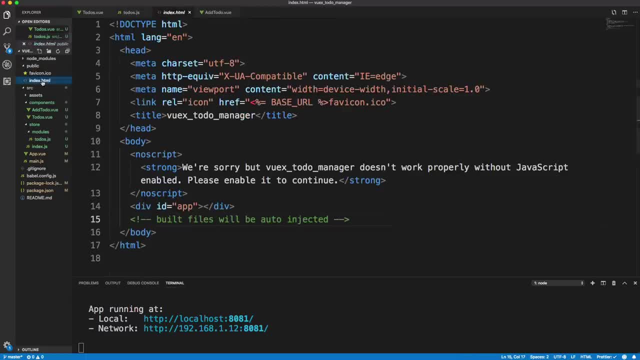 Click here. Let's put that in our public index HTML. 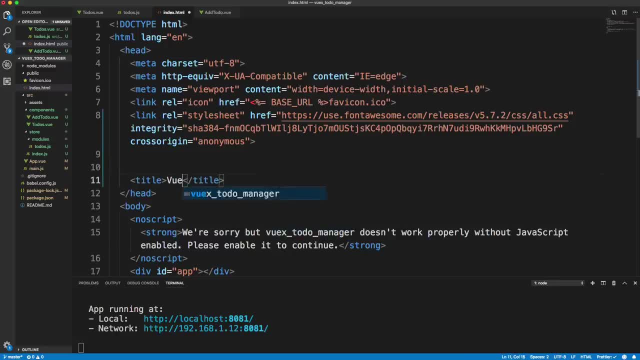 And I'm also going to just change this title, say view X to do manager and save. 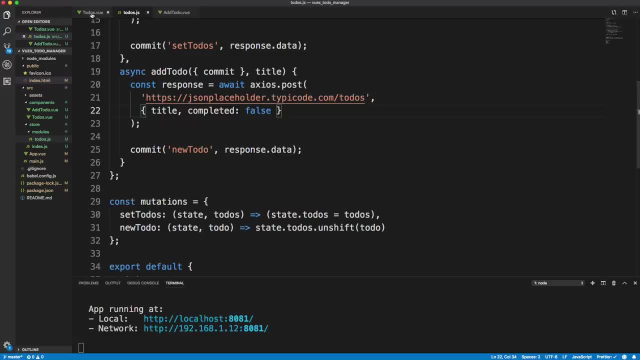 Okay. So now we have font. Awesome. So that we can use icons. 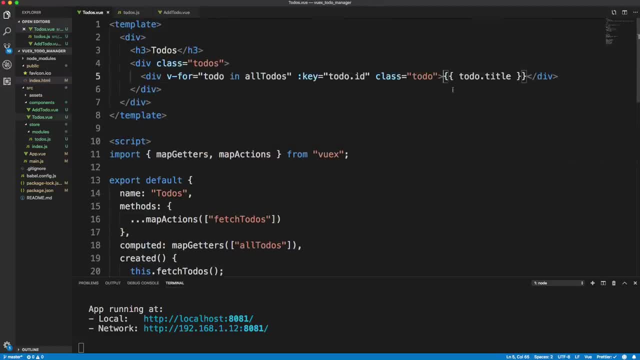 Let's go into our to do's dot view. We're going to go right under the title and let's do, um, some reason I can't use Ms. 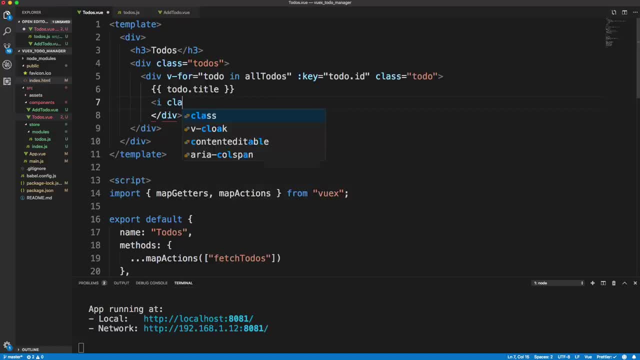 So I'm going to say, I'm going to do I class and class is going to be F a S and then F a dash. I think it's trash dash. Alt. Let's try that out. Yep. 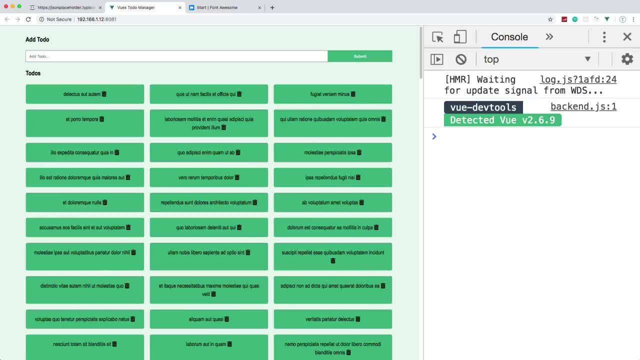 So we have this trash can. Now I want this to be in the bottom corner, so I'm going to add a little bit of styling down here. Uh, let me just find it real quick. Okay. 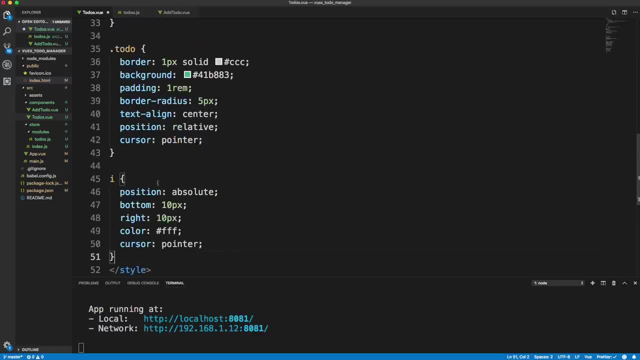 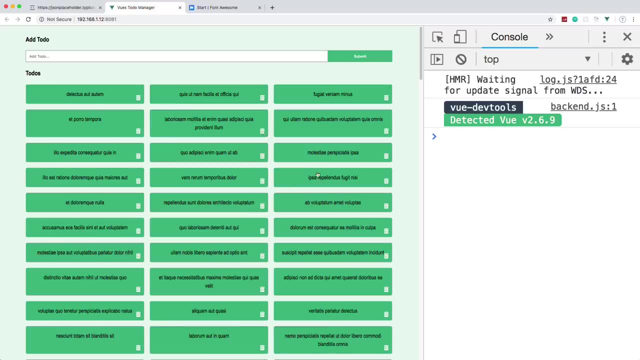 So we're just positioning an absolute bottom, right? Also adding a pointer to it and now it should look like that. 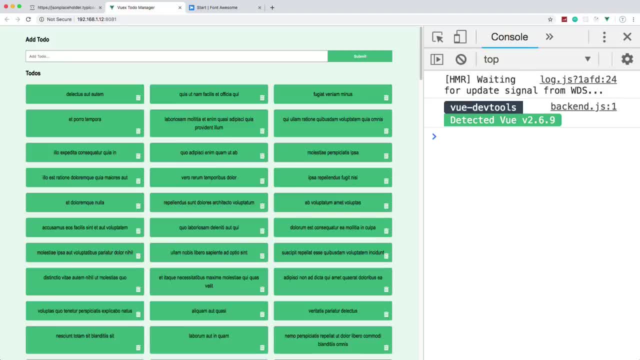 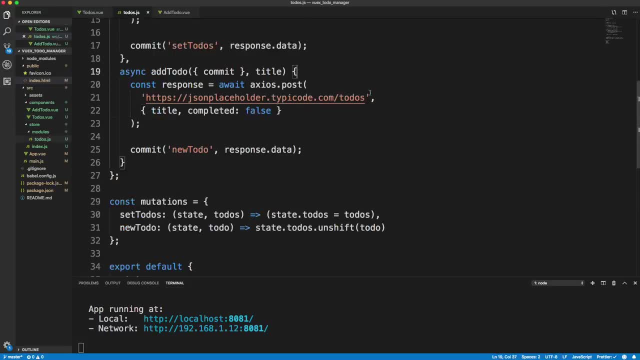 So we need to have an action now to delete a pop, not a post, a to do. So let's create that in our, our module. So we have fetch to do's add to do. So under add to do, we're going to do a sink. Delete to do all right. 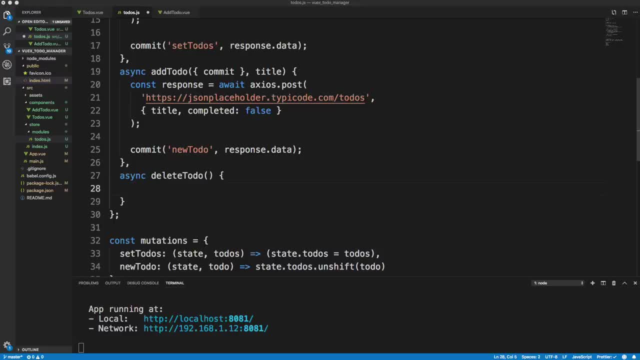 And this, uh, this delete to do is going to have, is going to take in an object we want to take out commit and it's going to need to know which I, which to do it's deleting. 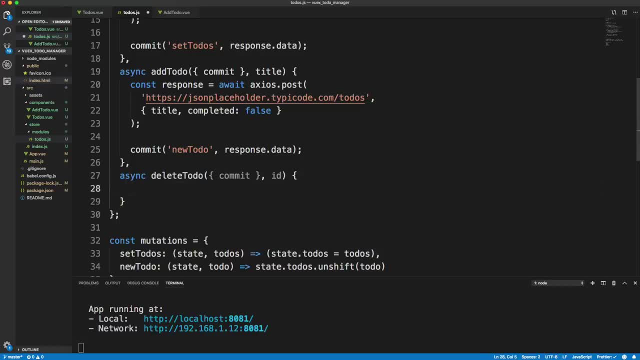 So we're also going to pass an ID in when we call it and then, uh, we're going to make our request. 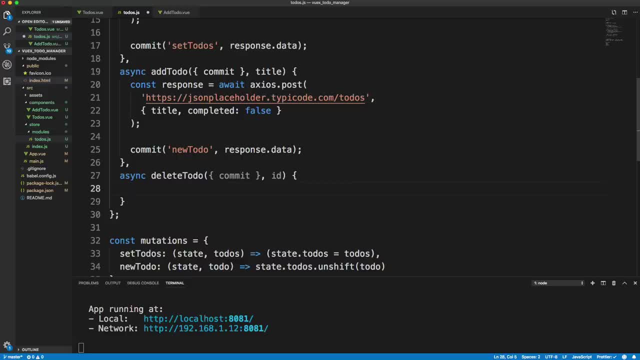 Now I don't have to store the response cause I'm, all I'm doing is, is I'm just going to call remove to do with the ID, I'm going to have a mutation for remove to do. 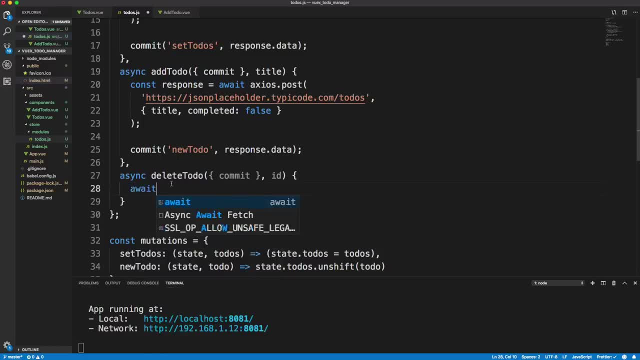 Um, so we don't actually need to put the response in a variable. So I'll just say a weight Axios dot, and then we're making a delete request and the delete request is going to go to this URL, but I'm actually going to put back ticks in here because I'm putting the URL slash and then the ID. So I want to go like that. 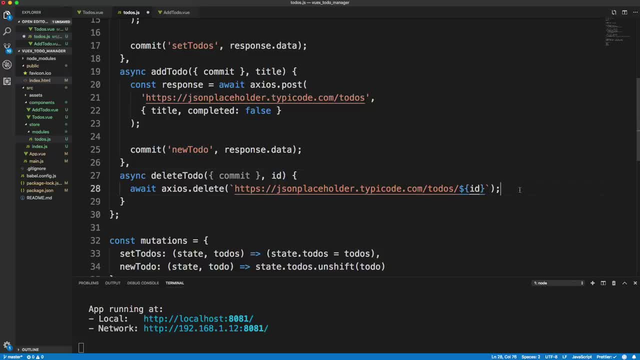 The ID is getting passed in here. Okay. So that deletes it from the server. 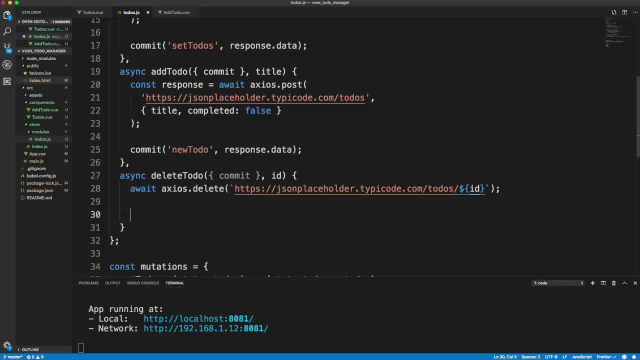 Hypothetically, it doesn't actually delete it like from the database, um, with Jason placeholder, but then we're going to want to commit a mutation. 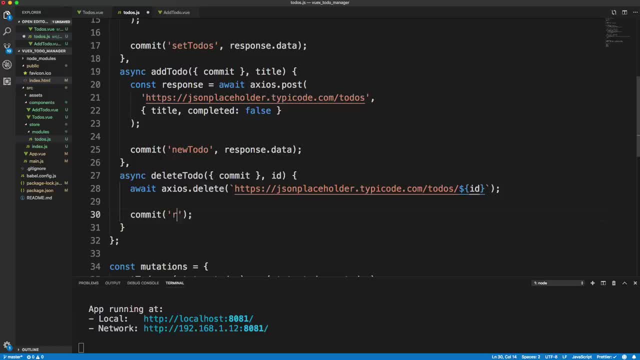 So this is going to be, um, remove to do, and we need to pass in the ID. Okay. So let's go down here. Yeah. 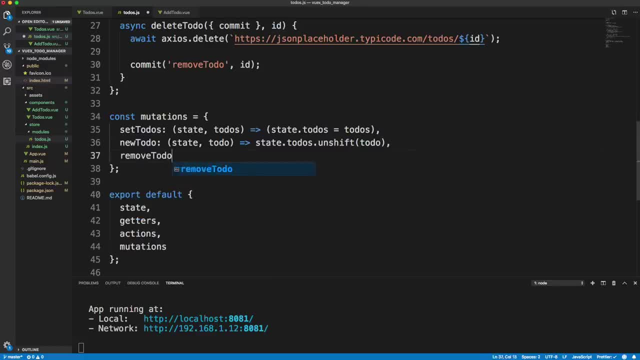 We're going to add in remove to do, okay, which is going to take in state and the ID. And I mean, you could do multiple things here. I'm going to use filter. So I'm just going to set the state dot to do's equal to state dot to do's dot filter. And we'll say for each to do, we want to return where the to do. ID is not equal to the ID that's passed in. So that will remove it from the UI. All right. 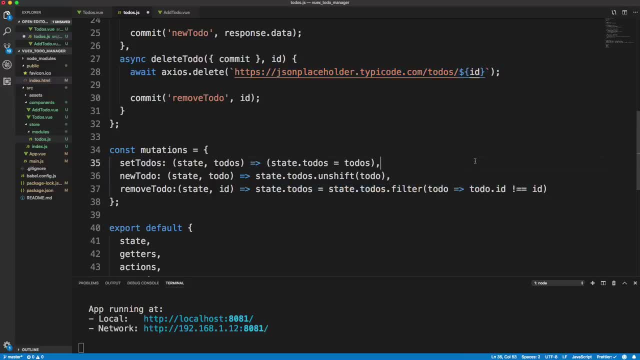 So this will remove it from the backend and this will remove it from the UI. So we'll save. Now we need to call this action. Okay. 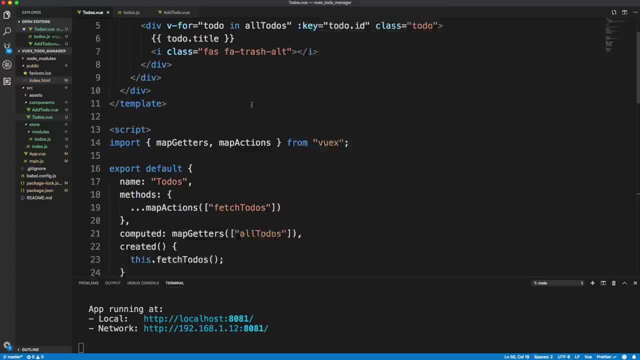 And where we want to call it from is our to do's component. Okay. We want, when we click this, this icon here, um, that's when we want this to happen. So. 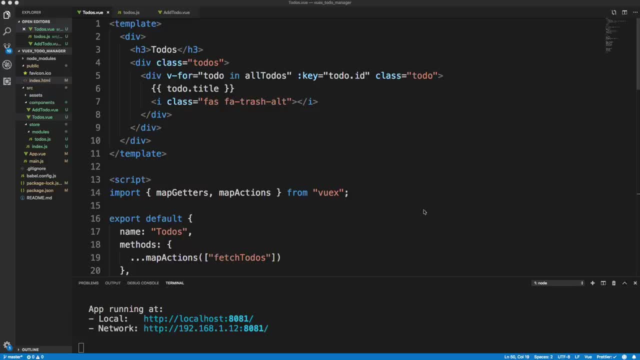 Let's add, uh, yeah, let's add a click event here. 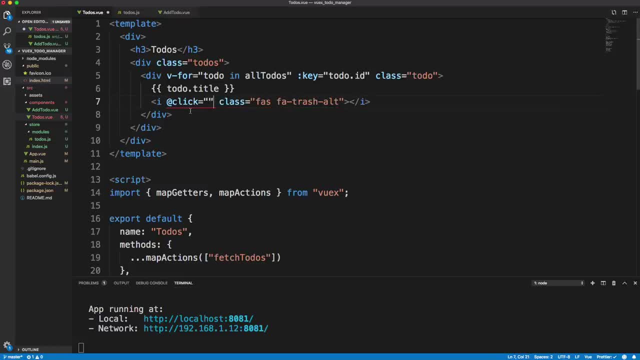 Okay. So when we click this icon, I'm going to call delete to do, and I'm going to pass in the to do dot ID. 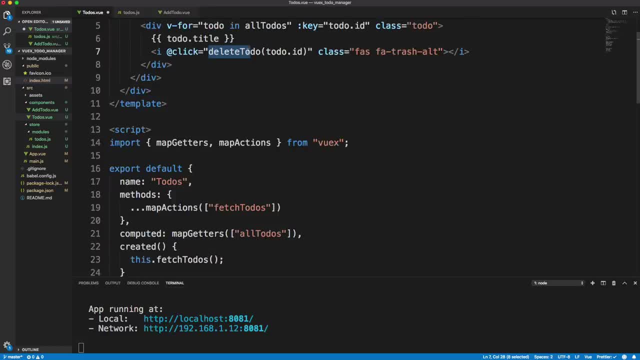 Now this delete to do, I'm actually going to, I'm going to call the action directly right here. 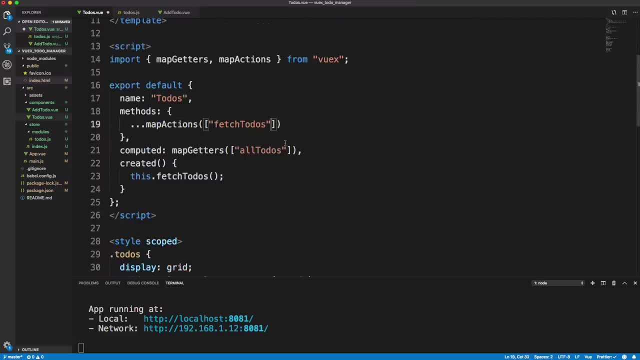 I'm not going to create a delete to do down here. I'm going to bring it in right here. So. Let's say we want to catch to do's. 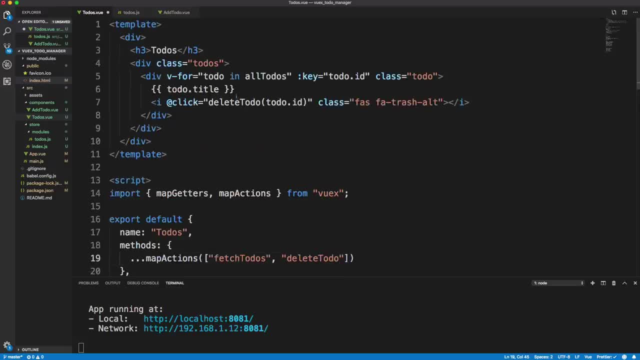 We want to bring in the delete to do action. And that's what I'm calling right here. All right. 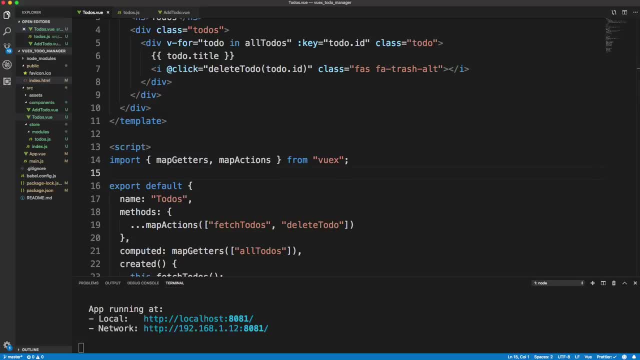 So let's go ahead and save that. Let's see if that works. And if I click one of these, there we go. They get deleted. 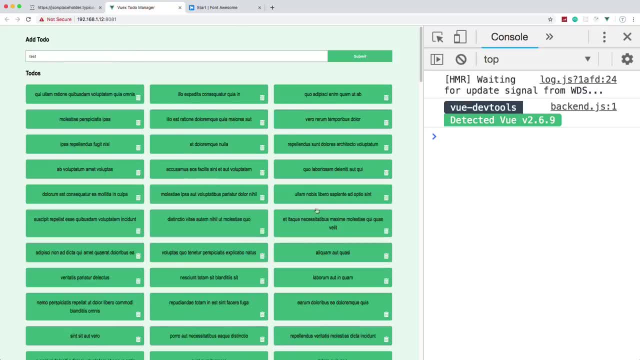 So if I add one, we'll say test that gets added and I can delete it. Good. So the next thing I want to do is filter. Okay. 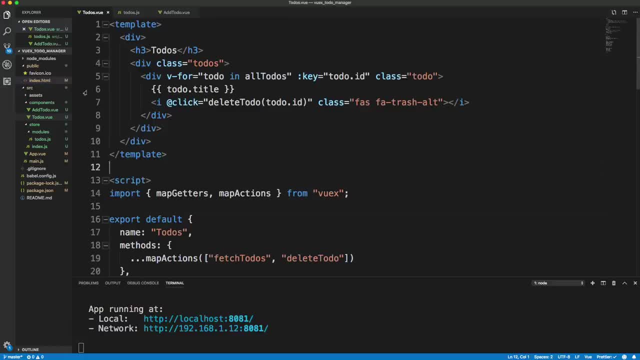 So we're actually going to have a separate component for that. And it's easy to add as many components as you want. 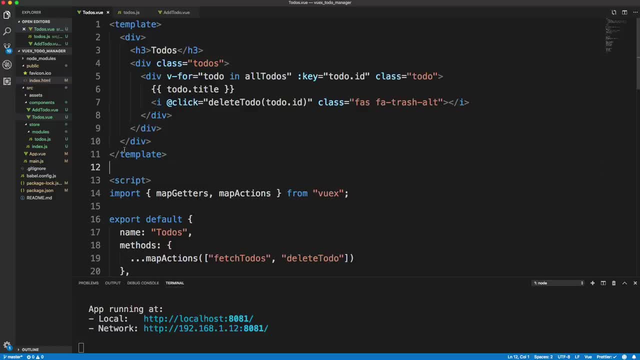 And you use the same state because we're using a state management library. If we were to use, if we were not to use Vue X, we would have to emit events to pass things up and props to pass things down and it gets, it gets tricky and it gets really annoying. 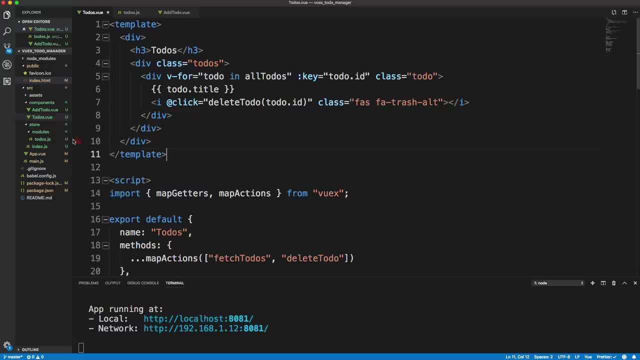 So you know, Redux, Vue X, these state managers really help. So let's create a new component. 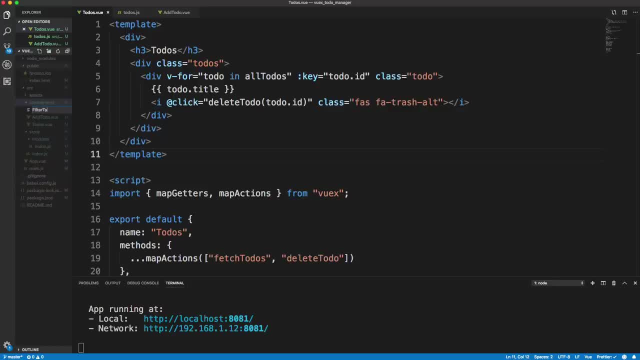 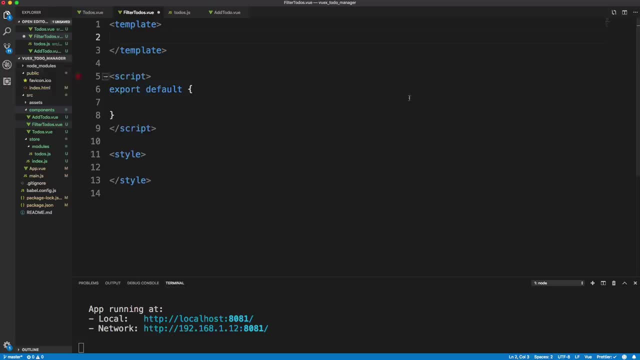 I'm going to call this filter to do's dot view. And we'll do our scaffold. Okay. So as far as the, um, as far as the template goes, I'm going to put in a div and I'm just going to say filter to do's and let's put in a select. We don't actually need, uh, this stuff here. Let's get rid of this. Okay. Okay. 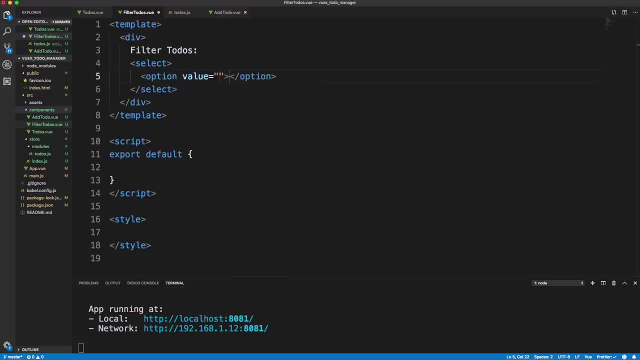 And we're going to do option. So value, let's do, I guess it's 200. I thought it was 100, but, um, I guess it's 200. So we'll do 200 whoops. That's the default. Uh, and then let's do one, two, three, four, five, I think. So we'll do 200, 100. Let's do a 50. Okay. 20, 10 and five. Okay. 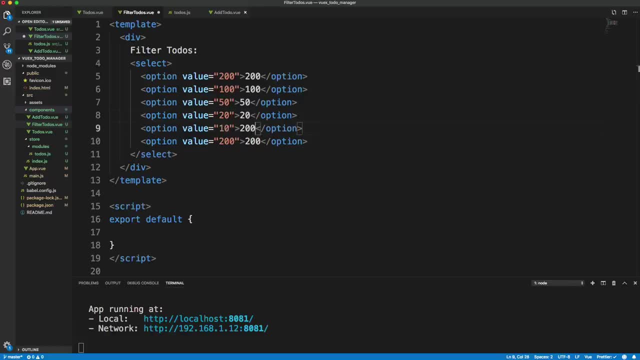 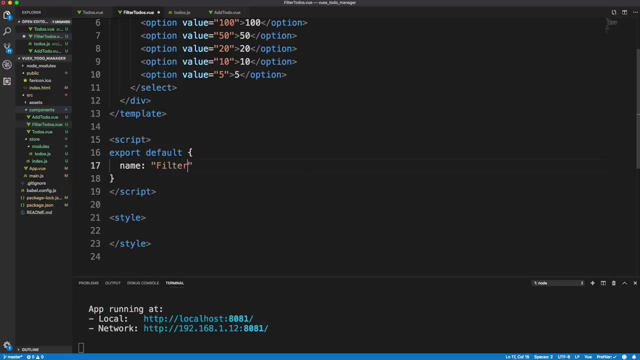 So that's our select list. So let's see, we have to put a name for this, which is filter to do's. 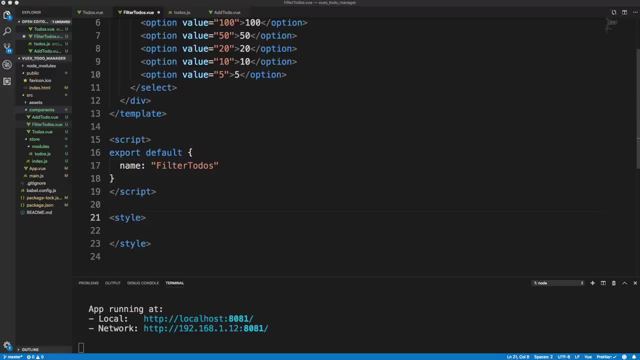 Um, and then I'm just going to put a little bit of styling in here just for the select, which doesn't seem to even work on Mac, but I'll put it anyway. All right. 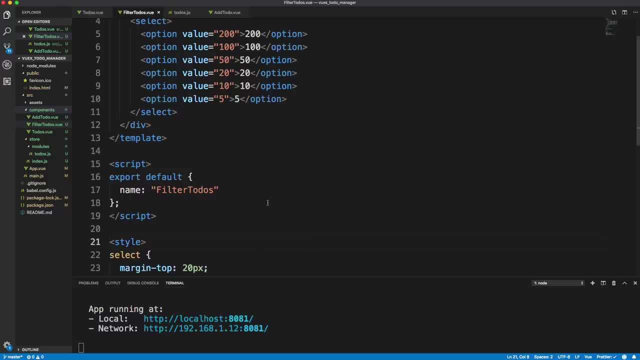 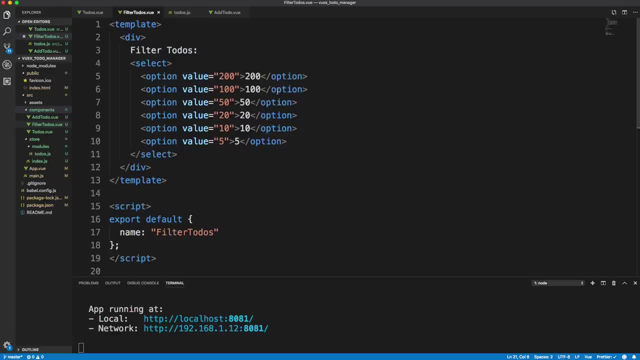 And then all we need to, all we need to do here is on when this changes, we want to call an action called filter to do's. Okay. But I'll implement that after we actually create it. 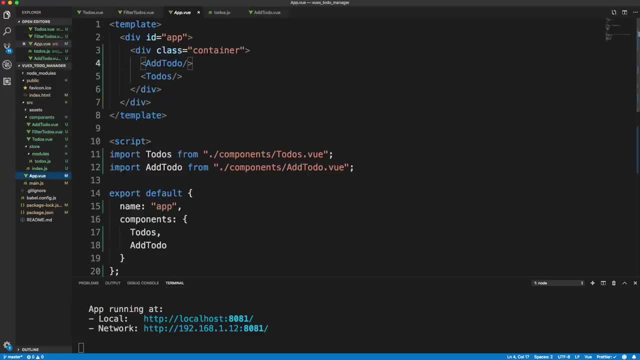 So for now, let's just bring this into our main app dot view. So we want to bring in a filter. Okay. Filter to do's and we're going to add this down here to our list and we want to go up here and put this right in the middle of the other two. 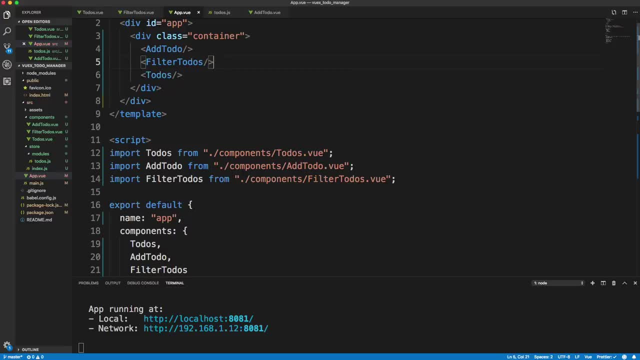 All right, let's save that. See if it shows up. 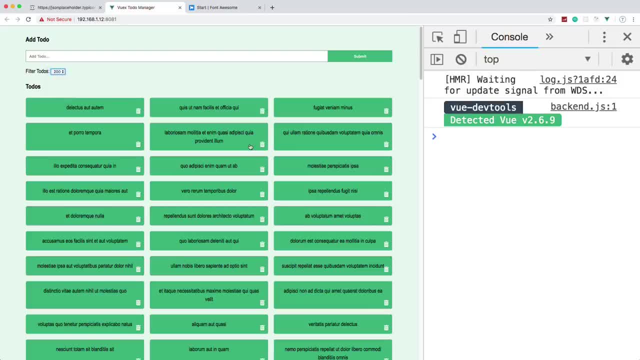 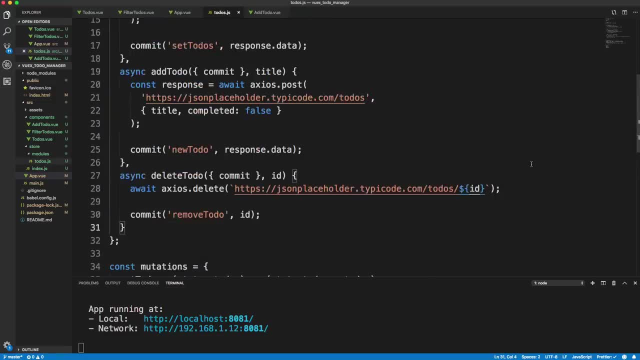 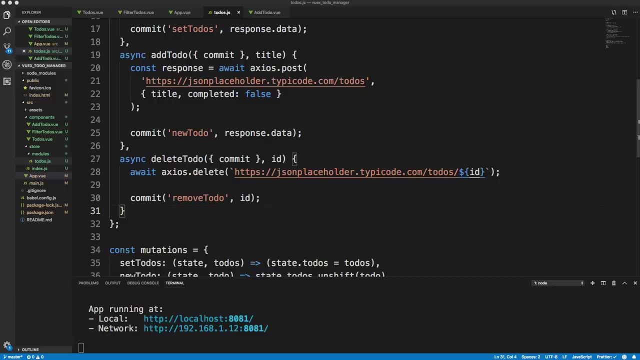 So there's our little dropdown select list, wherever the hell it is. And we're going to go back to our module now, our to do's module, and we're going to have another, um, uh, action to filter the to do's. Okay. 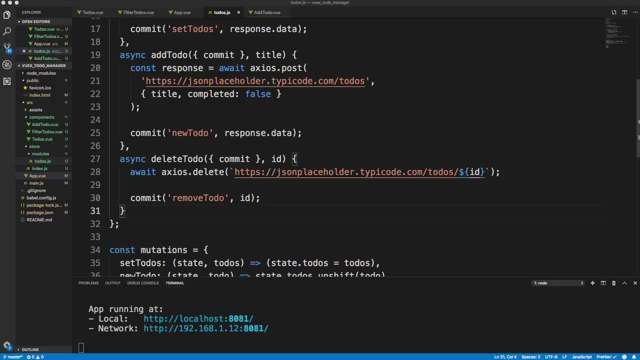 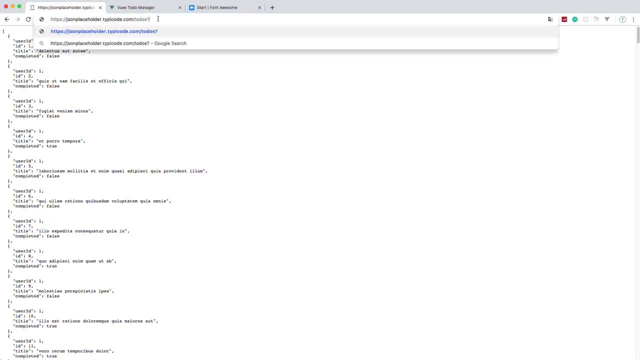 So let's go ahead and let me just explain how we're going to do this. You can limit the resources from Jason placeholder simply by putting in a query string. If I do question mark underscore limit equals five and I run that, it only gives me five to do's. So while we're going to, all it's going to happen here is we're going to just make another request with this limit, a parameter, all right, each time we change that select. 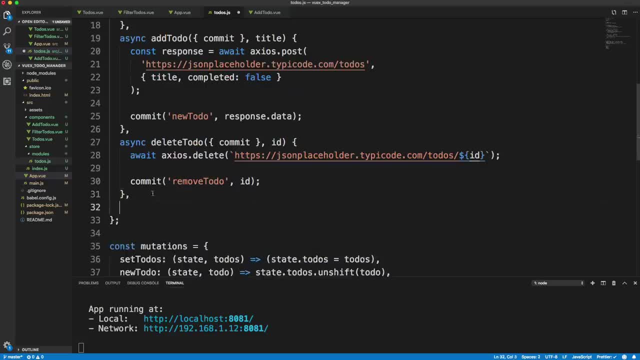 So right here, actually let's put a comma and let's say a sink and let's call this filter to do's. Okay. 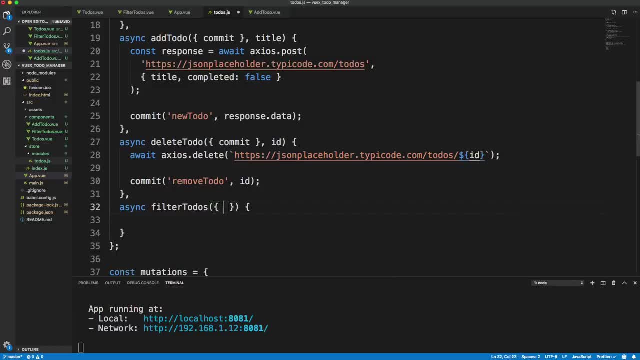 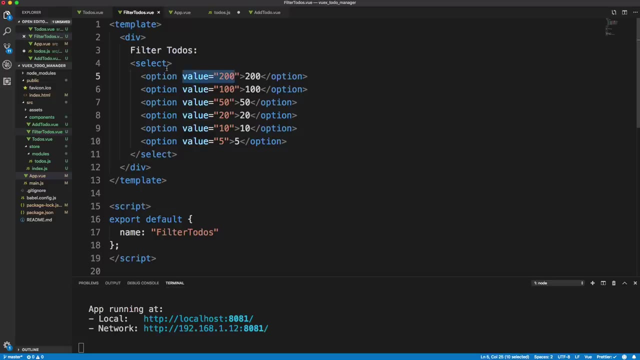 So we're going to want to commit a mutation. So we need to bring in commit, uh, let's see, we're also going to pass in the event parameter because we need to, we need to be able to get this value here from the select list. Okay. 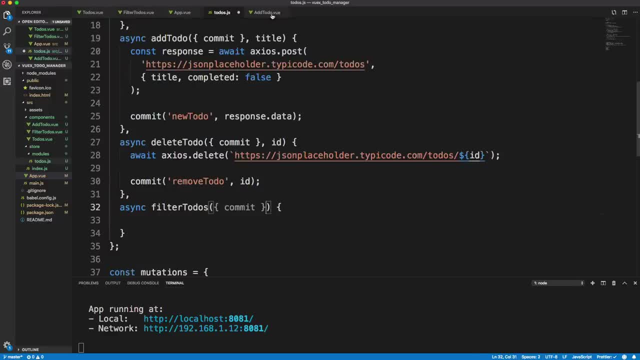 So I'm going to show you how we can do that. Um, where are we? Let's close that up. 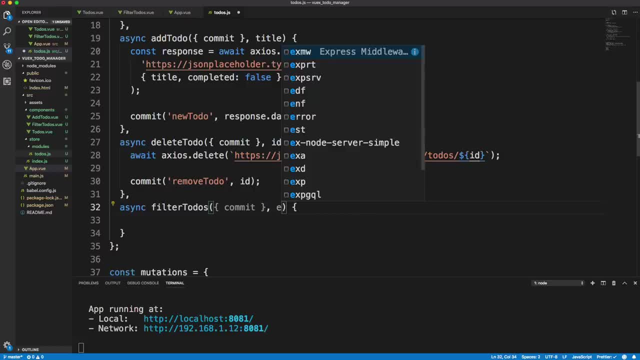 So we're going to pass in an event parameter here. Um. 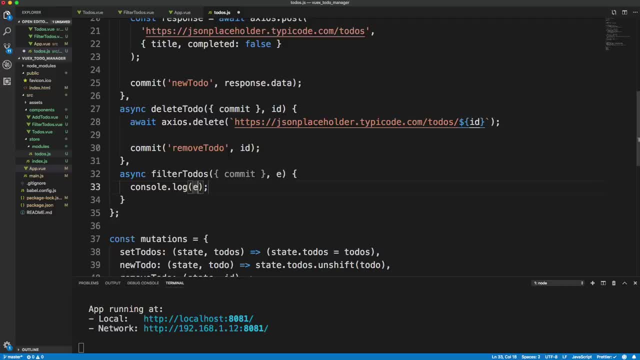 And I guess for right now I'm just going to console log that event parameter. I'm not going to do anything else. So we just have an action that will console log the event that's passed in. 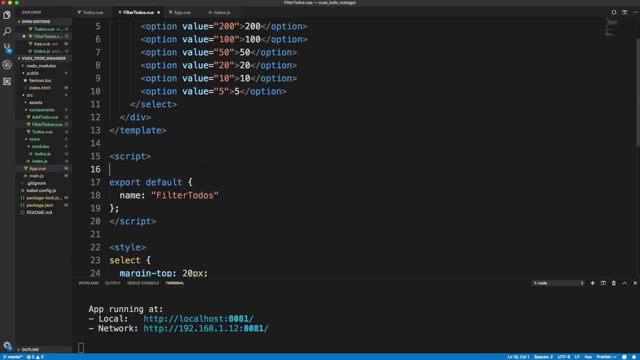 So let's go back to filter and in order to use that action, of course we need to import map actions. So hopefully this, this repetitiveness is, is really drilling it into your head, how to bring in actions and getters and use them. 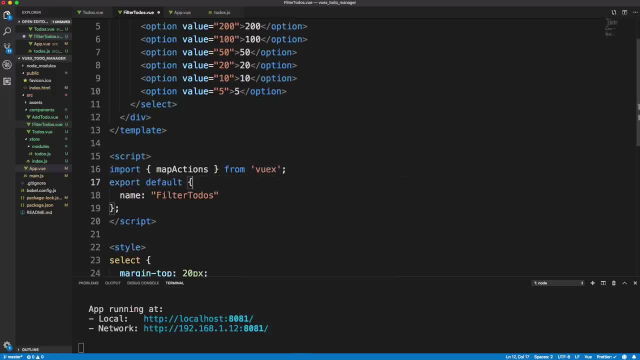 Um, so this is from view X. And let's see. Okay. Let's see. 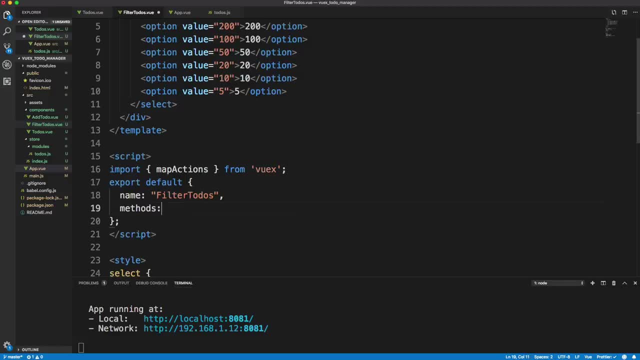 We're going to add methods since it's an action and all we're doing is, is the action. There's no other methods. So I don't have to use the curly braces and spread operator. I'll just simply put in map actions with an array that has, um, filter to dues. Okay. 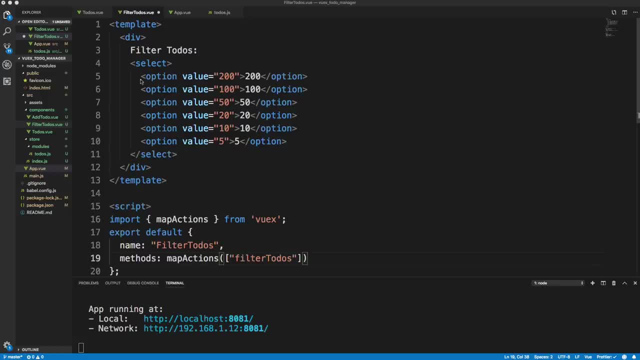 And then all we have to add up here is a change event to select. Okay. 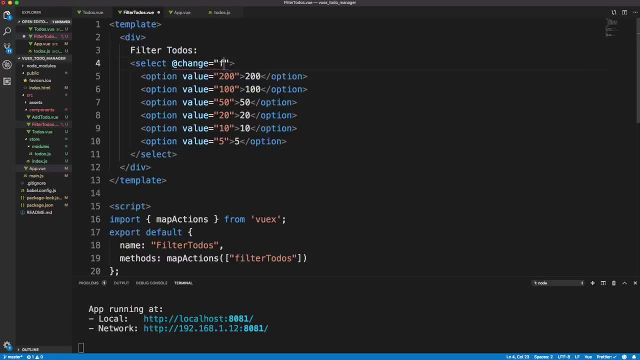 So whenever this is changed, we're going to call the filter to dues action and we're going to pass in dollar sign event that'll pass in the actual event. All right. So let's save that. 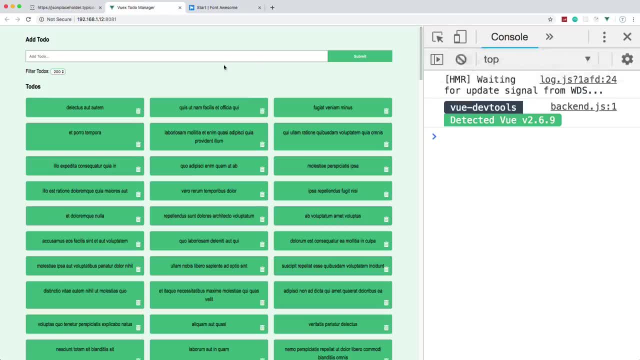 Now, whenever I change that select list, we should see in the console, the event. So let's change it to 50 and there we go. Now. 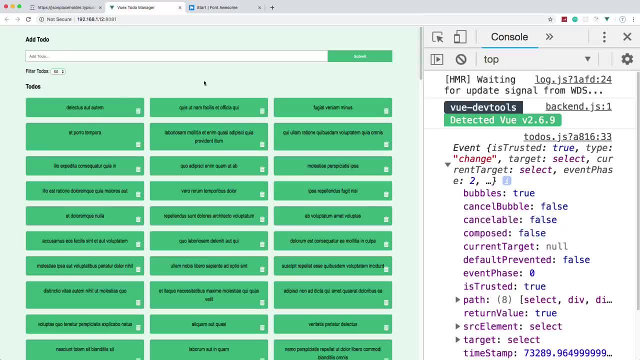 We need to target the inner value of whatever the op. Whatever the selected index. 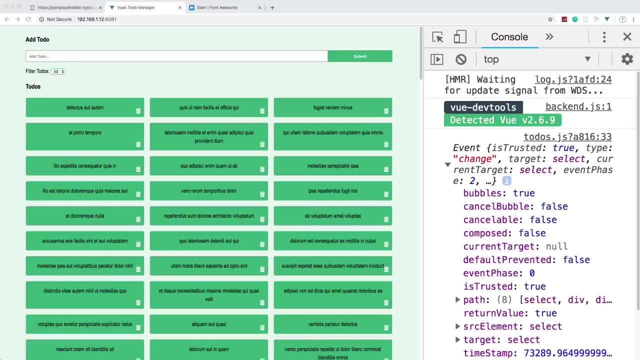 So we're going to use some just vanilla JavaScript here, um, to be able to do that. All right. 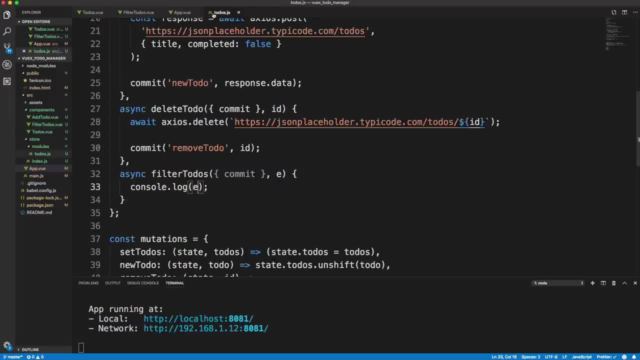 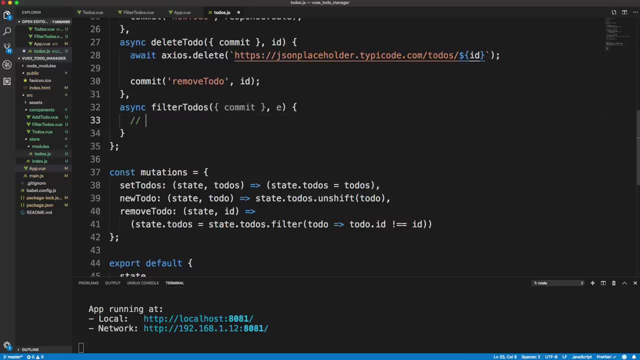 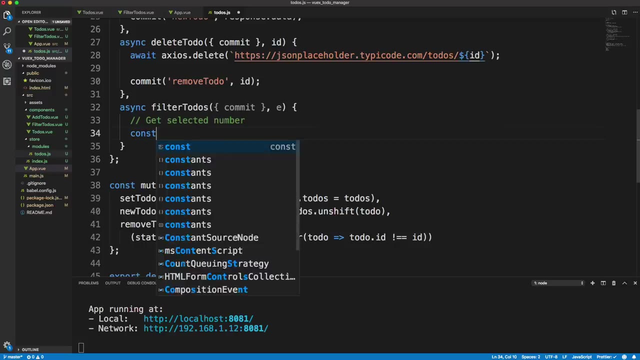 So let's go back to our module and go back to our filter to dues action. So now that we have this event parameter, let's say, uh, I'll just put a comment here. We'll say, get selected number, I'm going to create a variable, we'll call it limit. And we've got with. We want this to be a number. 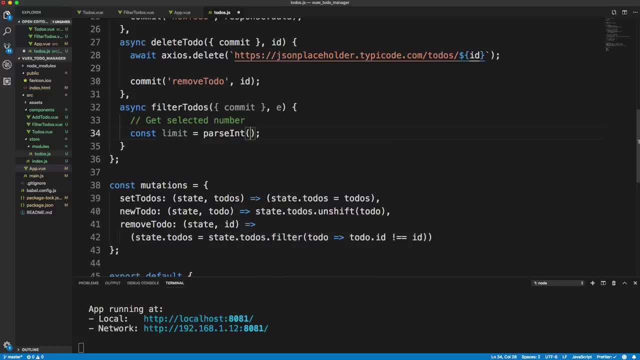 So we're going to run it through parse int okay. And inside parsing, we want to take that event parameter, get the target dot options. 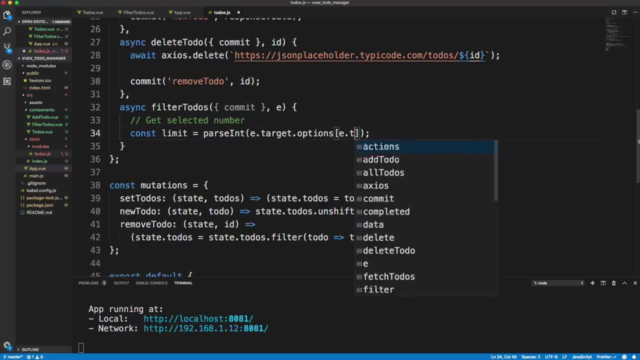 And then as far as the index is going to be E dot target dot options, dot selected index. Okay. 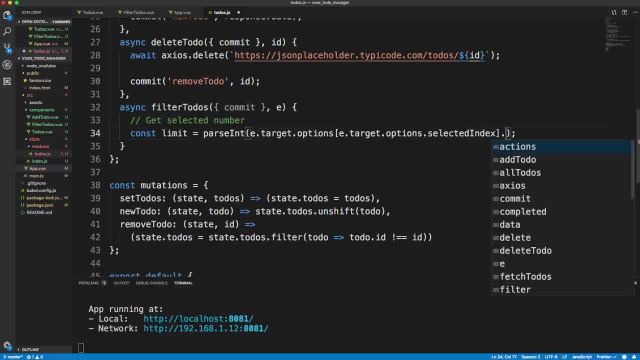 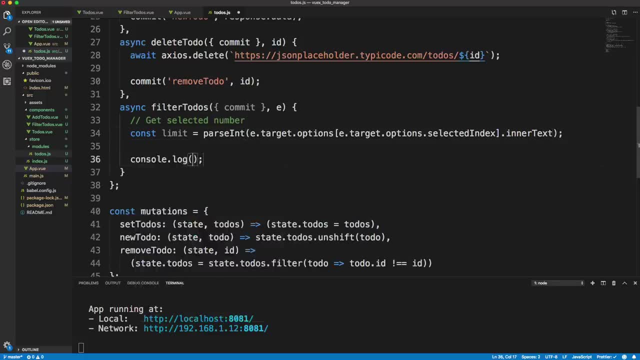 This is just vanilla JavaScript right here and we want the inner text that'll give us the option. But the inner text will give us the action. It's going to be the actual number. So let's just console log now that limit. Okay. So we'll save that. 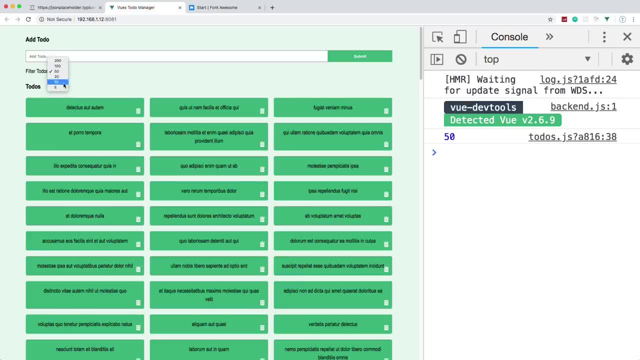 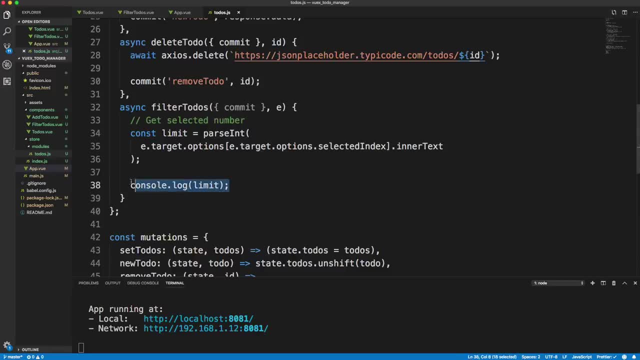 And now if I choose 50, you'll see over in the console, we get 55 and so on. All right. So now that we have that limit variable, let's make our request, which is going to be very similar to our, our fetch to do. 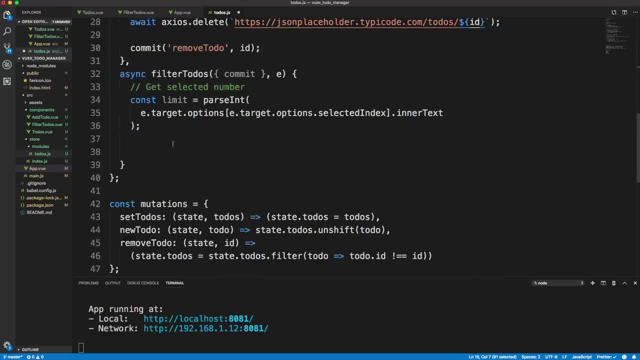 So I'm actually just going to copy this. Okay. So we'll paste that in. 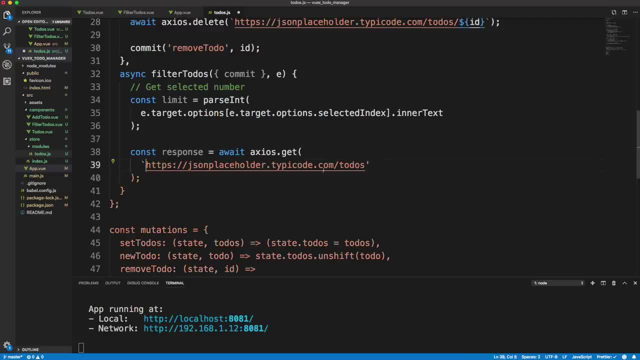 And then I'm simply going to add on, let's change these to a back ticks because I'm going to add on a question mark and underscore limit and set that to whatever that limit is. 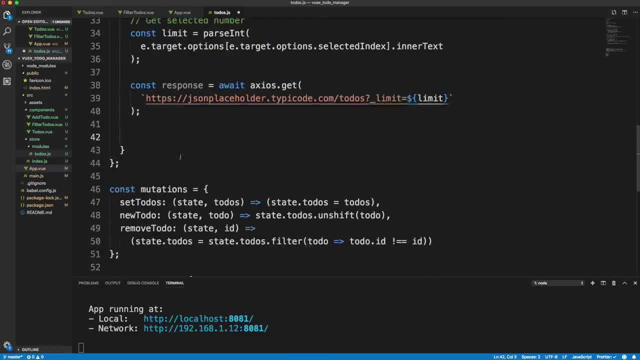 All right. Now once that's done, all we need to do is commit the set to dues mutation. Okay. Because now it's just going to give us the state. However. 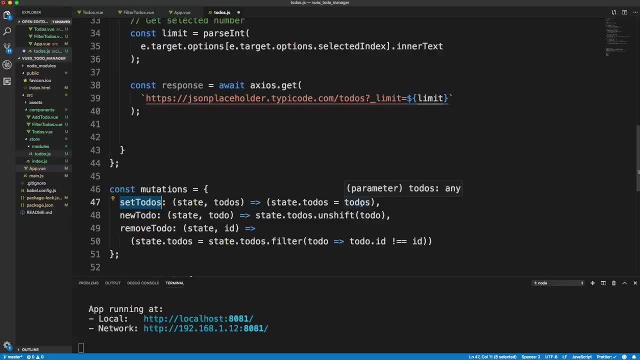 The state is going to have the, the, the limited, um, uh, the limited to dues. Okay. 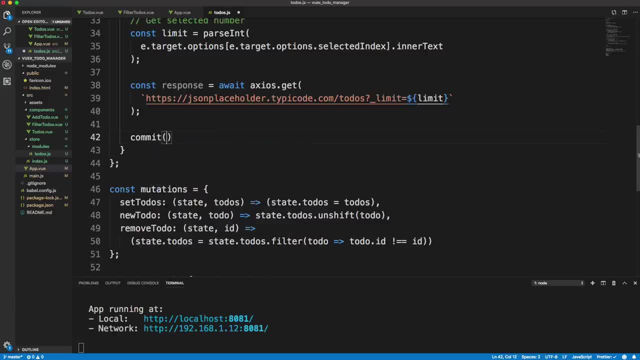 Because we pass in the response data. So let's say commit and set to dues and pass in the response dot data. 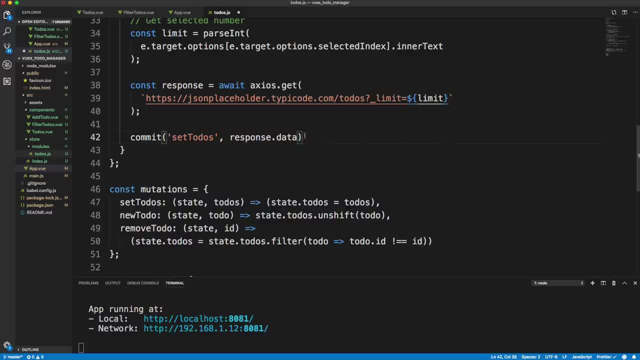 And remember if this is five, this response data will only have five. Okay. 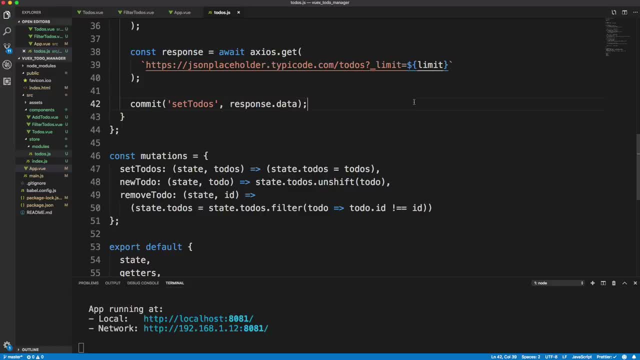 And again, it's just going to return the state, which we're getting with our getter. So let's save that. 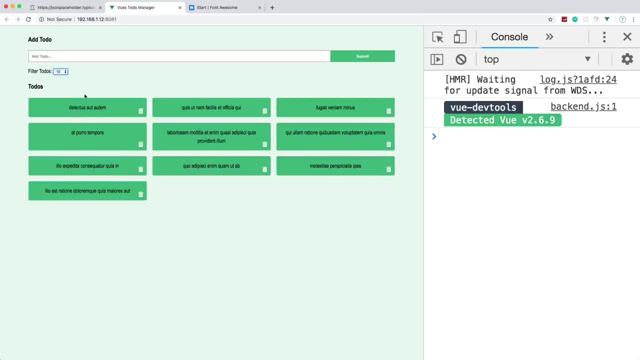 Let's go back. Let's choose 10 shows us 10, five, there we go. 200, 100. Awesome. 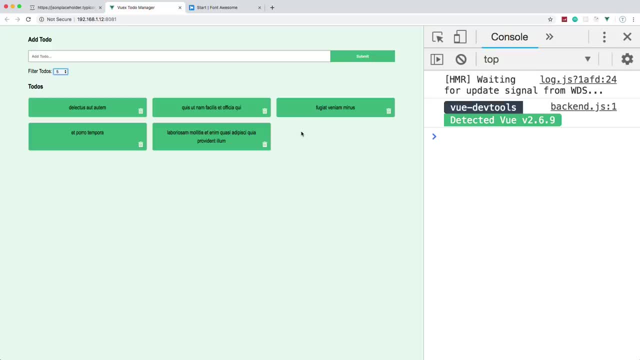 So we can fetch to dues. We can add them. We can delete them. We can filter them. Now let's work on updating them. Okay. 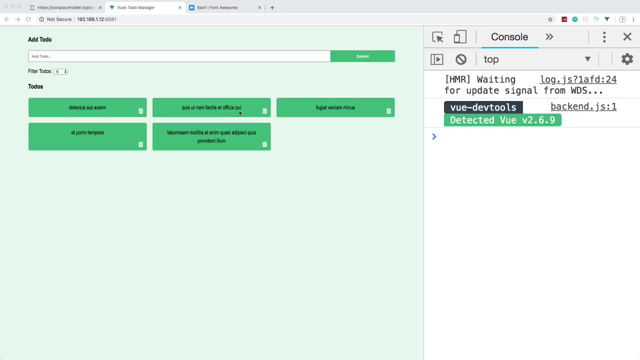 Now I'm not going to do update where like we can update the title. If you guys want to move on and try that, uh, you can do that, but I'm going to update. 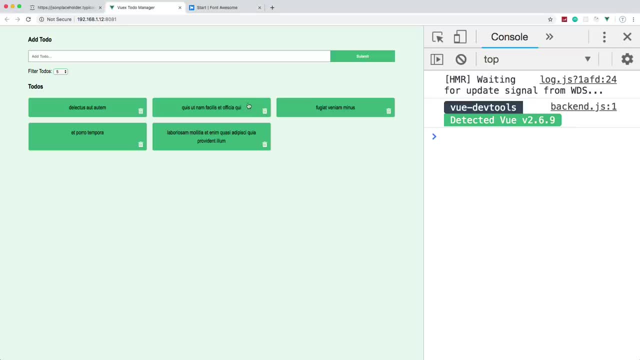 I'm going to update by just double clicking and making it. So it, it makes it either completed or, or incomplete. All right. 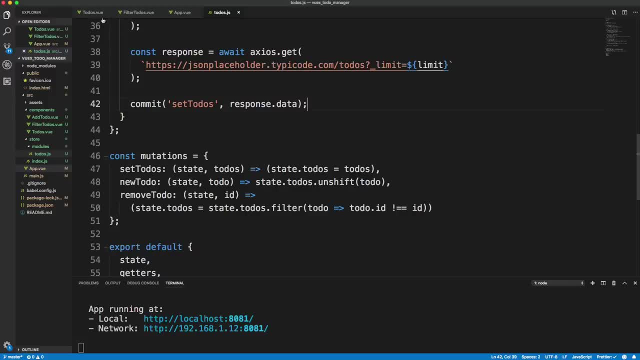 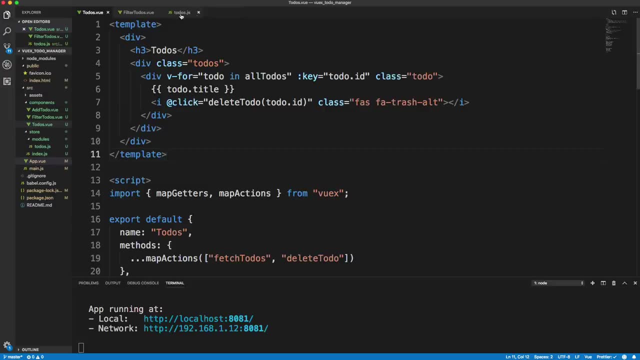 So let's go to our to do's, um, yeah, let's go to our to do's component here. Close that up filter to dues. That's all set. So in our to dues component, I'm going to have like a little legend that shows if it's 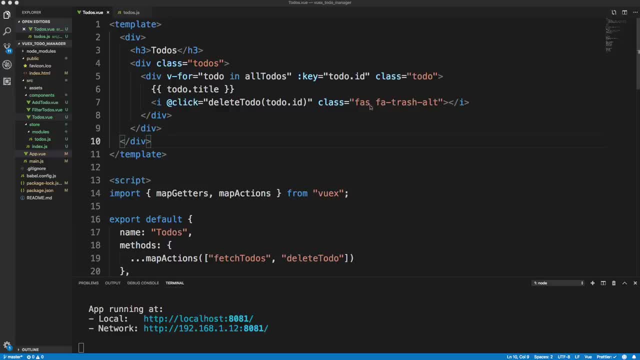 green, it's, it's incomplete. If it's blue, it's not. 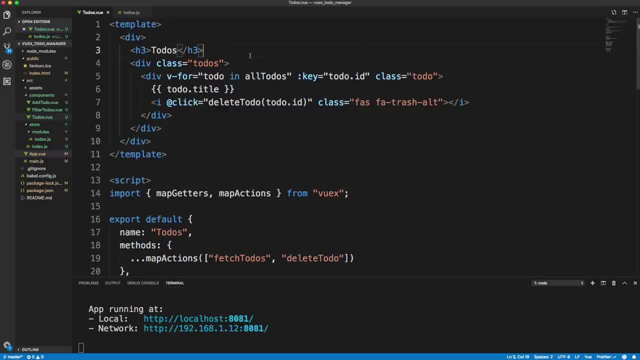 So up in the template here, uh, I'm going to pace this in because it's just, it's just HTML. 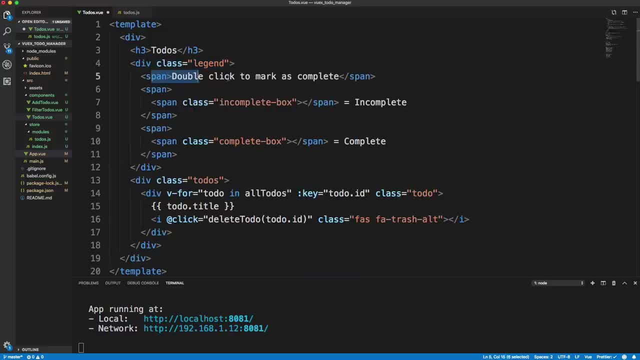 There's no, I don't want to type it all out. So just to dip with the class of legend, we have a span here, a span, two spans here. Um, this incomplete box will be just the color. This will be the other color. So it's just a legend. 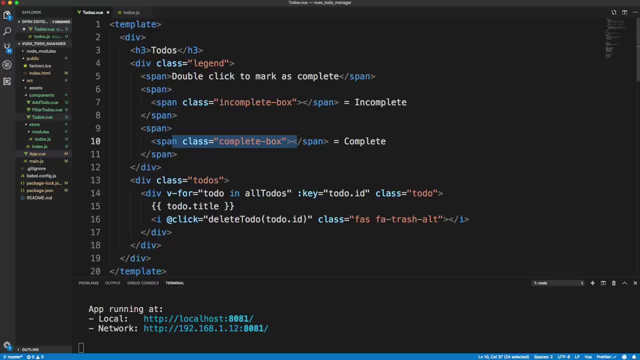 And then I'm just going to put the CSS in. So give me one second. 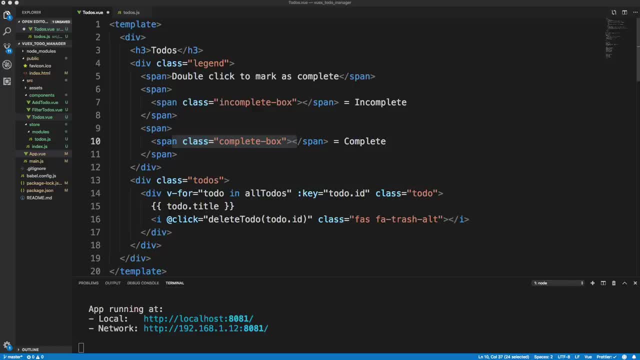 Um. So we have, uh, where is it? Okay. 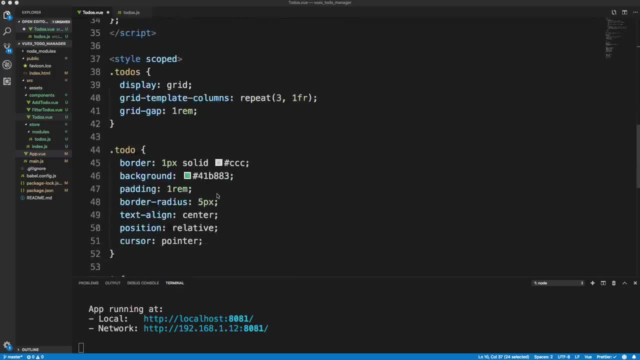 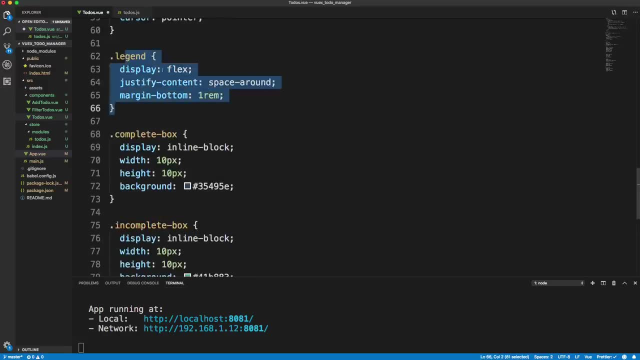 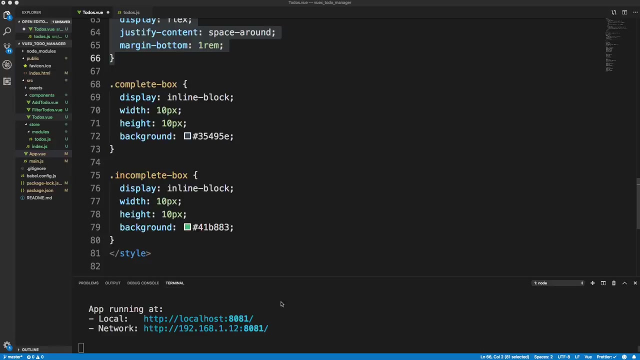 So I'm going to just grab that. I just don't want to type out CSS because that's not what this court, what this is about. So we have legends just going to display flex, the complete box, the incomplete. I'm also going to add a media query to make this the to do's responsive because right now there are three across. But if we have a min width of 500 pixels. 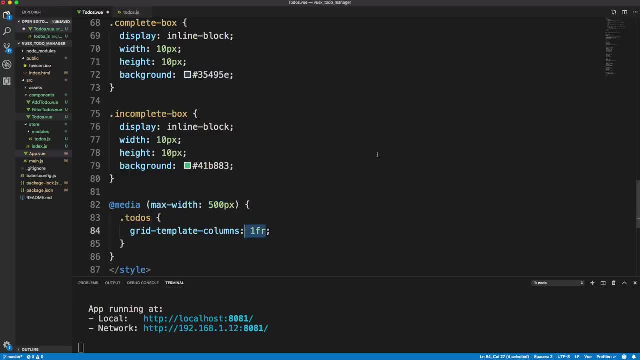 I'm just going to set it to, to be stacked. Okay. 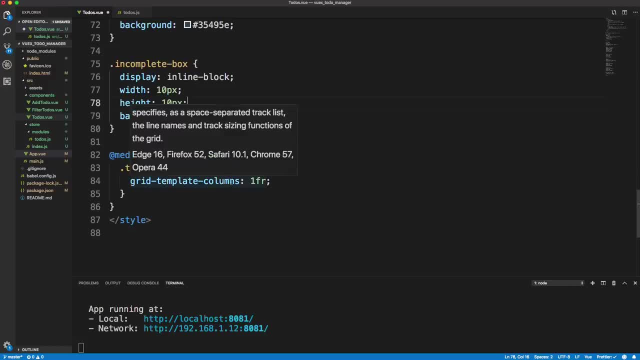 And I, if you're interested in learning about the grid and stuff like that, I just released a course on Udemy called modern, um, modern HTML and CSS from the beginning had to throw that in there. So we'll save that. 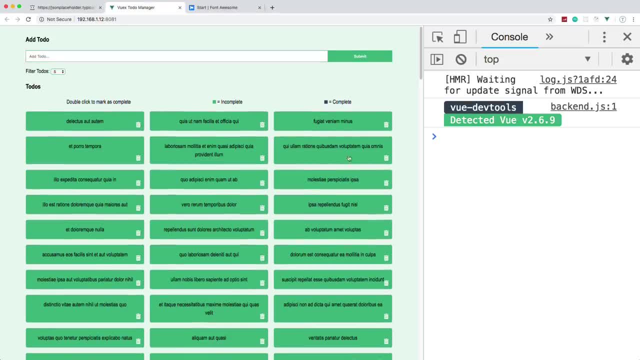 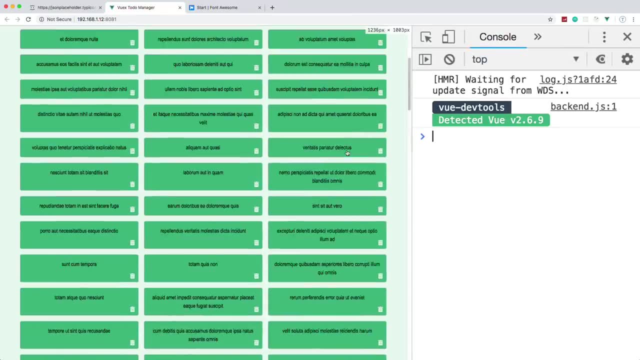 And now if we go back, we have our little key here and it's also responsive. So if we shrink that up, when it gets to 500, it stacks up. Okay. So now. 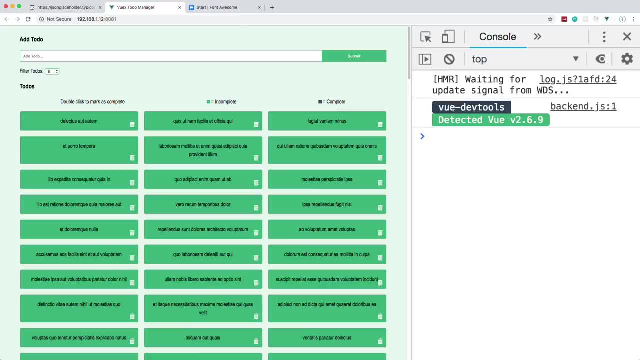 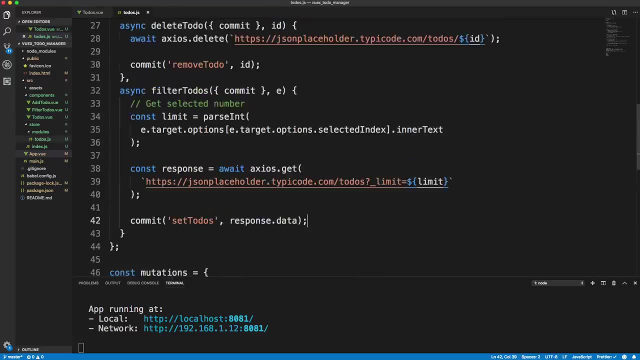 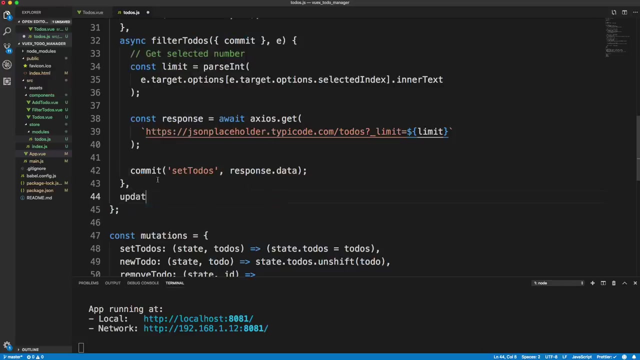 Back to view, let's, um, let's create, let's see, just trying to think of how I want to do this. Um, let's create a new action in our module. All right. Now this action I'm going to call update to do. So let's go under filter, which ends right here and let's say update to do actually a sync. Okay. 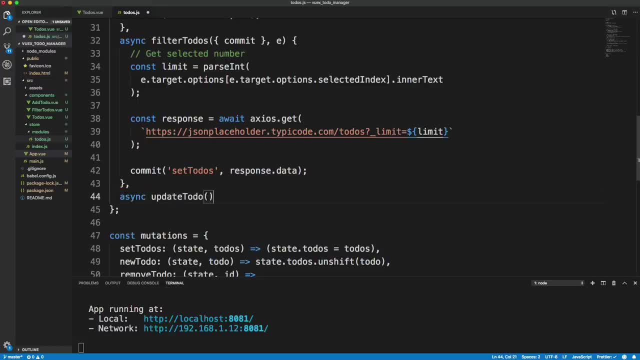 So update to do, and this of course takes in an object and we want commit and it's also going to take in an updated to do. 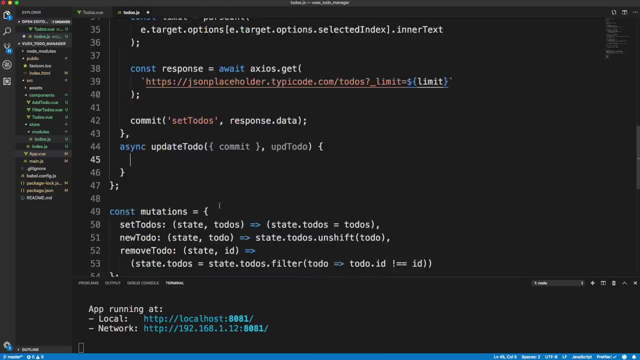 So whatever, whatever we want to update now, this action can be used for any kind of update. We just want to, we're just going to update the, the completed value. But again, I, I, as I said, if you want to update, you can do that. 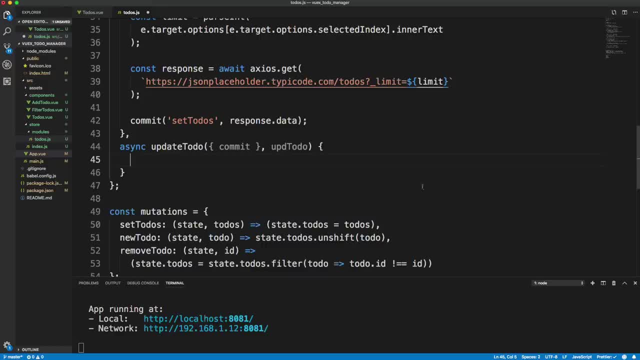 As I said, if you want to make it so you, you can update the text, you can do that as well. 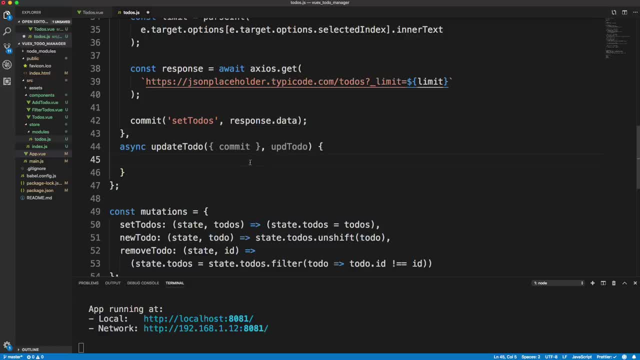 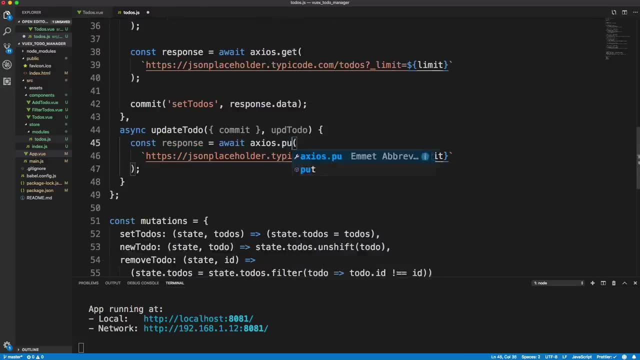 Um, so in this update, let's, um, let's just copy this right here because we're just making a request, putting it into a response, except we're making a put request. 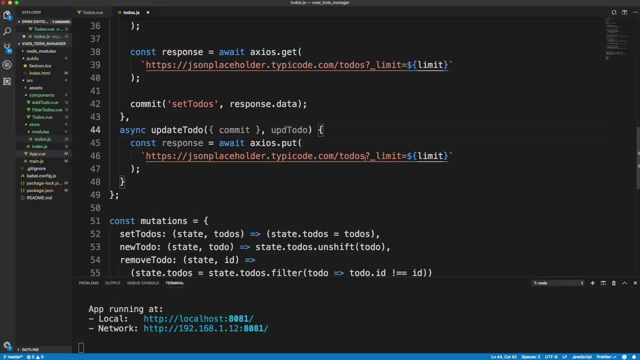 When you update something, you want to use put. So we're going to use this URL, uh, we don't need a limit. So we want to do to dues slash and then whatever the ID. Now this update to do. Object that's passed in UPD to do has an ID on it. So we're going to use that. And then after we get that response, uh, we're going to go ahead and commit updates to do, and let's pass in our update to do like that. All right. Now down here. Okay. 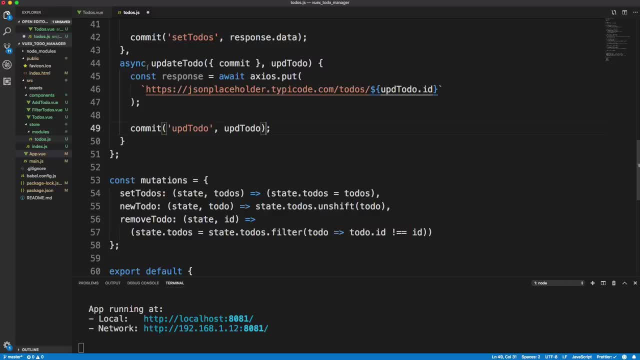 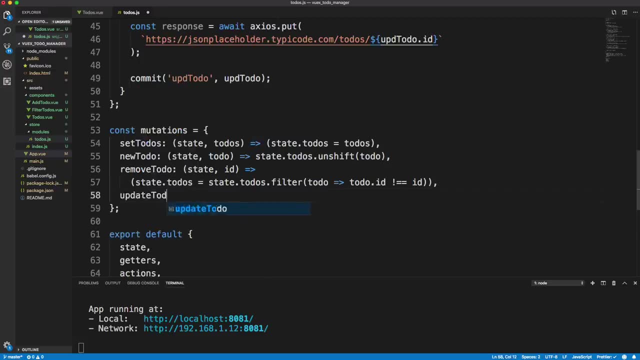 So I don't really like calling the mutation the same as the action, but I guess it's fine. So down here, let's say update to do, okay, so this is going to take in state and it's going to take in the new to do so updated to do, um, and let's see, I'm going to actually open up some curly brackets cause there's a couple of things I need to do here. I w we need it to. Okay. 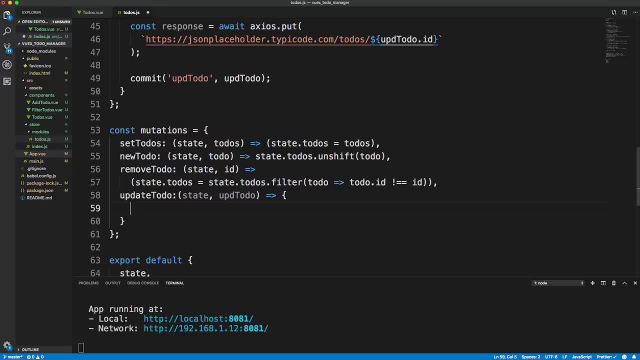 So we want it to be in the same place, right? When we update it, we don't want it to be pushed on to the end or something like that. 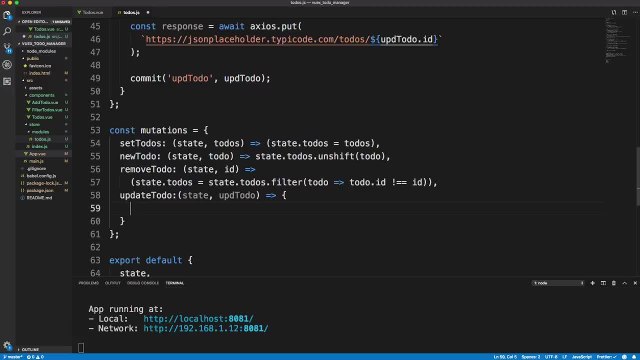 We want it to stay in the same place, which means we need the index of it. So let's do a const index and we're going to get the index of the current to do by using state dot to dues. So grabbing the to dues in the state and we're going to call find index. And for each one, we'll call it to do, and we're going to say where the to do dot ID is equal to the updated to do dot ID. That'll give us the index. Okay. We just want to check real quick to make sure the index exists. 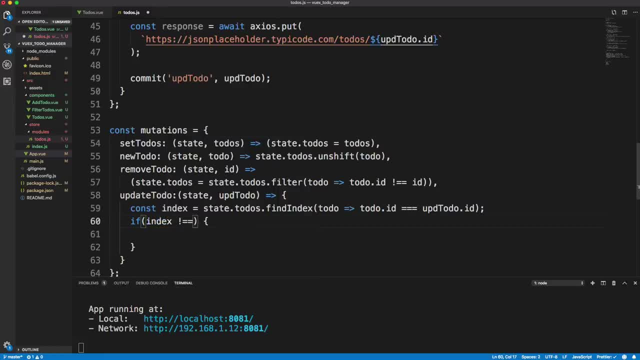 So we want to say if index is not equal to negative one, then now, now we want to do is splice it out and replace it. 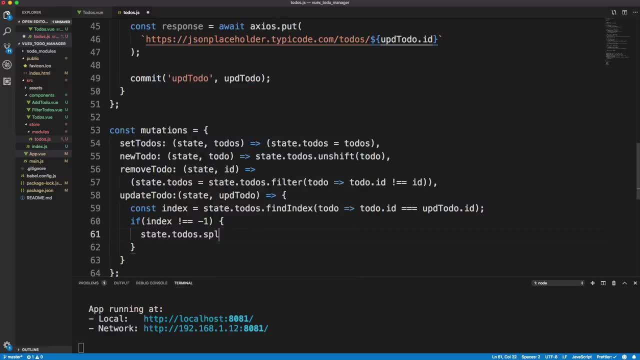 So we're going to say. Dot to dues dot splice, and there's different methods you could use to do this. I'm just choosing to use splice. So we want to pass an index one and then the actual updated to do all right. So that should do it. 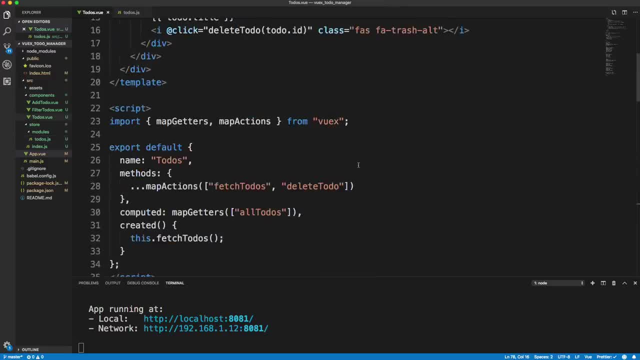 Now we want to go back to our component and we want to bring in a, let's see, we want to bring in the action of update to do. 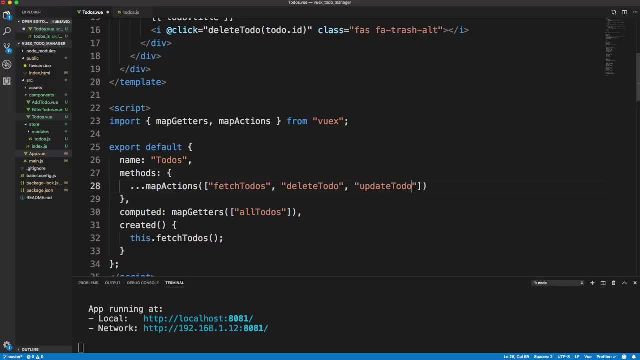 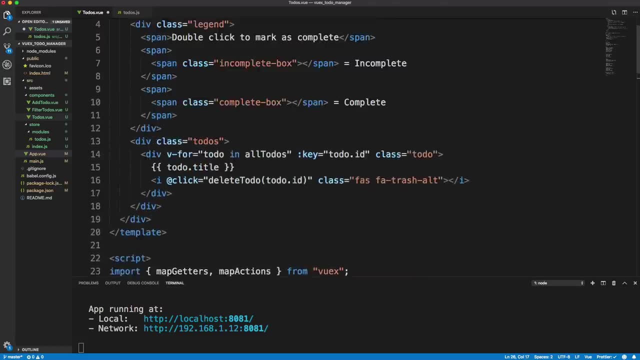 Or map it. And we want this to happen when we double click the entire to do. So let's see, where do I want to put this? We have our class of to dues and then we have each one. So we want to put it on this same, the same one that we have the loop, the V4 on. So I'll do at DBL click equals. Okay. And once we call that, let's call a method called on DBL click. Okay. 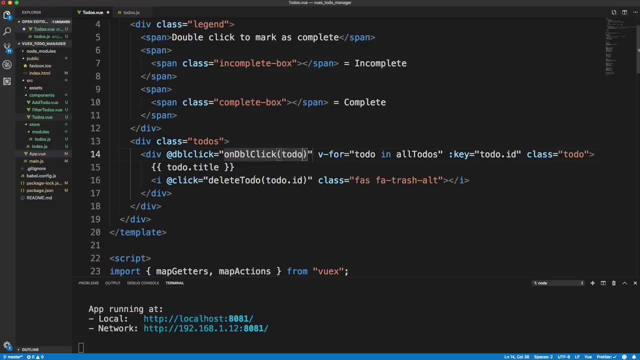 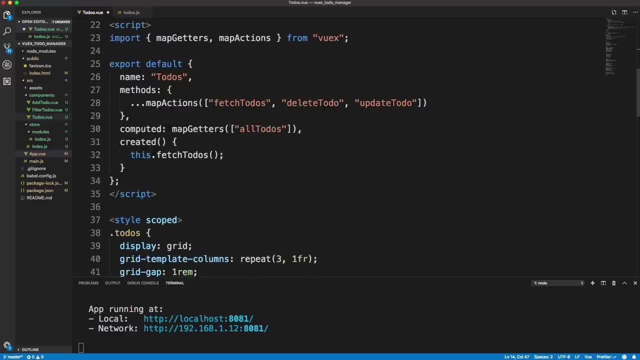 And we want to pass in to do all right. And then we'll go down here and let's create our on double click method. So right here, I'll put a comma, we'll say on a double click. Which takes in. The. The current to do. And I'm going to create a variable called update to do and set it to some new values. Well, actually the only value I want changed is the completed, right? That's all we're updating. 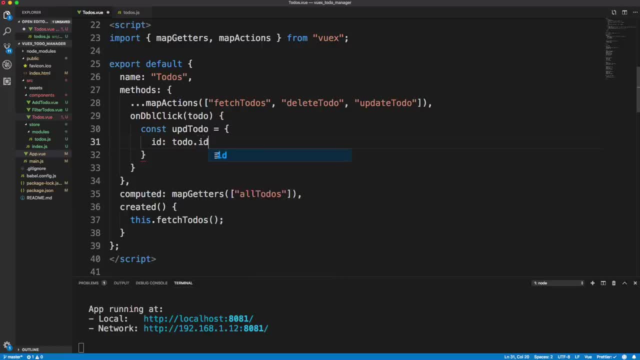 So I'm going to say update, I mean, I'm sorry, ID is going to be equal to to do dot ID. So the same ID title, same title, but this is where you could change it if you want, but. If you want to have the same title, however, completed, I'm going to set that to the opposite of to do dot completed. So if it's true, it'll turn to false. If it's false, it'll turn to true. And then finally, after we create that object, we simply want to call this dot update, which we had IntelliSense for this update to do, and we'll pass in that new object. Okay. All right. 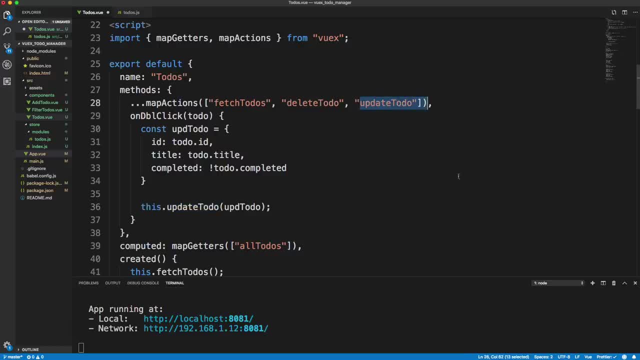 So when I call this dot update to do, it's calling the action that we brought in from our module. And I think that should do it. 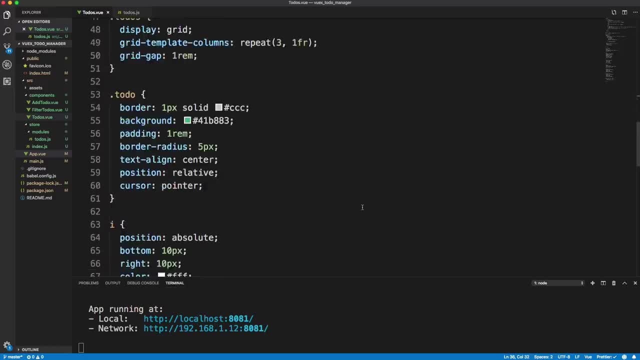 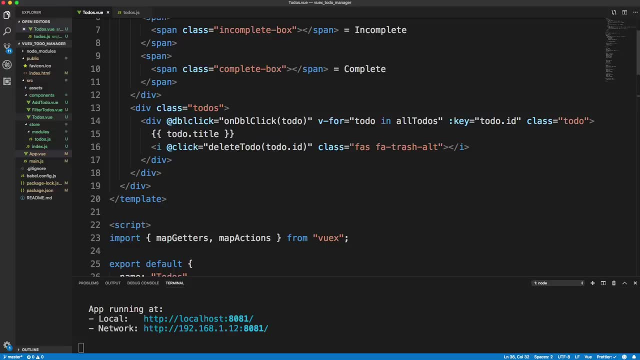 So let's save actually one other thing I forgot is we need to bind a class if if it's false. We want it to be a different color. What I'm saying is the complete. If this is false, we want it to be a different color than if this is true. So. 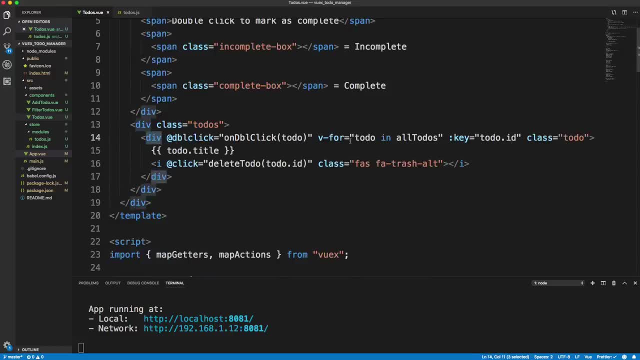 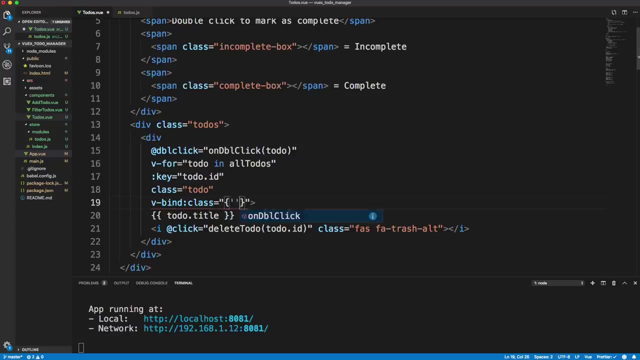 So let's go back up to the to do this div here. This has a lot of stuff on it. I can put these on separate lines, but I think prettier will put it back. Okay, so you can see we have a bunch of attributes here. We want to add one more, which is going to be let's go right out under the class here and let's do V dash bind class. And we want to set this to. We're going to say if is dash complete, well, that's the class name. 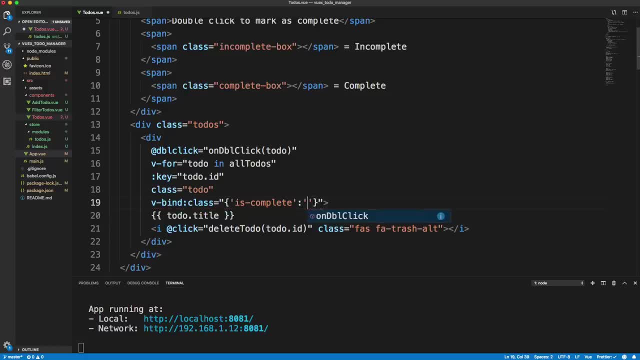 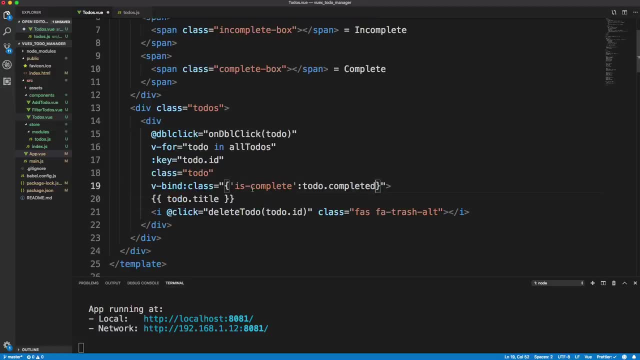 We want to assign this class name if to do dot completed is true. So that's what this will do. 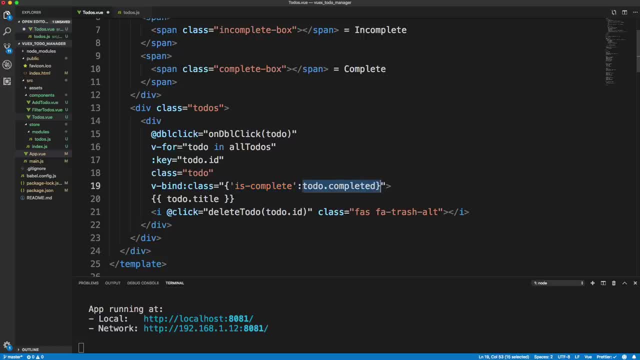 It'll add this class if this value is true. So let's create this is complete CSS class. So down here. Okay. 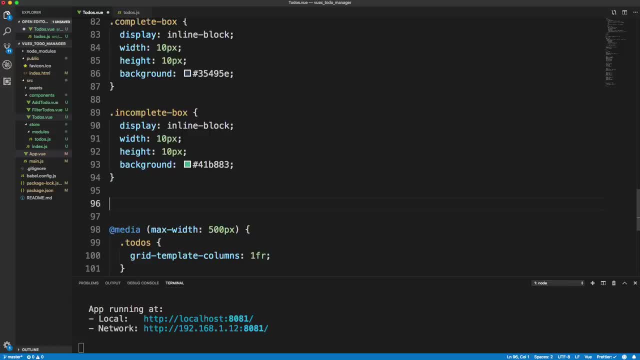 Let me just. Grab it real quick. I forget what it is. 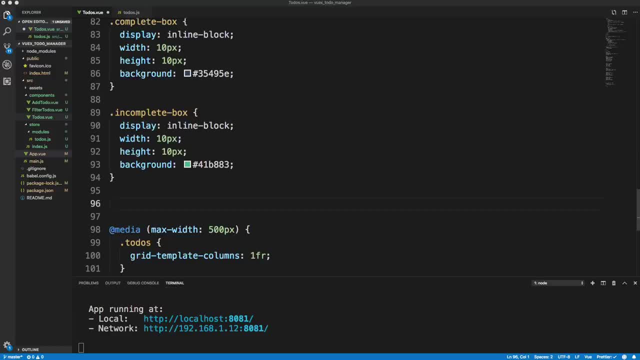 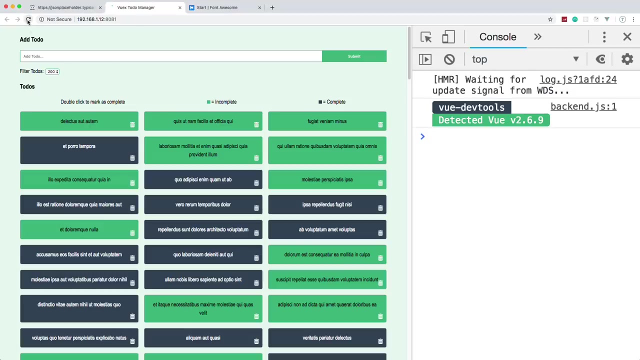 Shoot, where is it? Oh, it's just the background color. Okay, so it's just the blue background or the grayish blue background in a white text. All right, so let's save that and let's go back here and make sure we have no errors or anything. 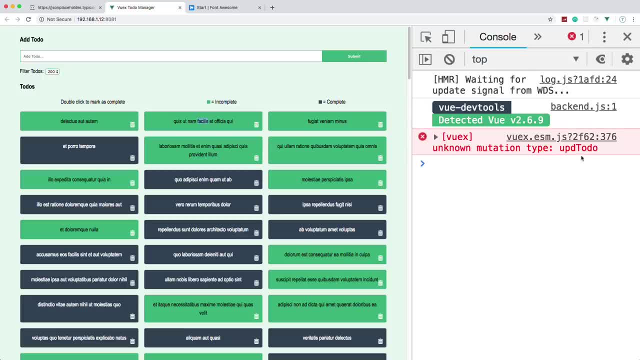 And let's double click. Unknown mutation type. 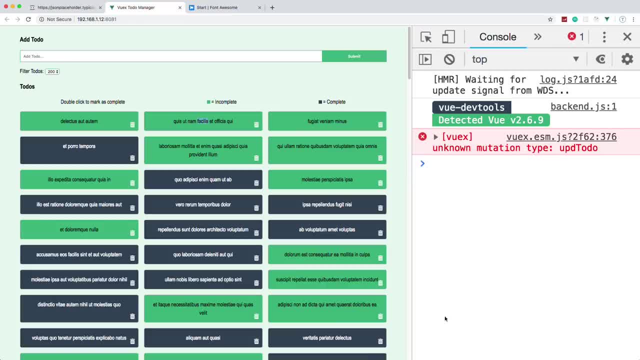 UPD to do. Okay, so let's see. 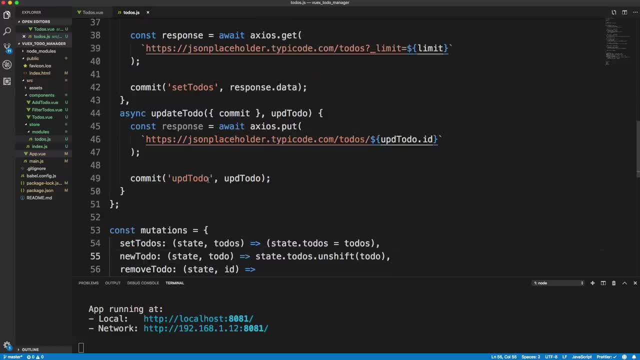 We have an issue here. Oh, I commit. This should be updates to do. And actually when I made this put request, I didn't even pass in the new object. So we have to pass that in as a second parameter. Update to do. And then down here. Okay. Okay. 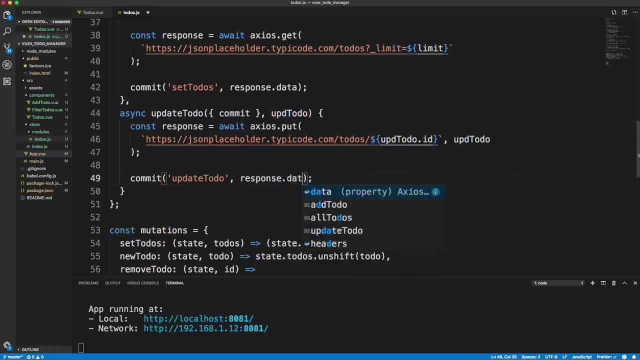 Okay. this we need to pass in our response dot data which will be the updated object all right so 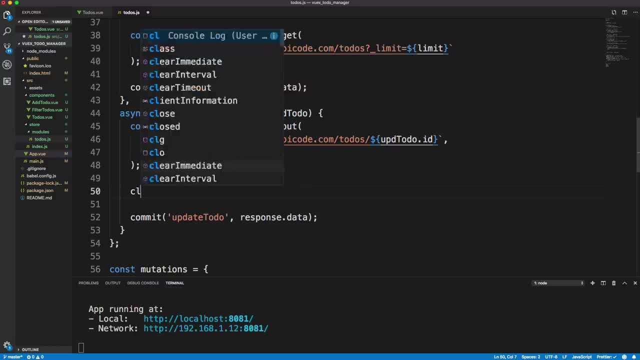 let's try that and let's just console log response data just to verify that it's actually updating 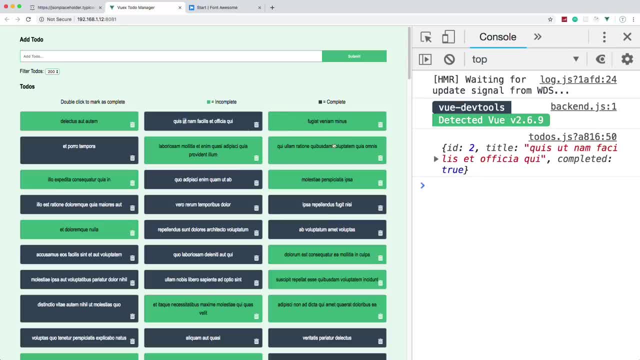 on the server so double click okay so you can see over here completed is true if i double click 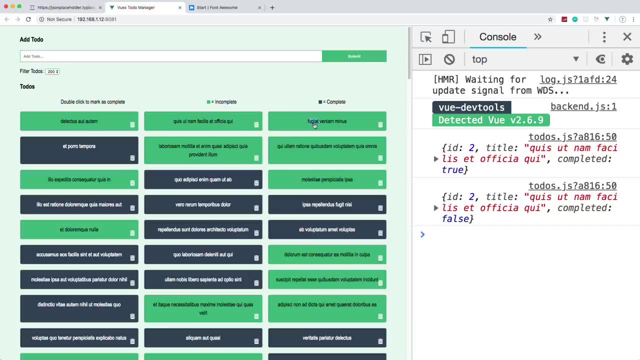 again completed is false good so it's it's making the update on the server with the request we get 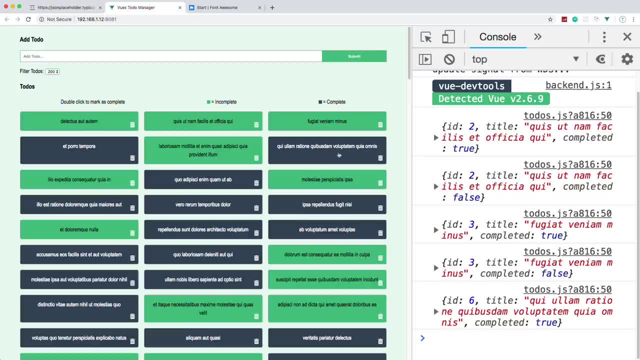 the response back and then we're updating the state which is in turn changing the class all 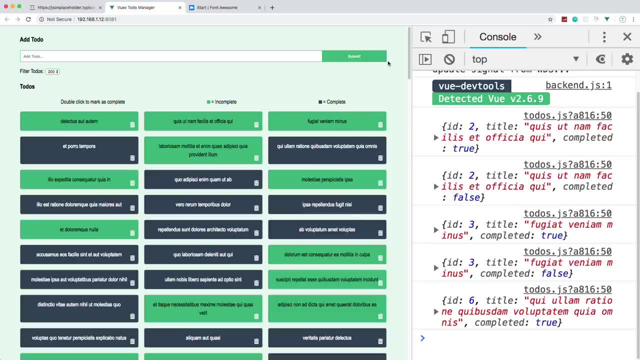 right so that's going to be it guys if you like this please leave a like i also want to mention